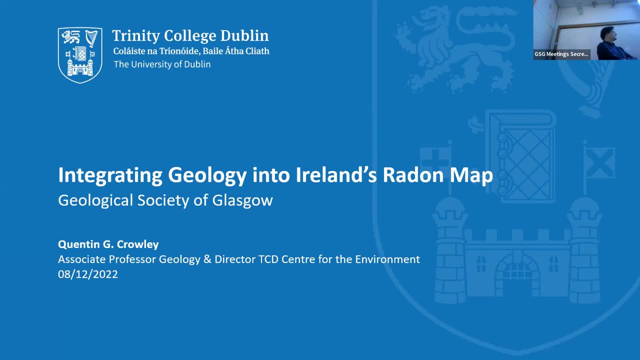 that rocks can do to us, and that's what we got to hear about this evening. so the floor is yours, Brilliant, thank you. thank you so much. it's really, really lovely to be here. I spent- like most people, I suppose- a lot of time at home. I spent two years teaching from my kitchen table. 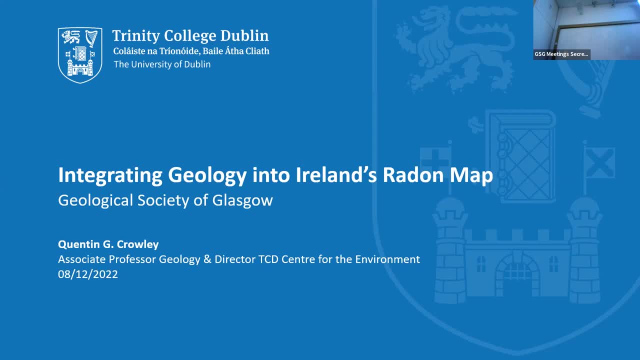 online and to be in front of a live audience. even now, having been teaching face-to-face for a whole year at Trinity College Dublin, it's still. it's really exciting. so I appreciate the invitation and it's really great to be here. Okeydoke so. 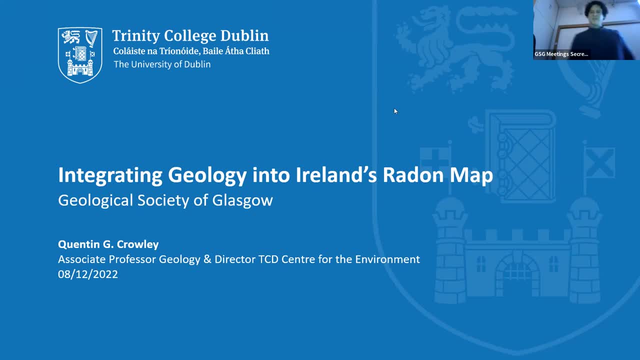 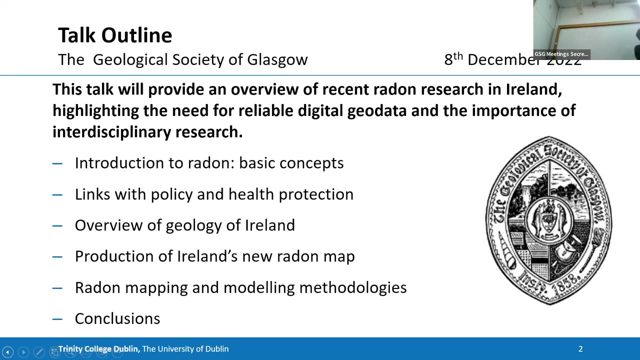 mouse. okay, here we go. so, as a matter of interest, can we get a show of hands? who has heard of radon before? okay, and keep your hands up if you think you know. you know, like a moderate amount, moderate amount about radon, not necessarily an expert, but okay, so that's a good, good indication. 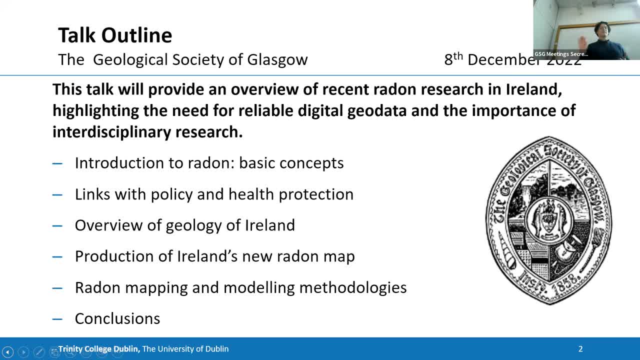 for me. I'm going to run through some of my recent research on radon in Ireland. it is something that's universal. we're in this room, we're breathing air and we're also breathing radon. even if you're outside on a lovely breezy day, there's still radon in outdoor air, so it's. 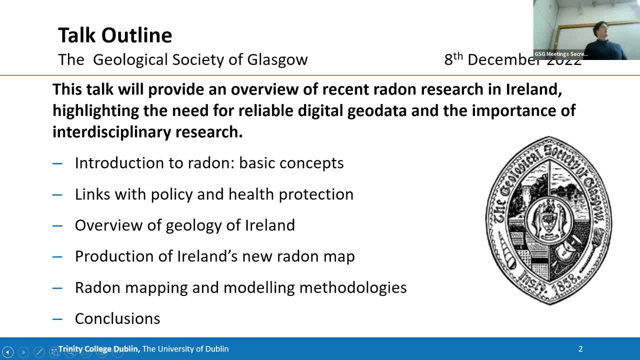 something which we can't avoid. we've always lived with this, humanity has always lived with it, and it can build up in indoor spaces or in closed spaces like mines, and and it is linked to some detrimental health effects. so I think it's worth knowing a thing or two about and it comes from. 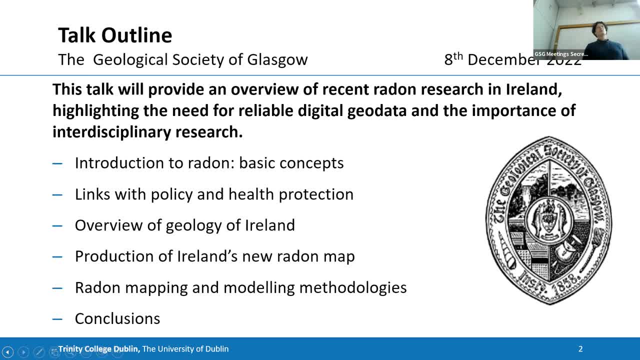 the earth. so knowing, understanding geology, understanding pathways and sources can inform us around. you know radon and where we can expect to find it, so I'm going to go through some basic concepts. it seems like pretty much the whole room knows something about radon, so I won't. 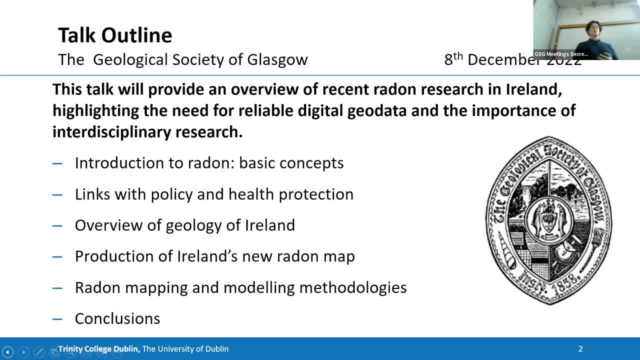 spend too long on that and I'm going to go through some links with policy and health protection. I'm going to give a very brief overview of Ireland's geology of Ireland- I've got one slide on that, so probably 30 seconds- and I'm going to talk through how a new map of radon was produced. 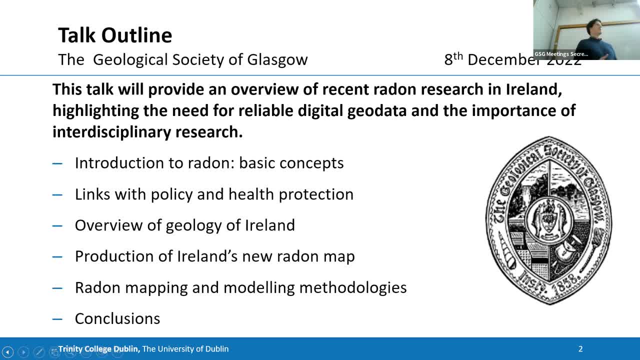 based on incorporating geology and geogenic factors, and talk a little bit about different methodologies and mapping. and, incidentally, a new radon map for the UK was just launched within the last week. I'm not going to be talking about that because I don't know too much about it. 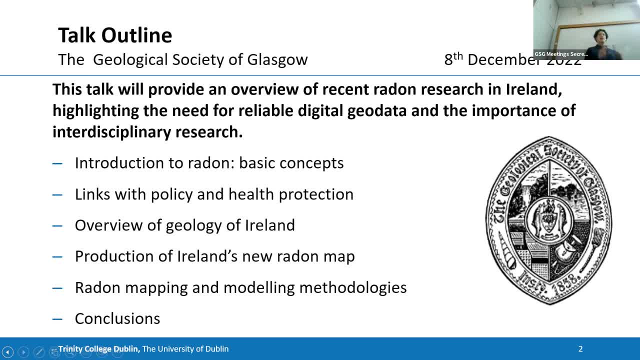 and really I suppose, if I can provide a tagline right at the start of the talk- I think it's important for us to appreciate, to have and appreciate reliable geological data, particularly when it's digitized and particularly when it's open access, so it's available to everybody, because a lot of what I'm going to talk about here I'm using digital. 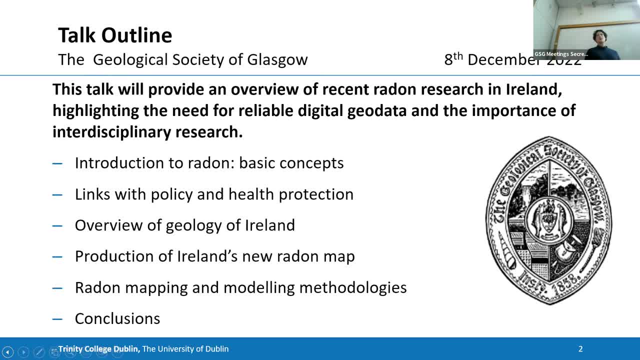 resources- high quality digital resources with geodata- and they weren't designed or captured to do this kind of research. so I'm going to talk a little bit more about that in just a few minutes. and so whoever collected the data and compiled it and archived it, they weren't thinking of radon. 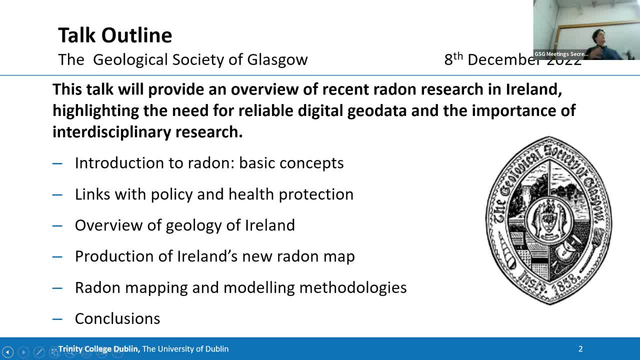 and but people like myself and other researchers, we can come along and we can do fairly novel things with data sets like this, and if they didn't exist, we wouldn't be able to do this research. and okay, and, by the way, you know, it's a very informal setting and if you want to ask a 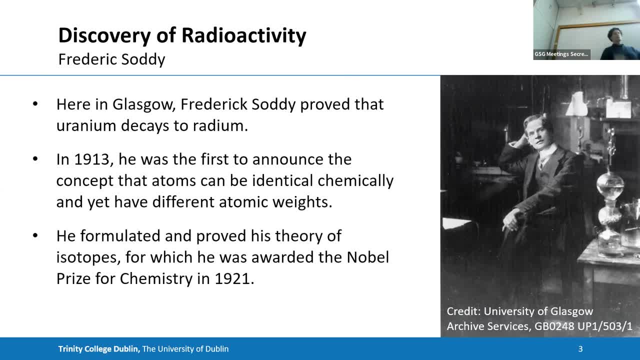 question part way through. that's fine, and if I get a lot of questions, maybe we'll save them to the end. but if there's something you fundamentally don't want to ask, then I'm going to leave it to you. Thank you, If you fundamentally don't understand, feel free to raise your hand. I'd much rather you ask me. 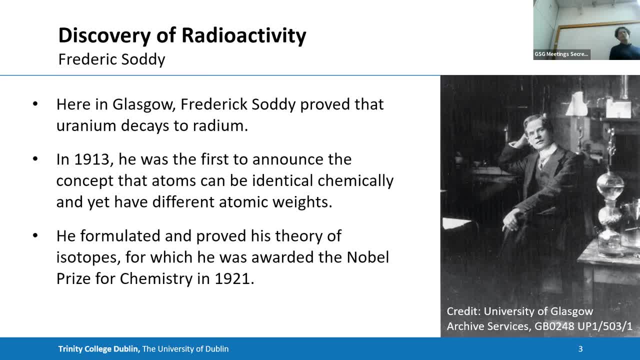 during the talk. then you wait till the end and say what was that thing on slide three? I have no clue what that was, so I couldn't be in Glasgow and not mention Frederick Soddy in terms of the huge, I suppose, that the benefits to physics and chemistry and radioactivity 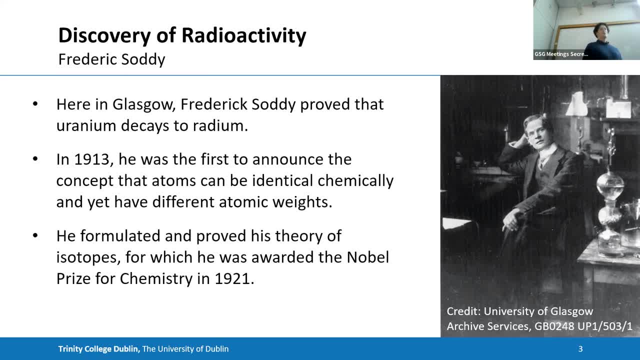 and his research was really fundamental to understanding radioactivity. so he was the researcher who proved that uranium decays to radium and, as you heard at the start, I'm kind of fascinated with radium and it's uranium and its decay products, and so I see this as a 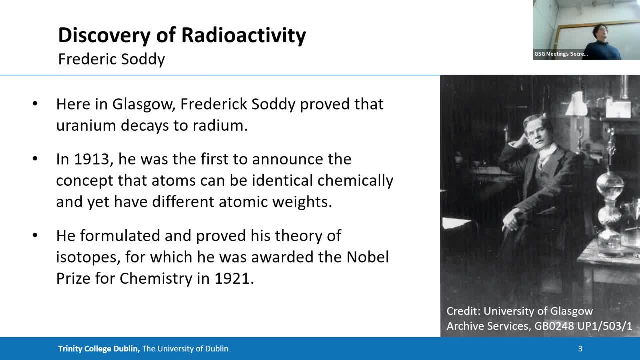 really kind of key milestone in understanding uranium series and its decay and daughter products. 1913 he was the first to announce this concept and which atoms can be. they can seem identical and they can have the same properties and it's the same element, but they can have. 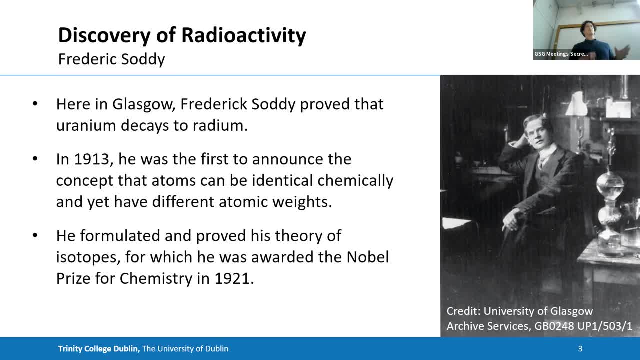 different atomic weights, and this was the whole notion of isotopes. so the same place, the same atoms, but they have different mass. they're different somehow and because of his research and these theories that he developed here in Glasgow and led him to win the Nobel prize for chemistry in 1921. so I couldn't start the lecture and not mention this, because 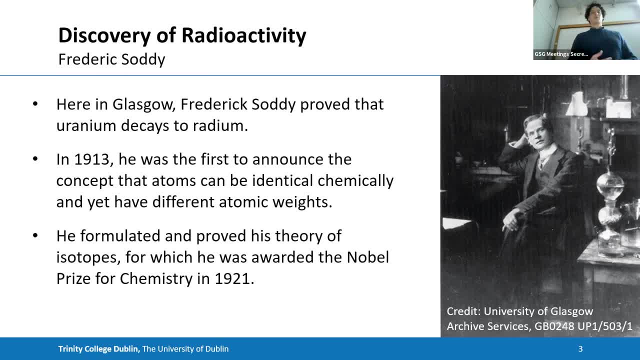 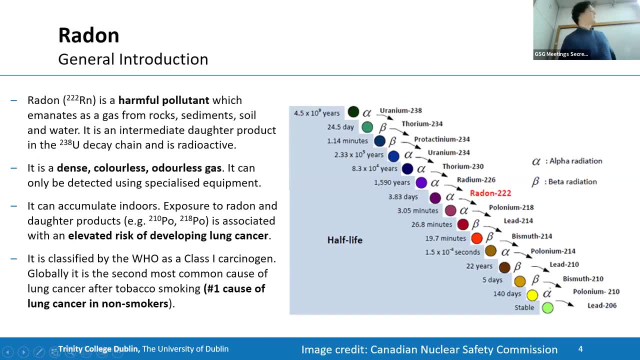 I wouldn't be here talking about radon if it wasn't for his research and back in the early 1900s. So we probably have seen this diagram or something very similar to it. let me just move this little box here top and so let me explain. at the top of a diagram we have uranium 238, so it's a. 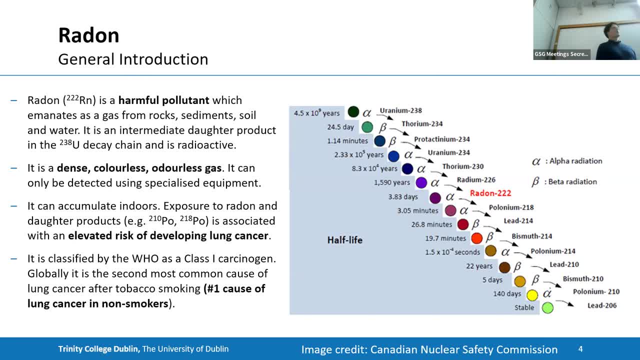 dash 238. so it's the isotope, and there's more than one isotope of uranium. I'm focusing on this one at the moment and you can see there's kind of a cascade, these steps which go all the way down, and at the bottom in green is lead 206. so everything in between is lead 206. 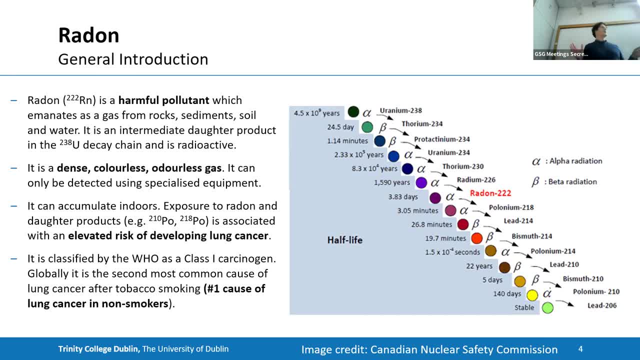 is an intermediate daughter product. so there's uranium in the environment, it's in soil, it's in dust, it's in water, it's all around us, and usually in very small quantities, and it also means that anything in this chain is also all around us okay, so we can't avoid them now in red over here, part. 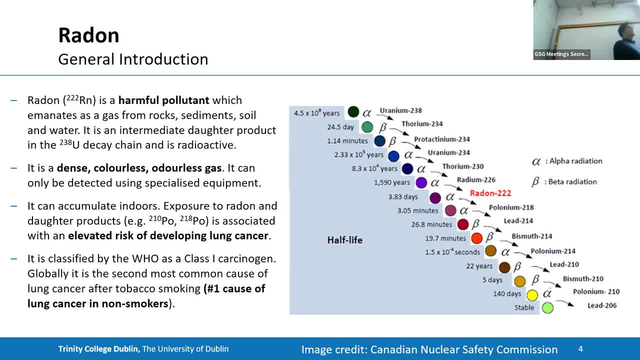 way through is radon. it's radon dash two, two, two. and this is the main um isotope of radon which exists naturally. it's not the only one. I'll mention, uh, one other during the talk. I'll mention one other talk and there's something very curious about radon: it's a gas and everything else in this. 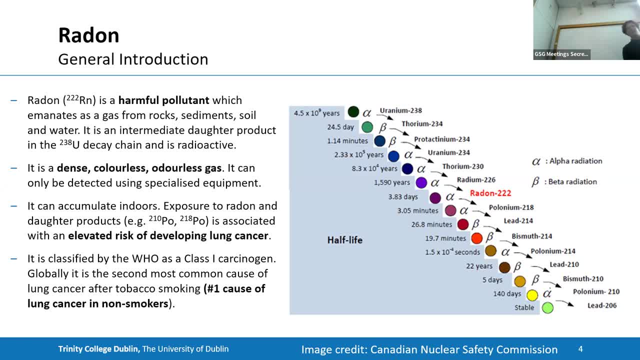 decay chain is a metal, so it's very unusual in that in that respect, and it's actually chemically inert so it's non-reactive, but it is radioactive, so it does. it does give off energy. it has a half life of 3.8 days or thereabouts, so every 3.8 days if there's no new radon coming into a room. 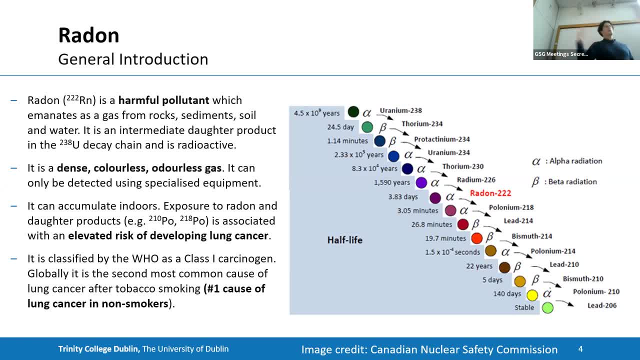 or a chamber. it means that that concentration has been halved and subsequently halved again after another 3.8 days. so it's a very curious thing. um, each step of the way, some radiation is given off. you can think of this as a package of energy. largely it's either alpha 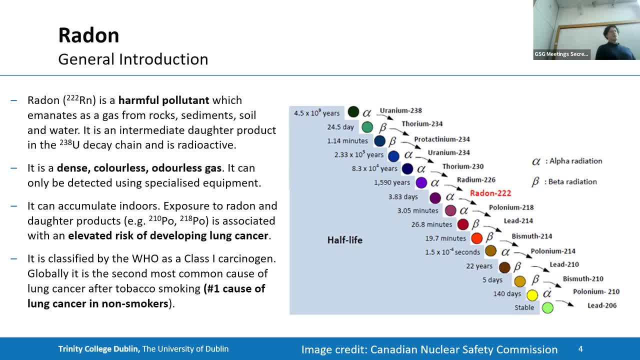 or beta radiation. now, um, alpha radiation can be stopped by your skin cells- dead skin cells, okay. and yet radon is an alpha emitter. and you may think: well, okay, what's the big deal? if our, if our skin can stop alpha radiation, then why? why is this considered something which is hazardous or detrimental to human health? the thing is that 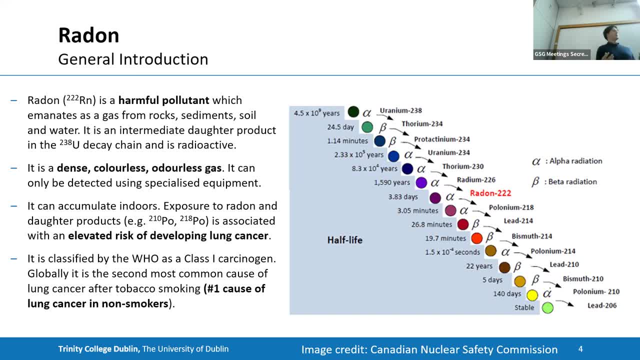 if we somehow inhale or ingest an alpha emitter, then all that energy is absorbed by the tissue and the cells and if we have enough damage accumulating, this can affect our DNA and then this can lead to an increased likelihood of developing cancer. so, because it's a gas and 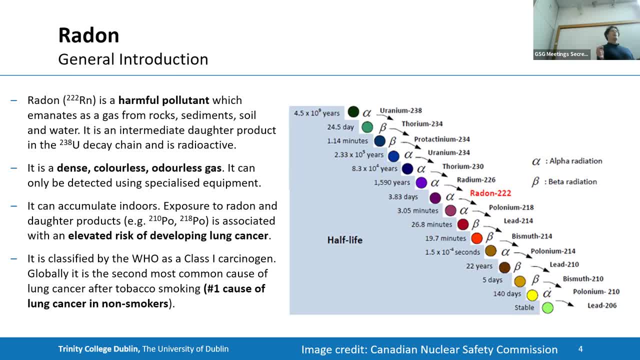 because the daughter products, these- these are charged metal ions and they can stick to particulates and we can inhale the radon or we can inhale the daughter products and this can become lodged in our lung tissue and then this alpha radiation sits there and it irradiates the tissue and this can. 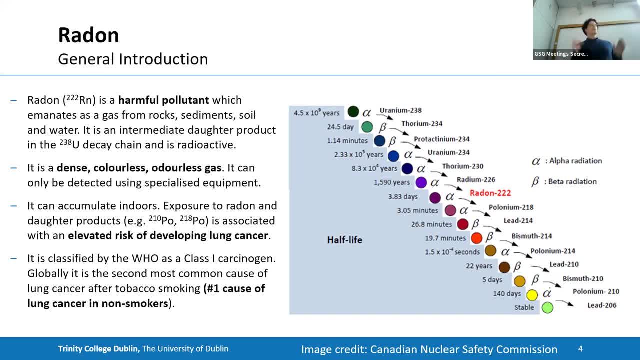 lead to development of lung cancer. so it's not something that's guaranteed. it works in probability um, but definitely there is a link between radon exposure and an increased likelihood of developing lung cancer in life. it's actually classified as a class one carcinogen by the world health organization and globally radon is the second most common cause of lung. 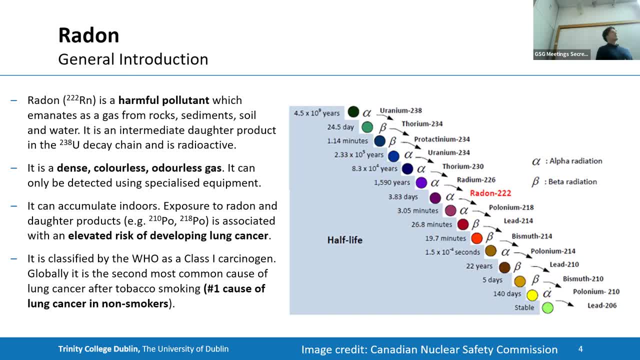 cancer after tobacco smoking and it's the first cause of lung cancer in non-smokers. so it is a pretty big deal and i wonder why more of public haven't heard about this thing. i think it's important to know about. the thing is we can't see it and we can't smell it, and it's very easy. 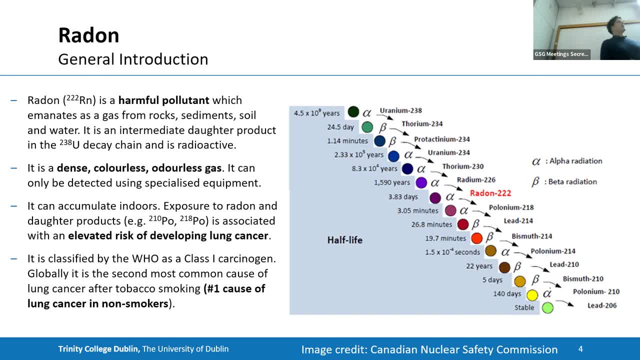 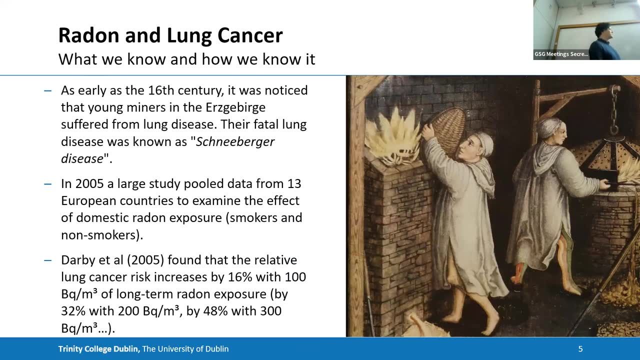 to ignore. it's a dense gas, so if there's a house with several stories, it tends to accumulate most on the ground floor, where a lot of radiation has been emitted, so the soil doesn't really get any, or the basement, but you can find it anywhere. so, um, what do we know about radon and how do we know it? 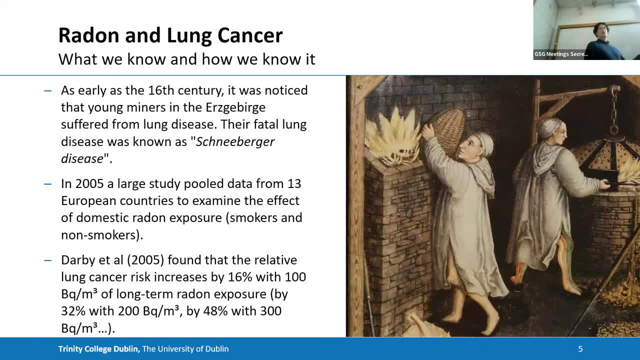 it really goes back a long way, way before the discovery of radioactivity, and there was this causal association that was made as early as the 16th century and in the Erzgebirge mountains where silver was being mined at the time, and there was, it was noticed by physicians that young, healthy 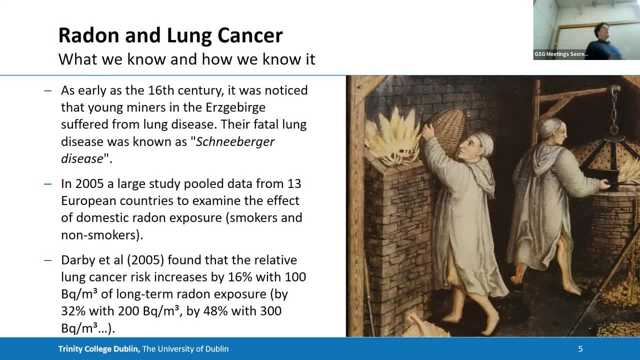 usually men would spend time in the mines and there was a very disproportionate high number of these healthy young men who were developing lung ailments, respiratory ailments and dying now. cancer wasn't known and radioactivity wasn't known, but some physicians made this link. they said there's something going on in the mines, there's something to do with the atmosphere in there. 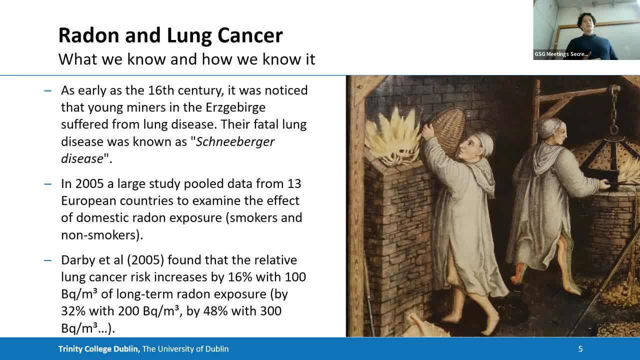 that's causing these young, these young males, to die, and they actually gave it a name, but without really understanding what was causing this and what was this thing. now fast forward to 2005 and a real seminal paper was published which took a large pooled data set from 13 countries around Europe and looking at domestic 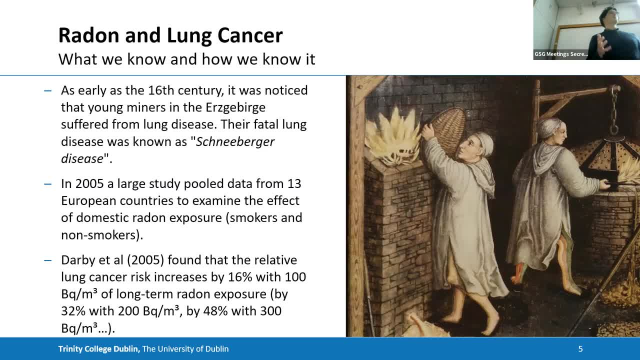 exposure of radon. so up to this point, most of what was known about radon exposure and its effect on human health came from small-scale population studies of miners- okay, people who worked underground, maybe even in uranium mines, some of them as well. so it was really in the early 2000s that this was. 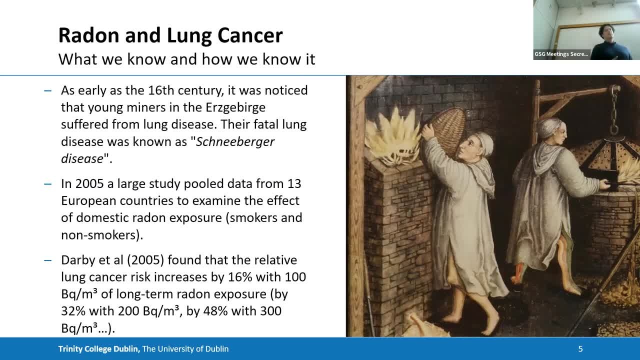 the first. this was a landmark study and it was published by a Darby et al, and one of the main findings from that study was that a relative lung cancer risk it increases by 16 percent. you might be wondering why not like 15 or 20? 16 percent with every 100 becquerels per cubic meter increase, so a 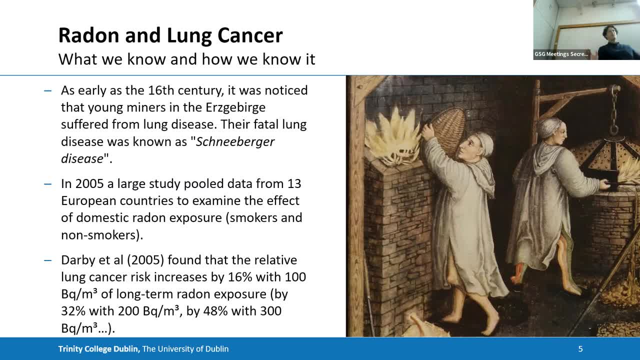 long-term example is if you can picture a cube of air, okay, meter by meter by meter, and one becquerel is one radioactive disintegration in one second. so 100 becquerels is 100 radioactive disintegrations in one second in that cube of air. so for every hundred increase there's a becquerels per cubic. 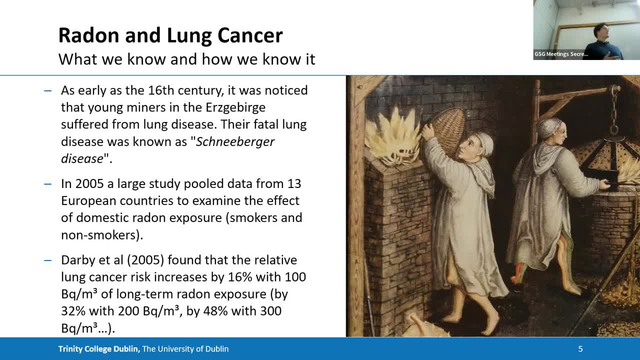 meter increase, there's a 16 percent increase in the likelihood of developing lung cancer over a 30 year period or so, so long-term exposure. so by 32 percent. um with 200 becquerels, 48 with 300 and so on, so forth, and actually um. 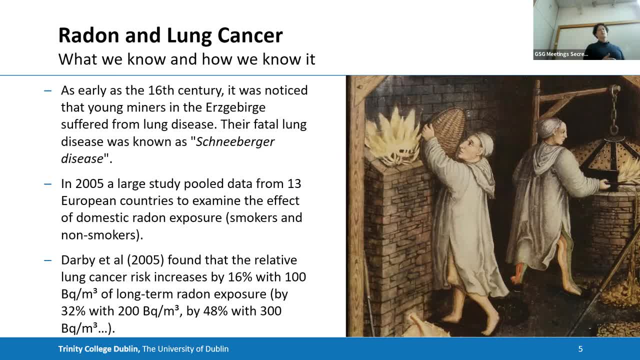 there's a synergistic effect between tobacco smoking and um radon exposure, so it's something which can be proven, not on a case-per-case basis, but in terms of population studies and looking at probabilities. so that's how we know what we know about radon. 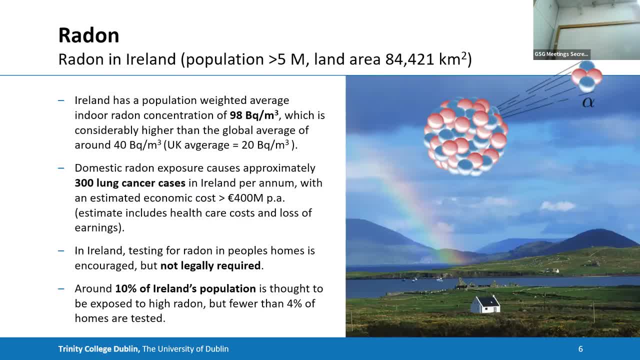 now um. most of the talk i'm going to talk, i'm going to focus on ireland, because it's what i know most about um in relation to radon, but equally, what i'm going to talk about in terms of a methodology or a process could be applied anywhere in the world. okay, so there's a reason why i've 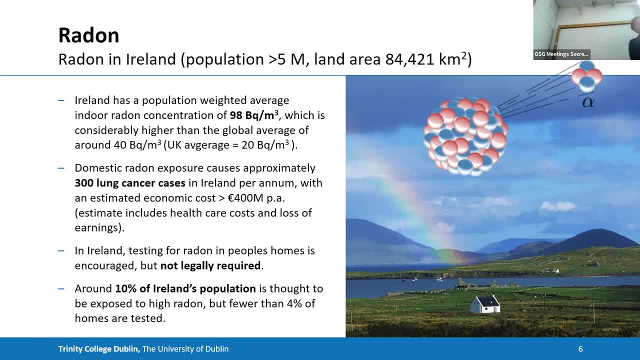 studied ireland, partly it's because where i'm based in trinity college, but also there's a um very high availability, open access to high quality digital geodata. i have tried to do similar kinds of research in some other countries, some of them in europe even, and it's been impossible. it could be. 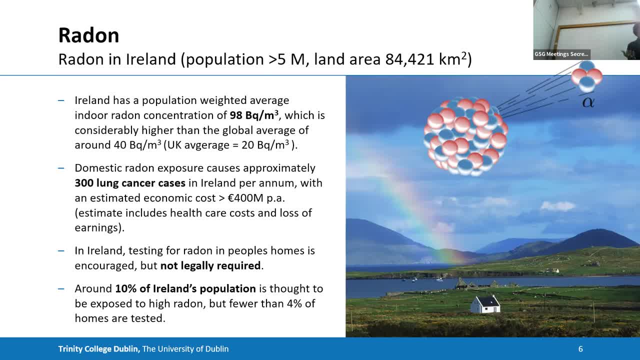 an issue in terms of getting access to the data, or just may not exist in the first place. so, um, by way of an introduction, i suppose another reason why i became interested in radon in ireland is because the average concentration is very high. the indoor average indoor concentration of radon. 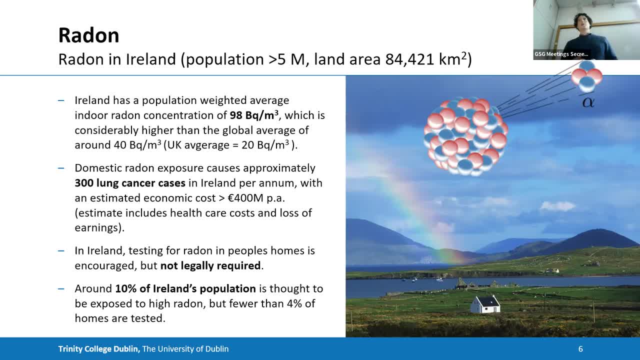 as a population weighted average is just under 100 becquerels per cubic meter. now the global average is around 40 and in the uk it's around 20.. so you'll see, ireland has quite a lot higher than average. and there's a reason for this: it's because of the geology. so as a geologist i became really. 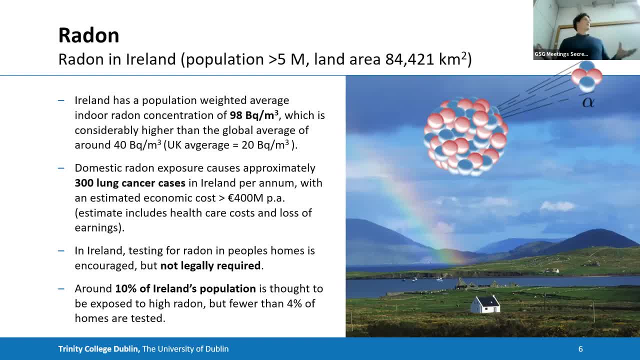 fascinated with this connection between geological heritage of our landscape and the kind of things which are inherently part and parcel with that, whether it's in a positive sense or a negative sense. now again, we can't um absolutely say, you know, if somebody is unfortunate enough to develop lung cancer, we cannot say 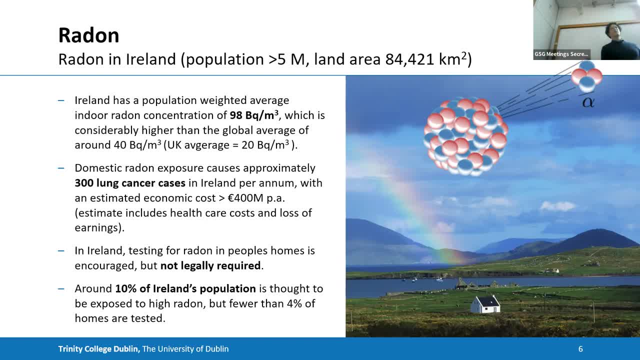 whether this is because of smoking or because of radon exposure or some other kind of, you know, hereditary aspect or a combination of things. but on the basis of probabilistic calculations, it's estimated that around 300 lung cancer cases in ireland every year are due to domestic exposure. 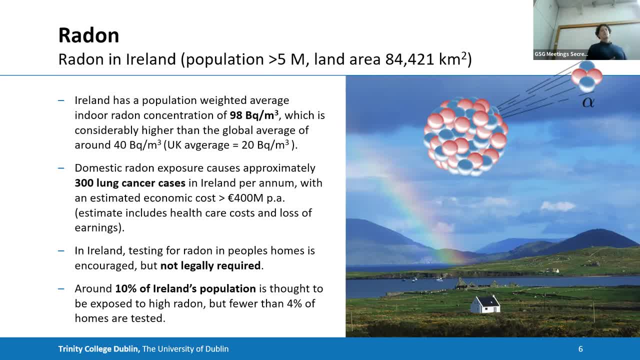 to radon. now it might not sound like a lot, but consider that the population of ireland is only 5 million and the population has just tipped over 5 million for the first time since the 1850s. and i won't say why that is. i think you know um and you know it's relatively 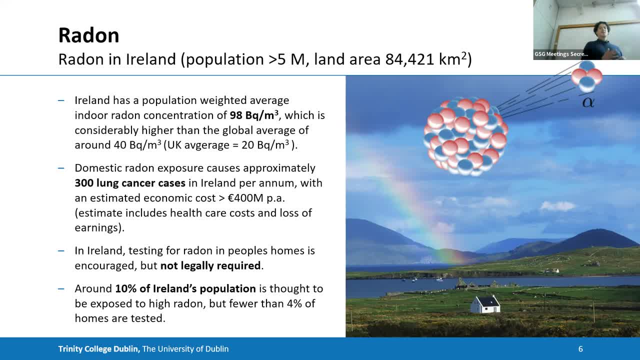 um low population density. so the land surface area is just over 84 000 square kilometers and most people live in cities, so it's a very low population density in rural areas. now, leaving aside the kind of you know, the suffering and everything you know which you can't quite understand, 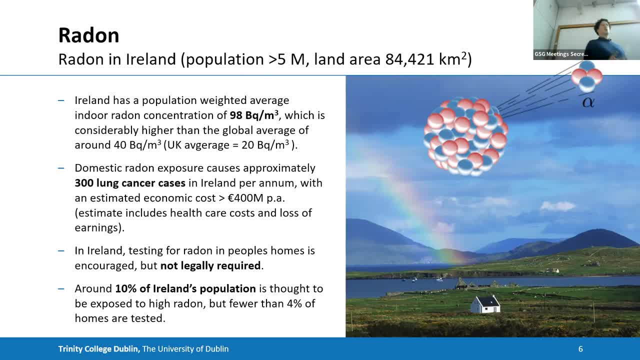 and so i think it's a very good thing to be able to quantify, and in terms of economic cost, that equates to more than 400 million euro per year and which includes health care costs and loss of earnings from premature death, and this is on an annual basis. so it's huge and i think really we. 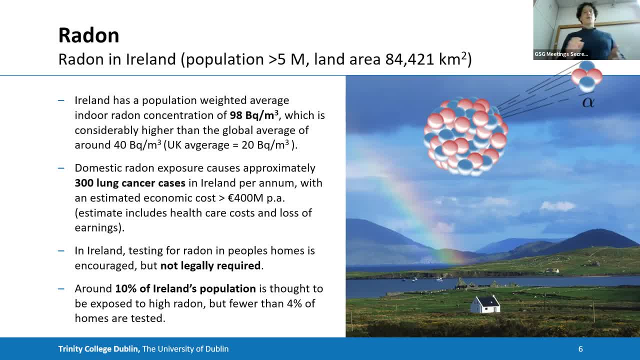 should be paying more attention to radon. for a whole load of reasons. now in ireland, testing for radon- it's not um legally required at all, so you could completely ignore it and not be breaking the law, but you can't do anything about it. you can't do it because you're not allowed to do it, because 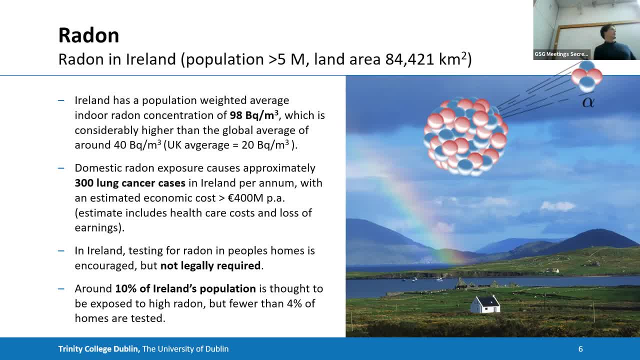 you're not allowed to do it. you could even be a landlord or a landlady and know that there's high rate on in your house or your apartment and you rent it out. you're not obliged to tell the tenants and you're not obliged to test, and so it's encouraged but it's not legally required. 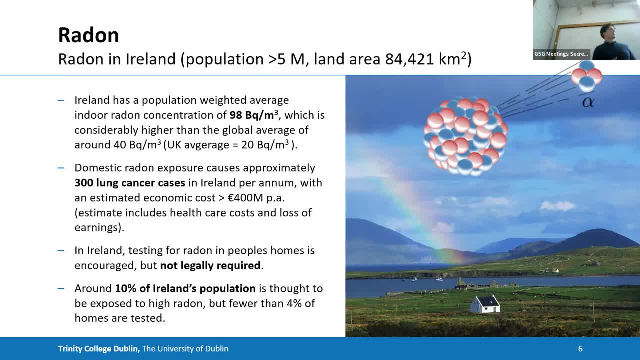 now i've estimated that around 10 of the population of ireland, so around 500 000 people um are living in homes and being exposed to higher rate on a daily basis and they don't know it because fewer than four percent of homes are actually tested and i think that's. that's just 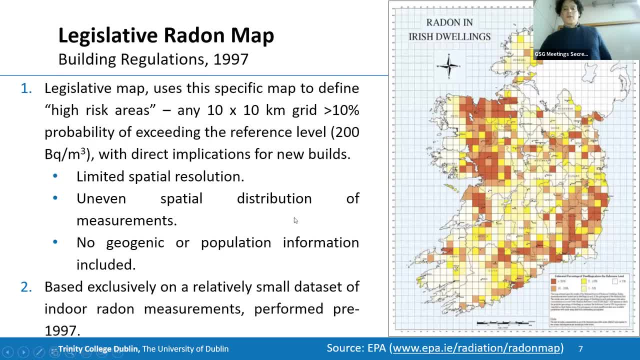 a shame, okay. so yes, the point of the the rainbow is that it's not always a crock of gold at the end of the rainbow, but you could be unlucky enough to house with really high radar. so there's a thing called the epa, the environmental protection agency in ireland, and there used to be a division called. 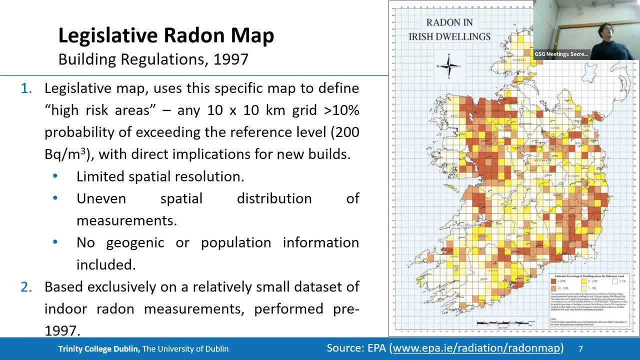 the rpii, which is the radiological protection institute of ireland, and several years ago they became part of the main organization of epa, so that they now work as an environmental part, a radiation protection unit, within the epa. so that's the thing that we're working on right now. 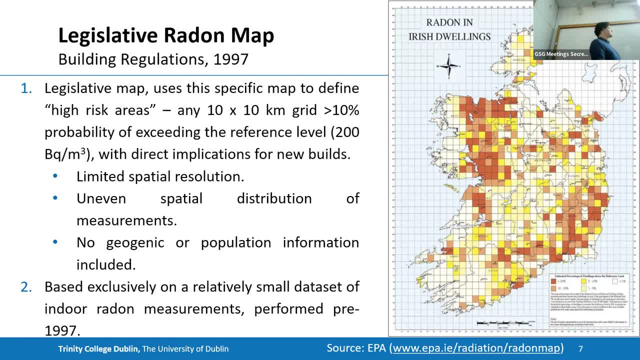 um. this map, which was published as part of the building regulations in 1997, also started me on my journey on radon research. and it's not a map of radon, it's actually kind of a probabilistic map. so there are um squares. each of these are 10 by 10 kilometers and the darker, the shade. 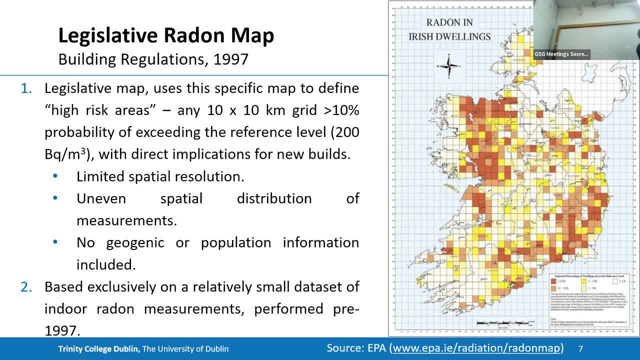 the um estimates, the higher the estimate of the number of homes which will be above a certain level, which is the number of homes that are in the region. and the number of homes that are in the region is a difficult thing to convey to the general public, but essentially it's a probabilistic map. 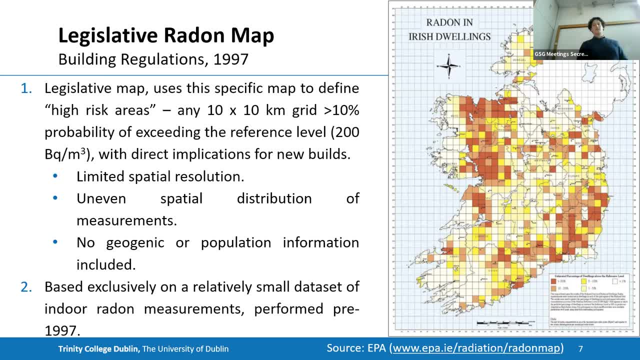 it's looking at probabilities, although it's not really phrased in that way. so any of the very kind of dark, orangey, brown squares mean that this is like a, an elevated um likelihood of a home exceeding a certain level and there's a threshold level. 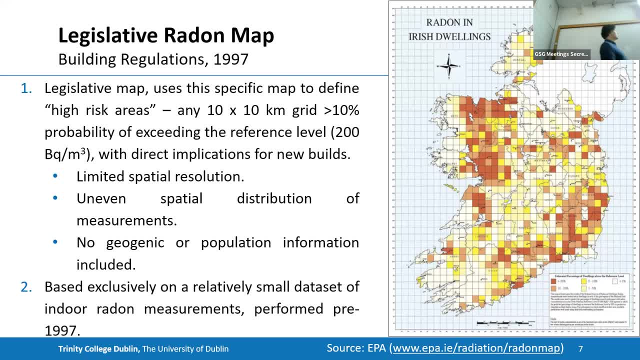 in ireland, which is defined legally at 200 back rails per cubic meter. it doesn't mean that if it's below this it's safe. but it's not because it's not safe. it's because if it's below this it's safe because actually there's no lower level below which there's zero risk for radon exposure. 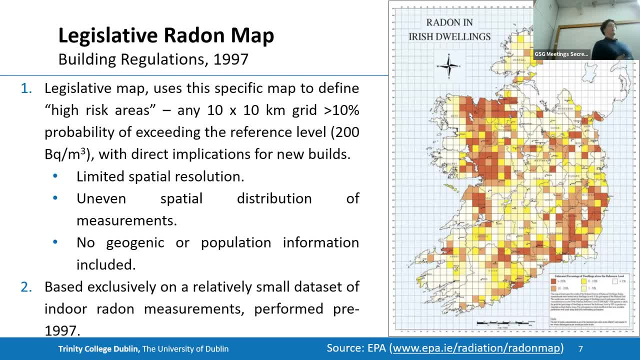 even if it's just one back rail, there's still a risk. okay, it just means it's practical level set by the epa and the relevant government department to say: well, if it's higher than this, you should do something about it to lower it, because you're exposing yourself to an excess risk. 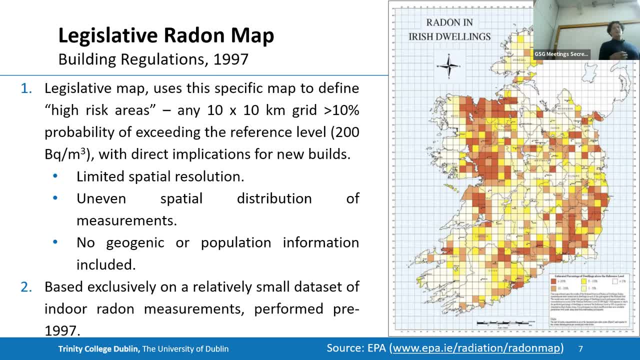 um, now a few things about this map. being a geologist, the first thing that's struck me is there's no geology incorporated in this. the map is compiled from indoor radon measurements, and actually quite a limited number of indoor radon measurements. it's spatially. 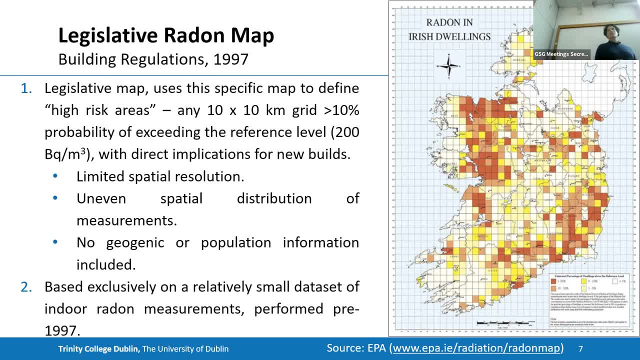 resolved into grids and there's an uneven spatial distribution of data points. so if you're a geologist and you're out sampling and you're thinking, if i have all my data points in one field and none in the other, how could i possibly say something about the other field? okay, so 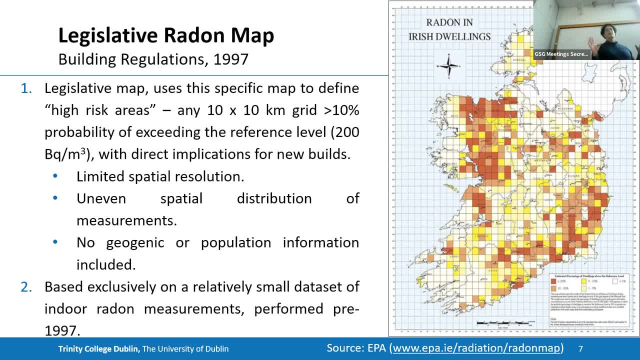 there's a, there's an element or there's an aspect of that in the map, in that a lot of the dates are going to be in cities, because that's where most people live and where there's lower population density. there could be few or no measurements, so there's 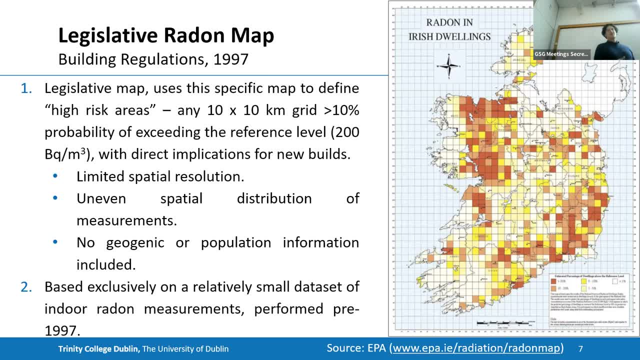 a lot of extrapolation and, i suppose, kind of statistical guesswork, for want of a better phrase, but up until very recently, up until this year, this has been the go-to map, so the inference being that if you build a new home in an area with a dark shade, you have to put in protect measures which 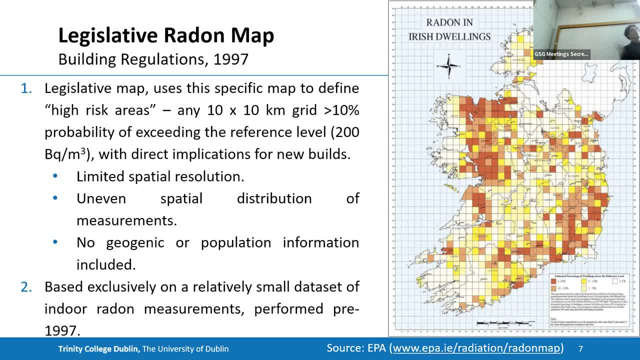 is a radar barrier under the foundation and this is to stop the ingress or to slow down the ingress of radon from the soil gas good getting into the house and any new home built since 1997 to have a standby pump or some fitted which could be activated at a later stage should high radon values be found. 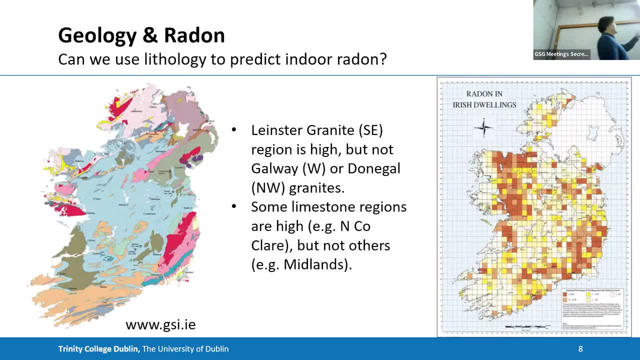 so that was all the starting points. now on the left hand side, this is my one geology map of ireland slides left hand map. we have a simplified geological map of ireland. the red areas are granites and the blue is a lot of limestone, mainly carboniferous limestone. we have some devonian. 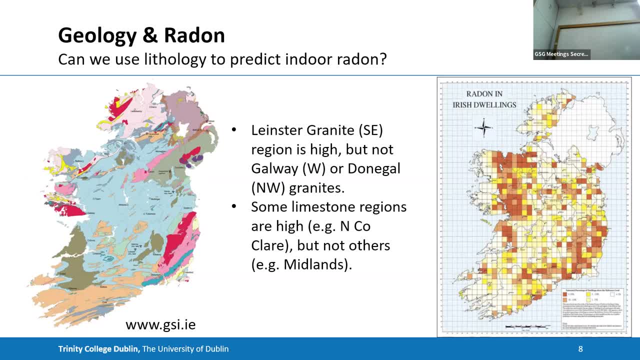 sandstones here, um limestones and shales and dark green, uh, metamorphic rocks in green, sorry, gray- and pink and yellow and antrum basalt in the northeast and that's you know, essentially in lithological terms. um, this is what we're looking at in this particular map. so we're looking at a lot of. 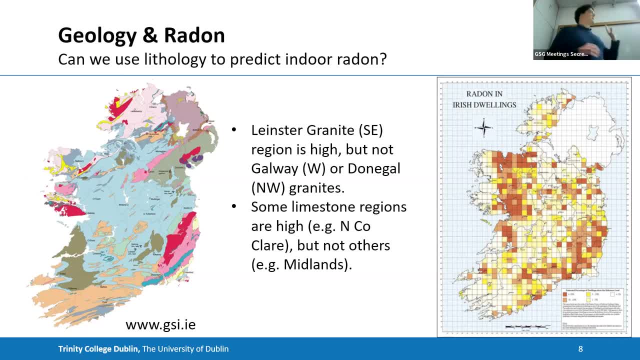 we have in the geological makeup of islands. If you compare the geological map on the other side and the ETA on the right, you'll see that there is some spatial association. Let's say, this is the Leinster Granite in Southeast Ireland in red here, and you can see that there are. 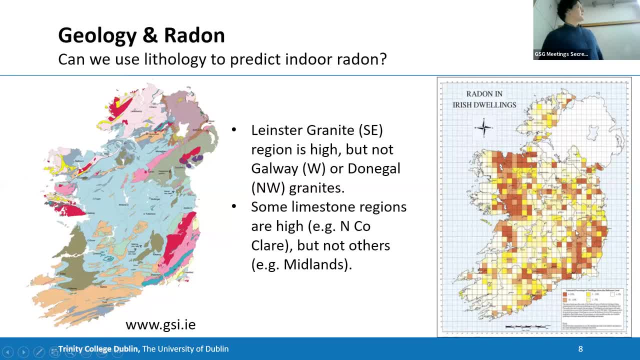 clusters of darker shades over here, which are the areas which are more radon prone or more likely. And again we go to the west. I'm from Galway originally and there's a graphical granite here, but if you look on the map on the right we can see that multiple of this A is associated with. 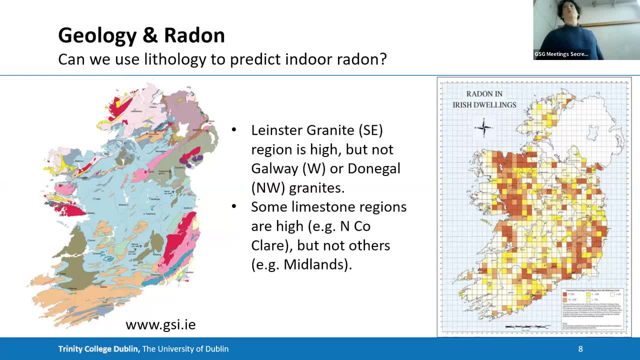 A original. So clearly material granites are equal. Similarly, down in the geograins up here in the northwest we don't see a lot of highly radon associated with these granites. So material granites are equal And probably like for most people in the west, the 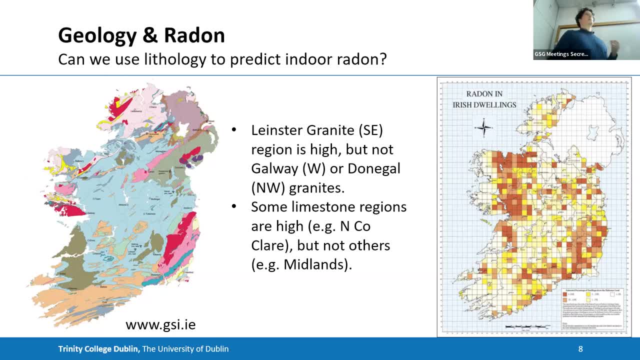 the phalange most commonly associated with granites. automatically people who know something about geology will say: granite. Yes, that could be the case, but it's not always the case. So if we look at some limestone regions, for instance, if we look at Middle County, Cliffs over, 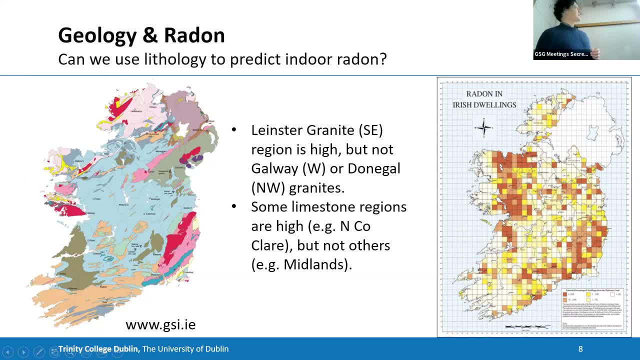 here in the west coast we can see there's a spatial association with. there's a band of highs over here and this is just of a division between different units in the Carboniferous. We also have a lot of shells around here, so that's the ground that we see And this is just a part of the. 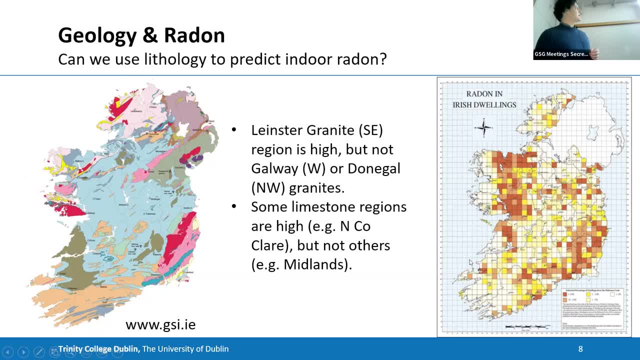 here carboniferous shales, and there's some shales around here and there are some highs over here, so perhaps that's a possibility. But the APJs of the Irish Midlands which are in blue- these are limestones- have been associated, at least spatially on the map, with highs. 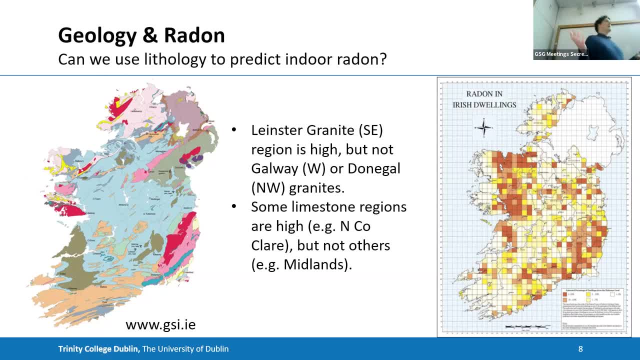 So yeah, just kind of a quick look at the angle of correlation. It's not really robust, it's not statistical, but we're just putting the two sides together and seeing if it can indicate spatial correlations. In some cases, yes, but sometimes it breaks down, And this was 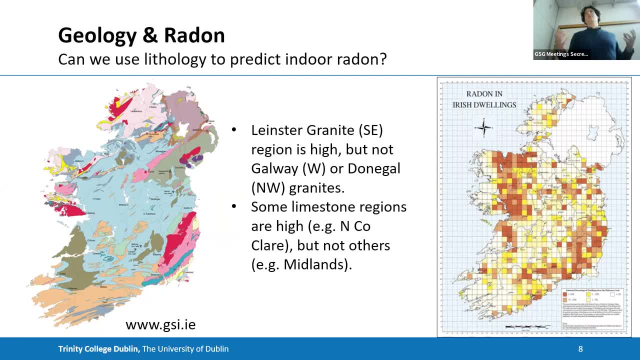 a first clue that there's something a little bit more complicated going on here. It's not just about the data. not all coordinates are equal, not all shales are equal, not all limestones are equal, and there's probably a greater degree of complexity in here that you'd miss if you're just 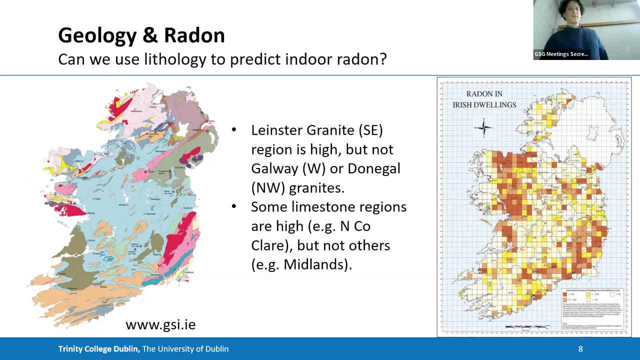 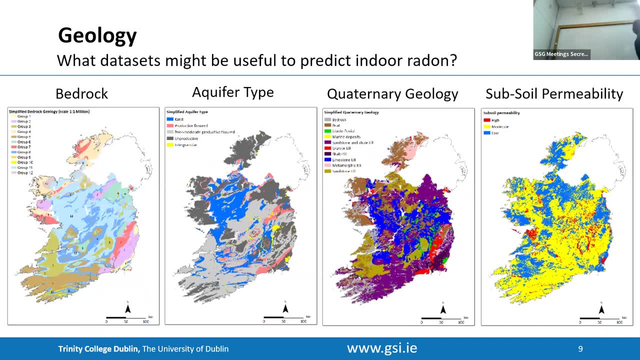 doing a simple comparison, So I thought: what are the other types of data sets that you could use? These are all digital maps produced by Geological Survey Ireland. Anybody can go onto the website anywhere in the world and download these data and a whole lot more. It's an amazing. 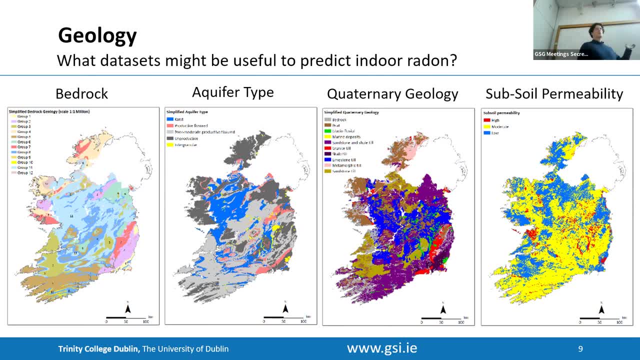 resource. Now, some of the mapping was done, for instance, by the Rock Geology Mapping going back to the 1800s. It's still happening in present day, you know. so there's a very, very long history of mapping on the islands of Ireland. So I'm going to talk about geography. 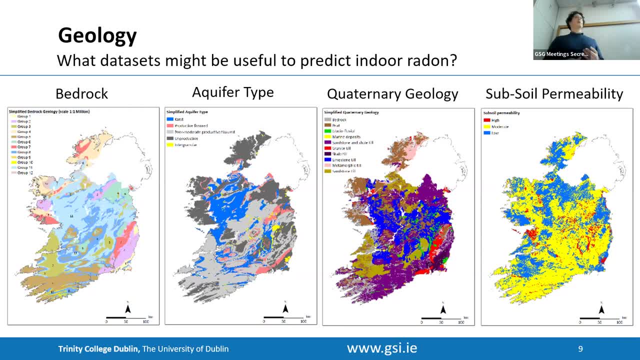 for shorter, but we'll look at what's aquifer type. So it's weakly sandy wooden water and it has a short half-life: 3.8 something days. So let's say you have a source area and you have some ground water and the groundwater can. 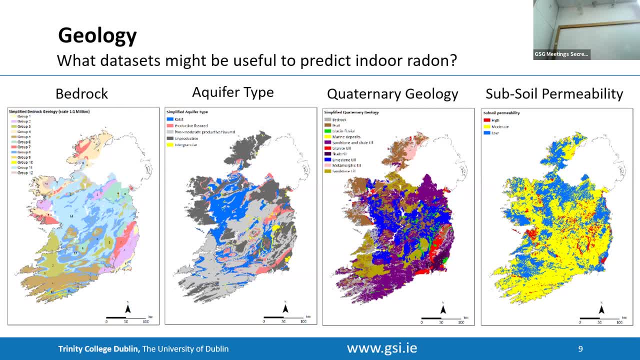 actually carry some of this radon and it can move it somewhere else And then it may degas or it may go to the surface and it may end up in somebody's house, And that house may be built over an ecology which is not commonly associated with radon. but the region hasn't been sourced in. 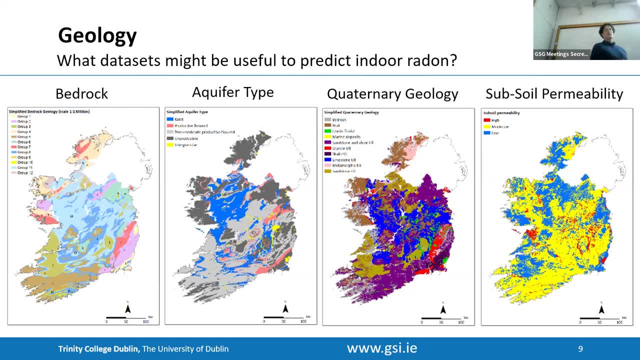 that location. So it's not necessarily associated with radon, but it's not necessarily associated with the geological mythology. It's ended up coming to the surface through that mythology. So I thought, okay, well, maybe aquifer type is an important geological characteristic. 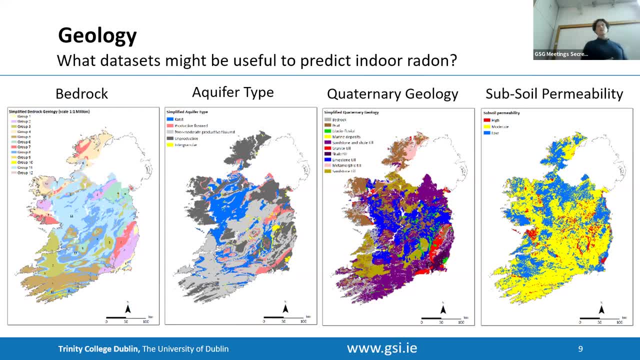 that we can include to try and understand radon. There's also quaternary geology. There's a really rich quaternary history and we have a lot of different quaternary types of sands and gravels. They have different types of. 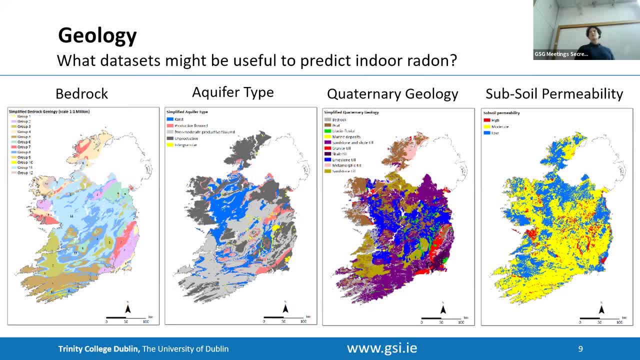 presence. They have different physical properties, different permeability, different landforms, and all of these things can help to affect radon at the surface. And then, with quaternary geology, in many cases we have soil, and those are characteristics of soil, both in terms of 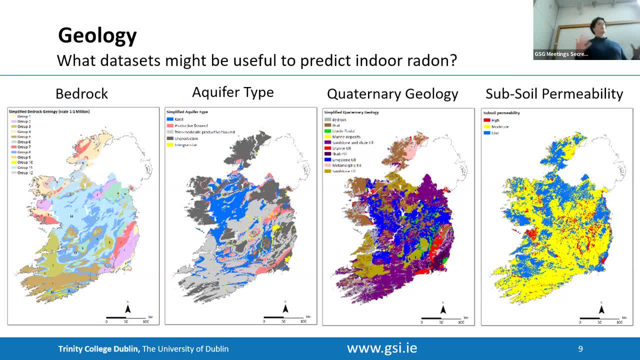 the mineralogy, but also the physical properties such as permeability. So I started to think- okay, I think about the source and I think about the pathway, and I think about where this ends up, And it becomes very much like a layer cake, like geology And each of these different layers. 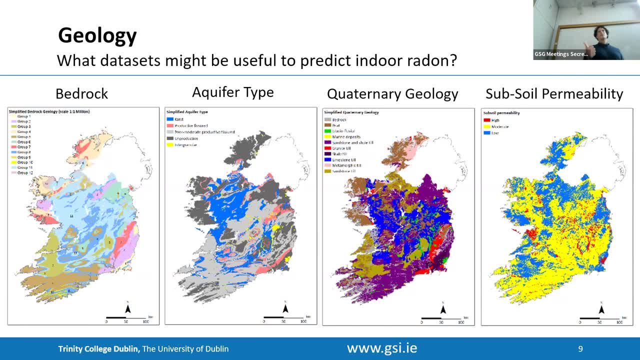 have different interactions. And so I think about the source and I think about the pathway, and I think about the intrinsic properties, whether it's the chemical composition, like the concentration of uranium, for instance, or radium, or the permeability, and how quickly. 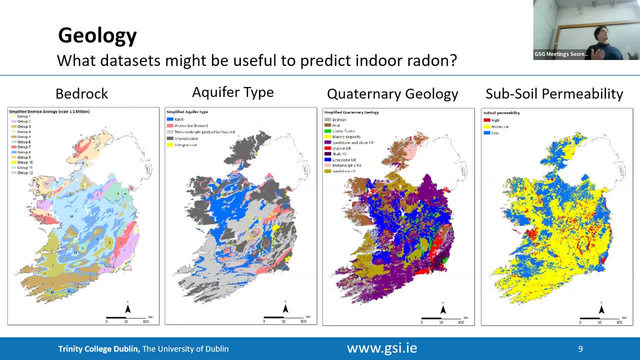 or easily can prime water flow through? Is it really fractured? So I suppose a question for you in the audience: what would be any other data sets that you might include in addition to these four that you can think of off the top of your heads? 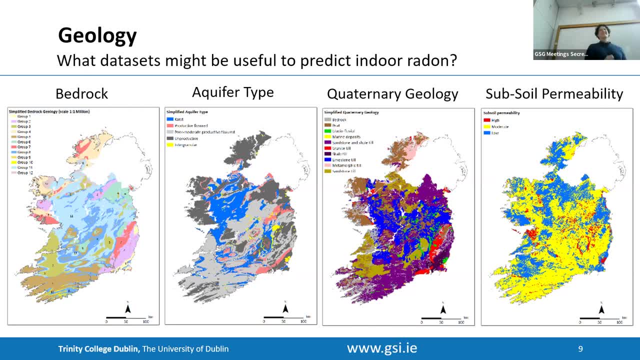 Is there more? No, I'll come back to that later. I'm thinking that you'd say on the geological map, What about the actual people, the NHS, that you're dating? Yes, That's definitely a consideration, but I'm thinking in a geological sense. 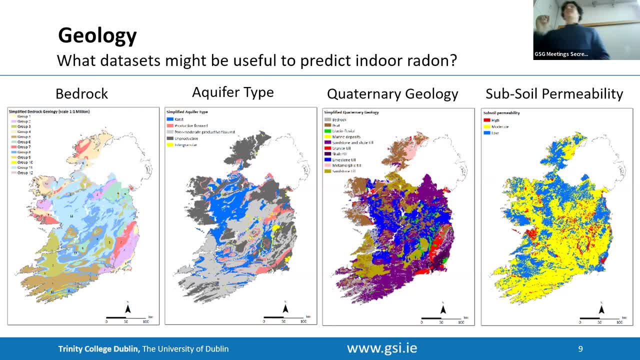 Well, you're right, okay, so it's really looking on hard and I just need to include them in this analysis because there's a little bit of uncertainty And there are faults and there are faults. you know, I talked about increased permeability and, for sure, some fault zones have increased. 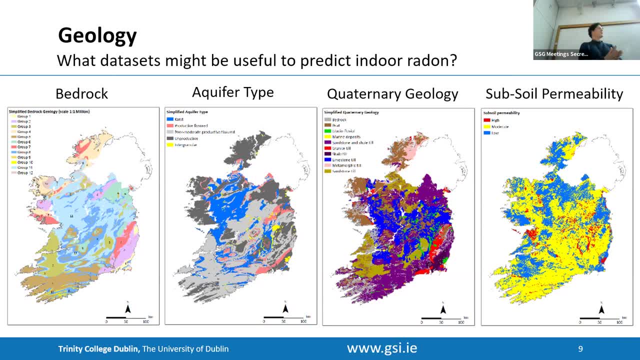 permeability. if it's a fracture zone, If these fractures are annealed or if it's mineralized, that fault zone can actually have lower permeability than the bedrock or the host rock. And when the fault is subsurface and it's unclear, there's a lot of uncertainty about. 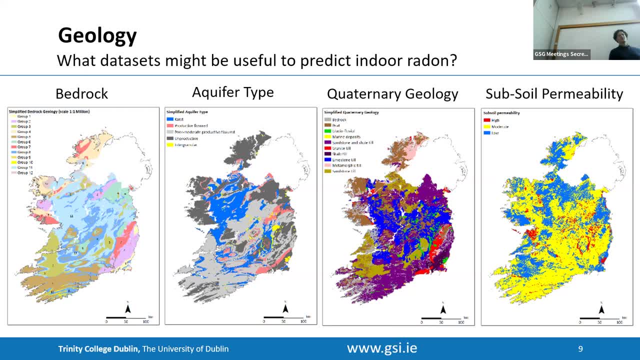 where exactly that is sited And it's 3D orientation. So if there's a better handle and more information and more details on faults and their exact location, whether they're mineralized or not, what they're mineralized with, definitely. 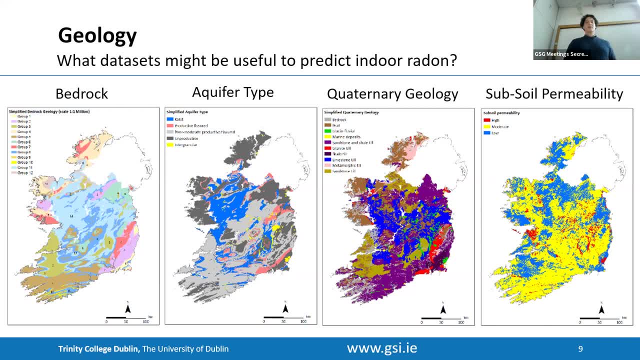 I would include this, But for the titan bean I've put it to one side and I haven't. So it's not the chemist who mentioned the four points. That's the kind of fault of the caledonium. Yes, 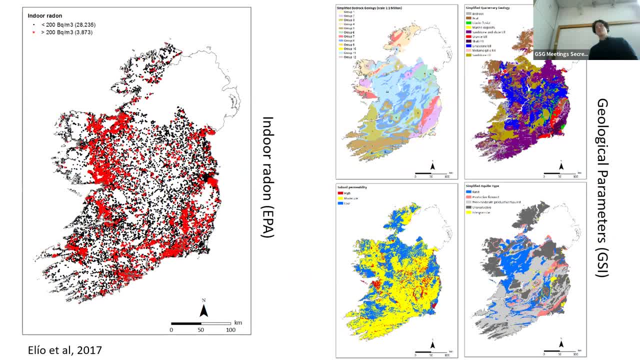 That in Scotland too? Absolutely yeah, because it just goes trans all the way through. yeah, So these are all of us, and it's not a geological map. It's actually geospatially resolved interladon tests. 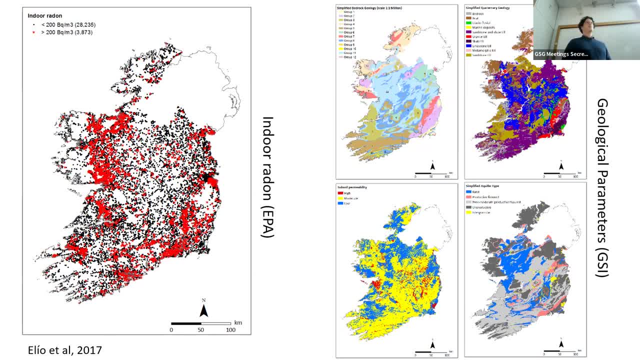 Now most of these have been performed by the EPA. in Ireland There's a number of private bodies and they used to send their data on an annual basis to the EPA. We'd put them in a spreadsheet and then put it to one side. 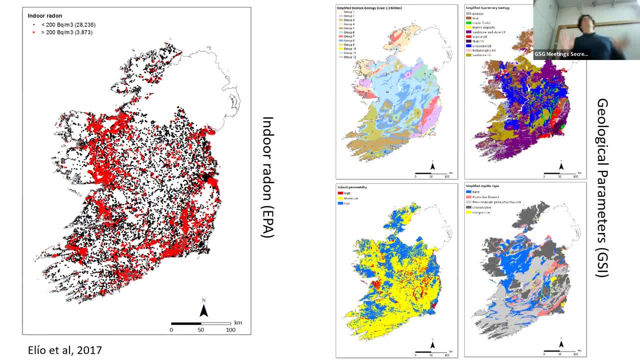 So several years ago I said I would really, really, really like if you would give me this data set so I can do some research and I will not make the exact localities identifiable like down to a house level. If I produce a map like this at a national level, we can't see whose houses have been. 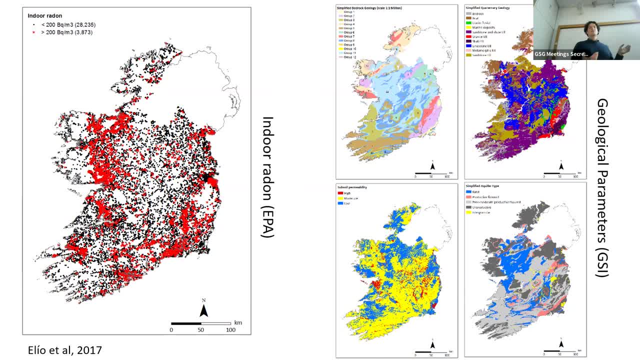 measured and whose haven't. We can see there are clusters. So the red dots are where there are indoor radon measurements greater than this threshold level I mentioned of 200 becquerels per cubic meter. The black dots are where they're below this. 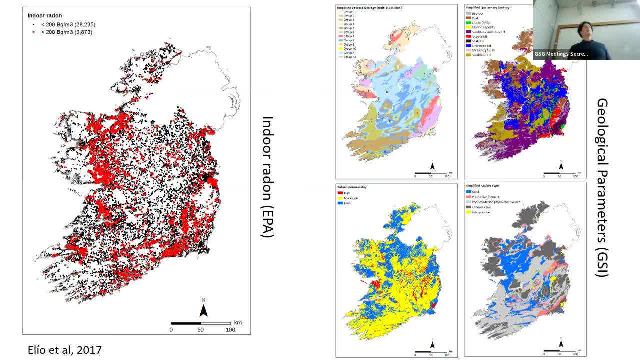 And the white. These are the places where there are no radon tests. So you can see there are areas of the country that have very few if any, and you see clusters in cities. There are also clusters around known highs. So if it's known, let's say your neighbor has a test done and they get a high value. 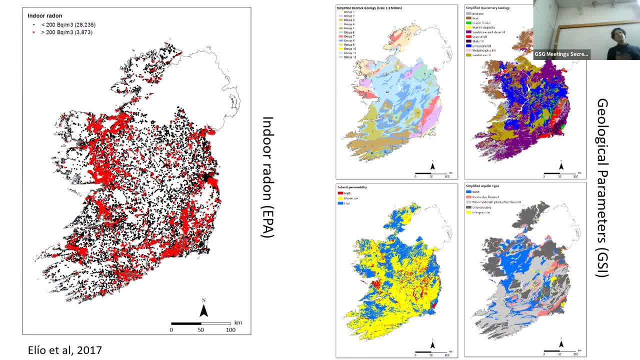 then this may produce an effect in the neighborhood where more people get testing done in these areas. So there's also there's a spatial bias in the data because of the way the population is, but because of the way people. what encourages people to test? 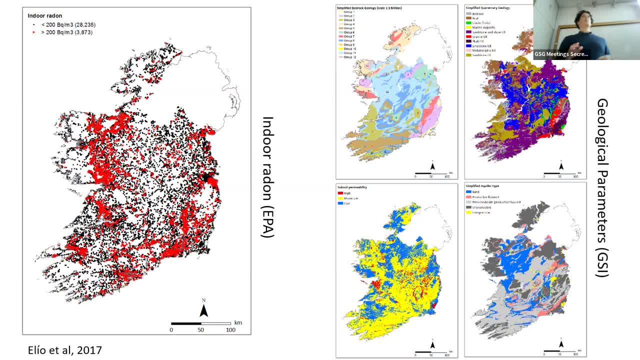 So when you work with any data set, you always have to be mindful of the kind of biases that may be introduced. So as a starting point, I thought: okay, I'm going to look at the bedrock geology, the Caternery geology, the aquifer type and the subsoil permeability and I'm going to 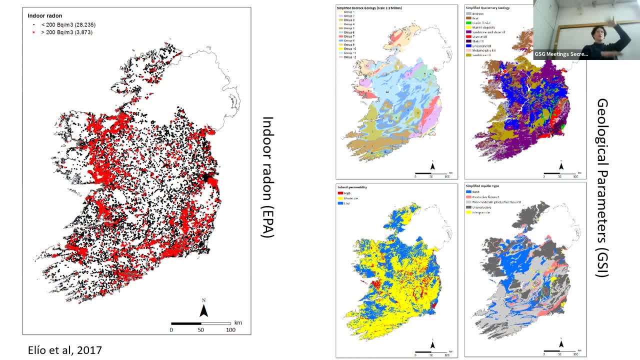 see how these intersect in layers. Okay, so I'm going to stack them one on top of the other and I'm going to investigate the occurrence of these radon highs at 200 becquerels per cubic meter. Okay, so I'm going to look at these radon highs at 200 becquerels or above for all of. 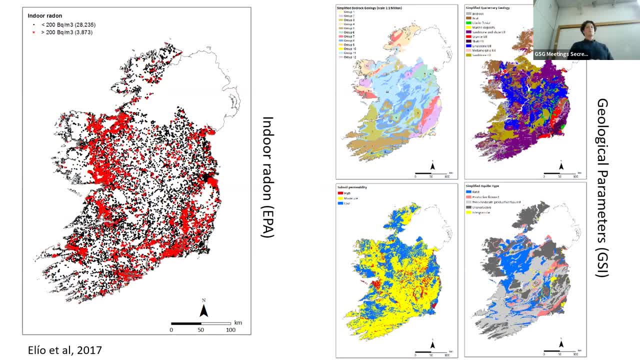 these points in relation to all of these different variables in the subsurface, and it's a lot of variables. So, for instance, there are 32 simplified to 20 or so. It's a one to one million scale for the bedrock geology map. but then there are about the 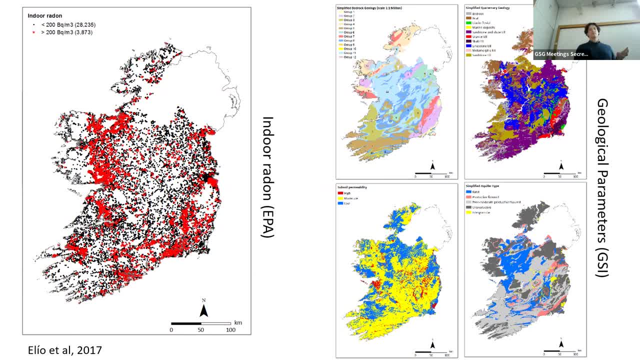 same number of Caternery geology. There are only, okay, three or four types of subsoil permeability, and all of these are simplifications, really to make the model. It's a little bit simpler, but you get the picture that it gets complicated very quickly. 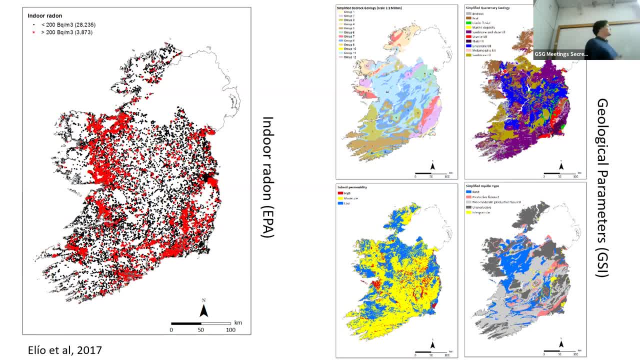 I tried lots of different styles of modeling, but one I settled on in the end actually came from epidemiology. Now, I'm not an epidemiologist, I don't understand very much about epidemiology, but I did start reading scientific papers around how epidemiologists deal with spatial heterogeneity, how they deal with biases and 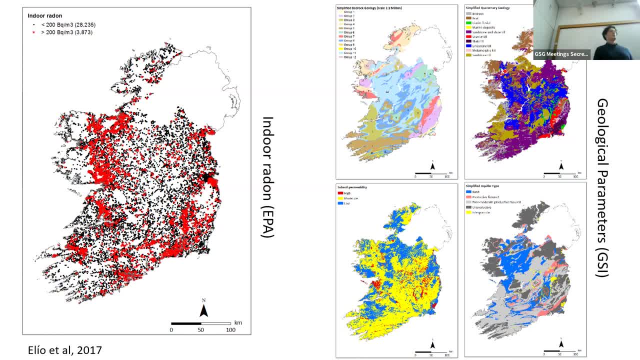 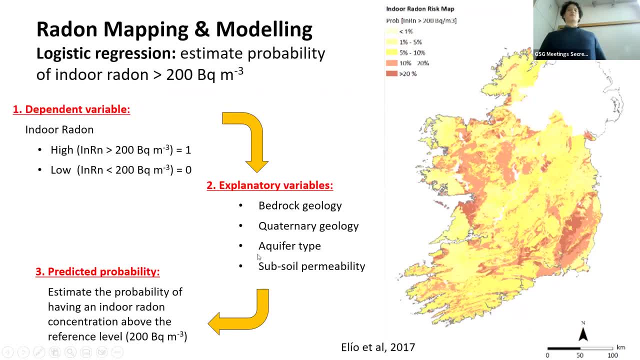 data sets and how they try and represent the spatial distribution of things like disease incidents, And there's one particular type of model that really caught my eye and the more I read about it I thought I think that's really going to work for radon. 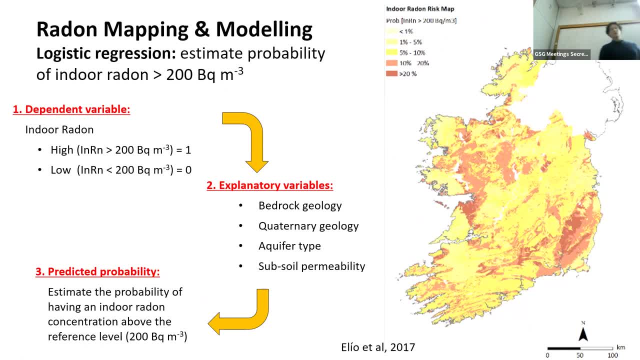 It's something called logistic regression modeling. I'll explain it quite simply. So I didn't invent logistic regression modeling. It's been around for a long time, but it was the first time that this had been applied to radon that I know of. 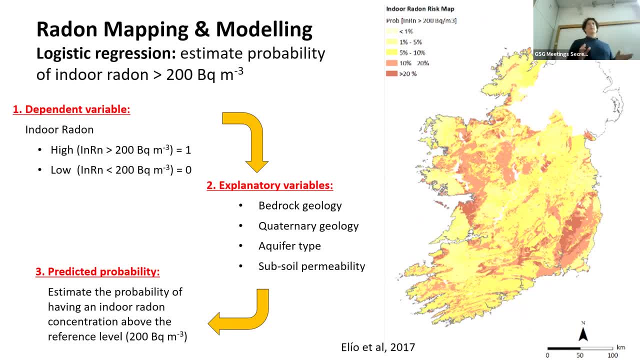 So the dependent variable is radon and I made it binary, so it's either black or red, It's either under or over 200 becquerels, just for simplicity's sake. It makes it easier to model. Then I have the explanatory variables, which are these geogenic properties I mentioned. 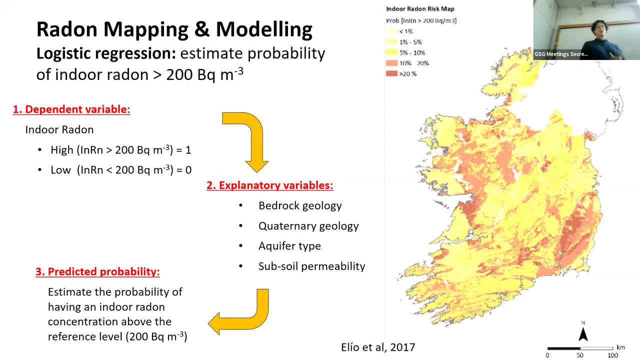 bedrock cuternary aquifer type subsoil permeability. And in the end, I have a predicted probability- and it's a prediction of a probability- of exceeding this threshold level for any point on the map. And this is the map I published with a postdoctoral researcher whose name- Elio- is there, Javier- 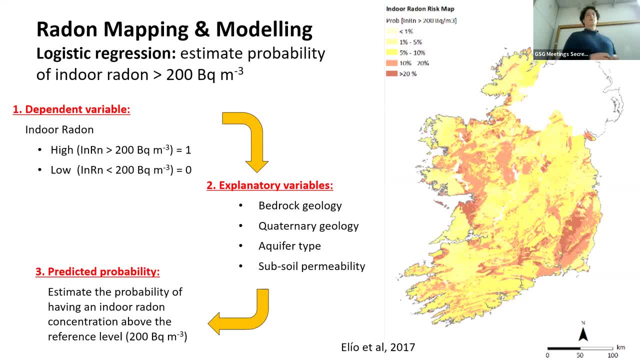 Elio, really, really talented researcher whose background was actually in geological engineering and had a very high skill level in programming. So I thought, great teamwork, I'll be the geological know-how, You can be the programming know-how. We're going to put this together. 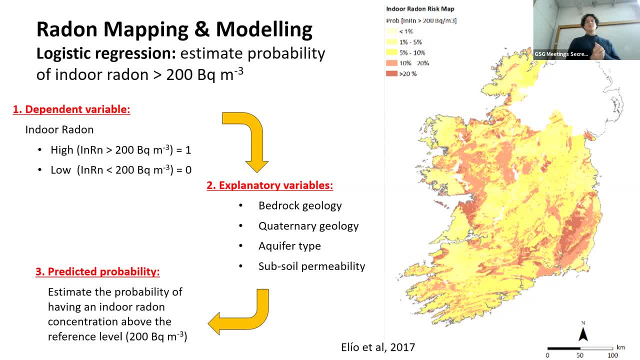 We're going to do something really cool. So we published this map in 2017.. And straight away you can see it's not pixelated. Each actual cell on the map or each dot we reduced down to one by one kilometer square. 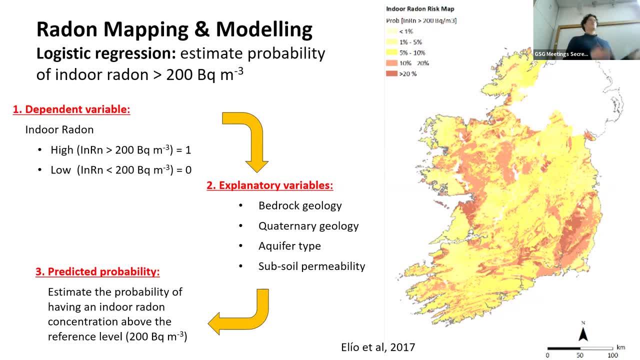 If you think back to the EPA map I showed you earlier, that's an order of magnitude higher. It was 10 by 10 kilometers. So the reason we could improve the spatial resolution of the map: partly because we have more indoor radar data points. 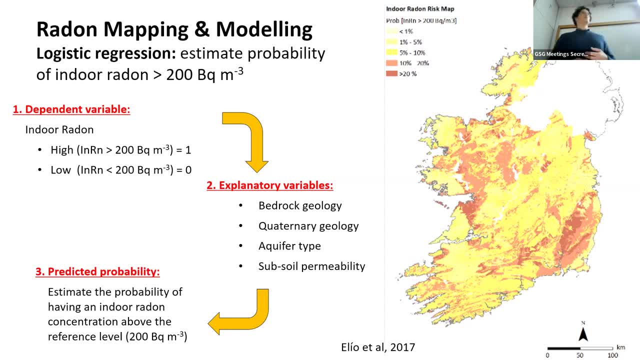 but also because we use these four geogenic properties. So really it was the incorporation of geology that improved the spatial resolution of the map. So that's the reason we could improve the spatial resolution of the map. So that's the reason we could improve the spatial resolution of the map. 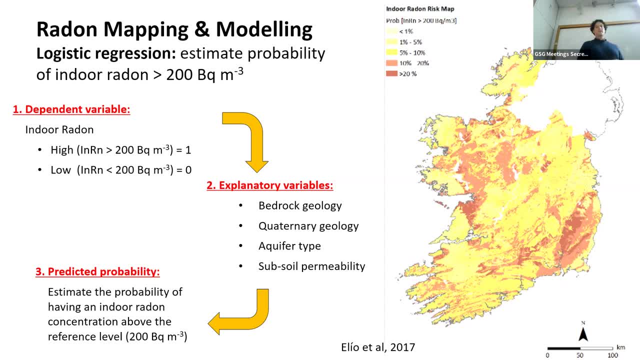 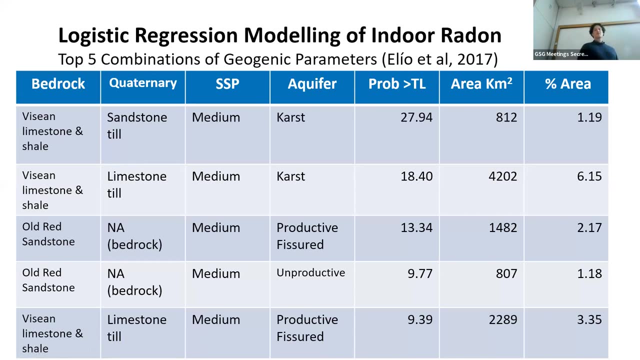 So that's the reason we could improve the spatial resolution of the map. It did cause a bit of a stir in the radon world, albeit the radon world is quite small, So you might not have read about it. And coming back to the whole notion of lithological associations and radon highs, 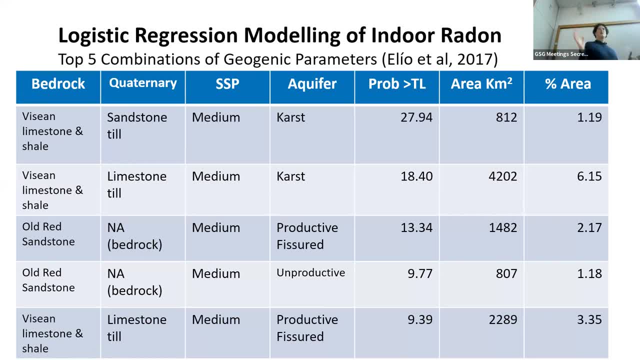 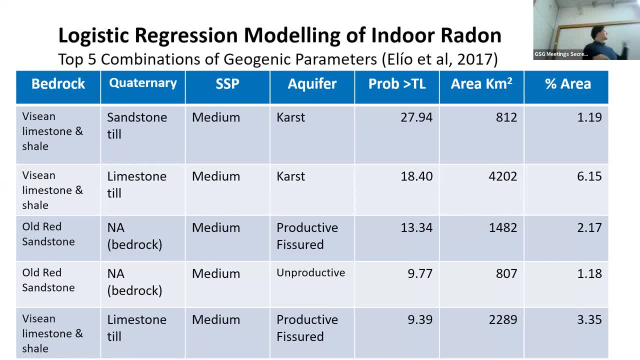 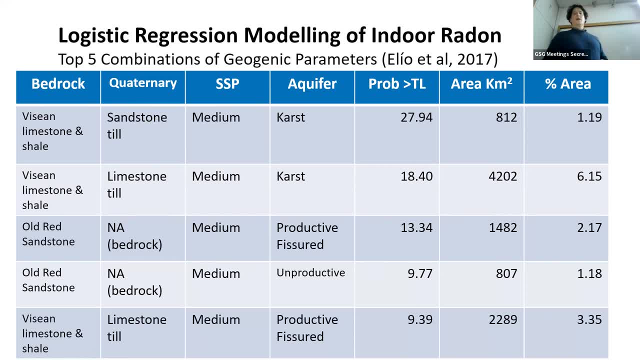 probability of exceeding the threshold level. that's TL and the area in square kilometers for that combination of parameters and the percentage surface area of Ireland. So the top association is Vizayan limestone and shale bedrock with a sandstone till a medium subsoil permeability. 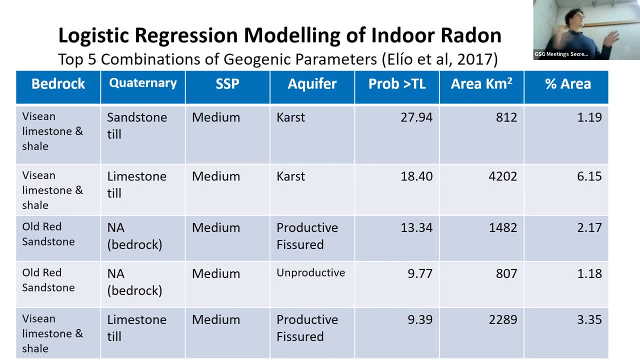 karstified aquifer and the probability. so if you had a house that was built on top of these four different variables, the probability for a house exceeding 200 becquerels per cubic meter would be just over, well, just under 28%. Okay, this only covers 812 square kilometers of Ireland. 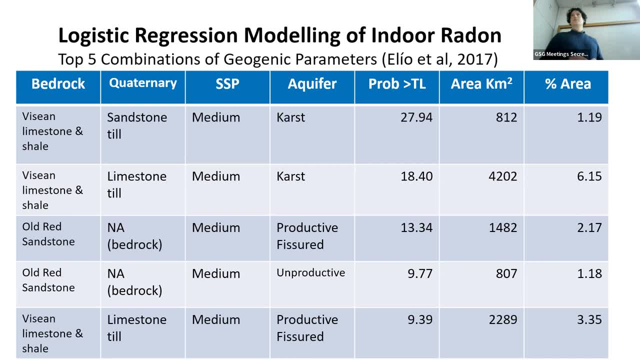 which is only 1.19% The total land surface area. So it's not a lot Okay. And but if you look at the next category again, we got Vizayan limestone shale, this time a limestone till medium subsoil permeability. 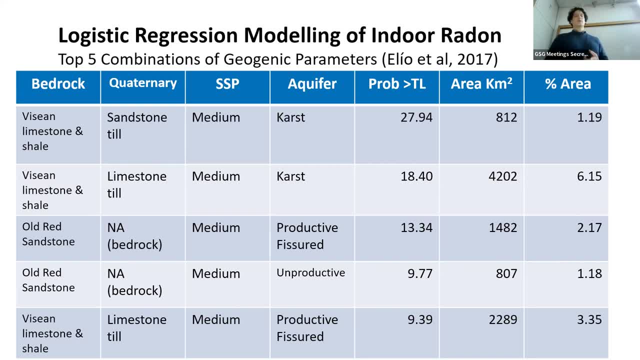 karstified aquifer, this time at 6.15%, and so on, so forth. So the top 1,, 2,, 3,, 4, 5 combinations of these parameters. granite actually doesn't feature at all. It comes down lower in the list. 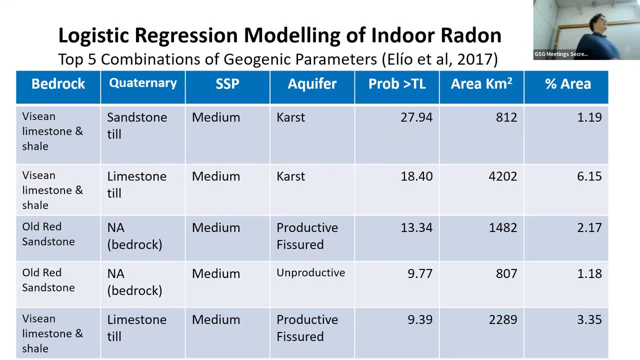 And this was an eye opener to a lot of people And I suppose as a communication message. people may be aware of the bedrock underlying their house and think it's not granite. I don't need to test, But when this became public knowledge there were a number of newspaper. 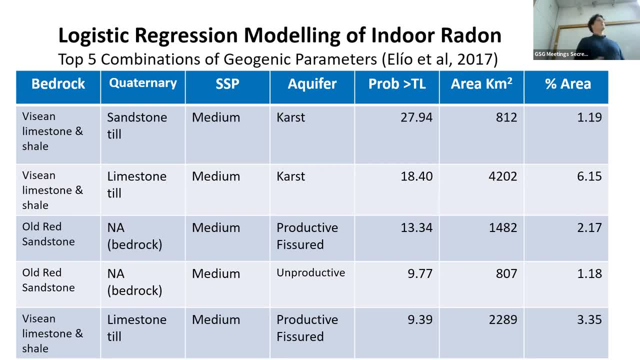 articles. we did radio interviews. you know there were websites. people phoned up, asked questions. the uptake in testing for the EPA went up exponentially after the paper. It was a blip. it did go back down again But it did encourage a lot of people to test but never tested before. 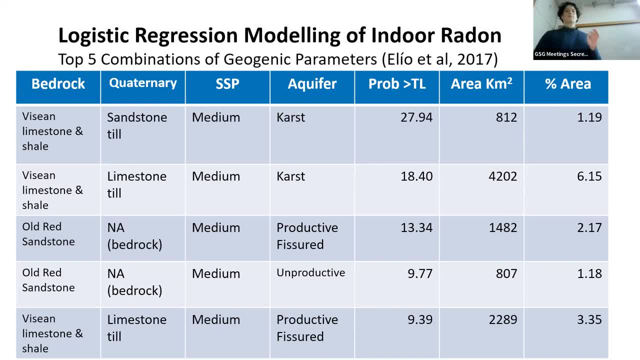 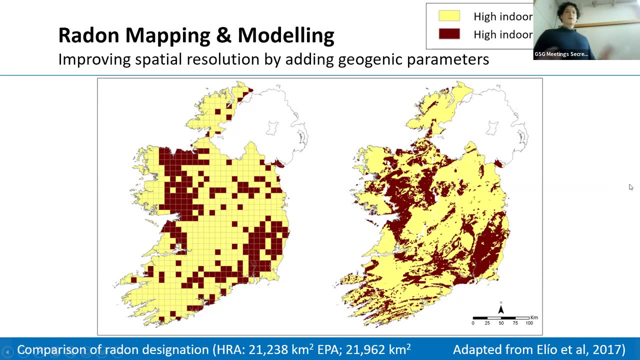 So I think there's a message there in that a better understanding of the subsurface, the geology under our feet, can actually lead to a better outcome in decision making for all kinds of things, including public health outcomes in relation to radon exposure. So I'll put these two maps side by side. they're simplified here. 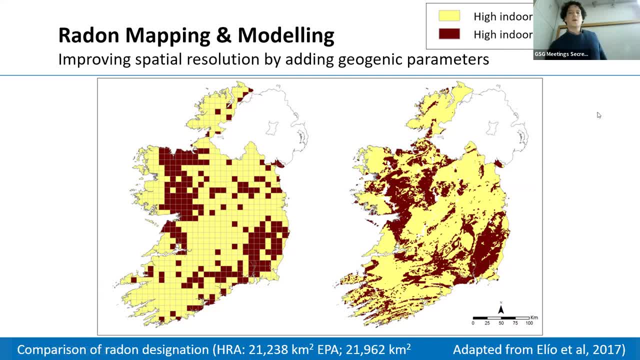 So they're just binary in terms of the colours. So the yellow is where high indoor radon is less likely, And I suppose the bottom line is that you can find high indoor radon anywhere. just because an area on the map that's got a light colour doesn't mean that it's not going to be high. 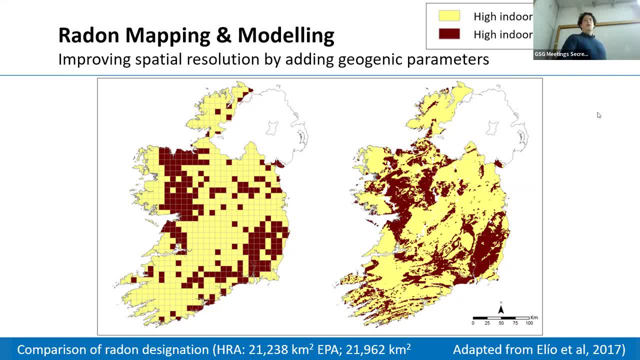 it still could be. it's just a lower probability And the darker areas, where high indoor radon is more likely or you know, has a higher probability. So you'll see, there's a difference not just in the spatial resolution but also in the distribution of some of these highs and lows. 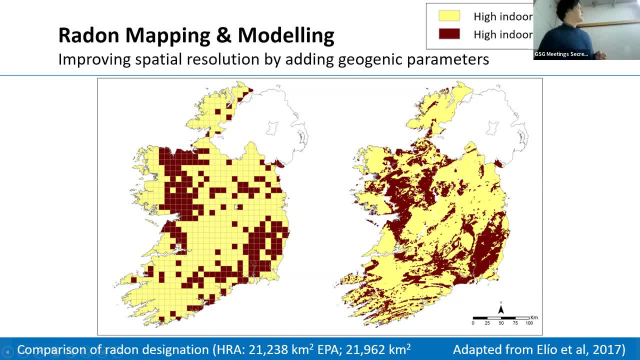 particularly, let's say, in the Midlands, which always used to perplex me, why on the map on the left that this was low. we did see at a higher spatial resolution and when we included the geology, that there are areas which are predicted to be high. 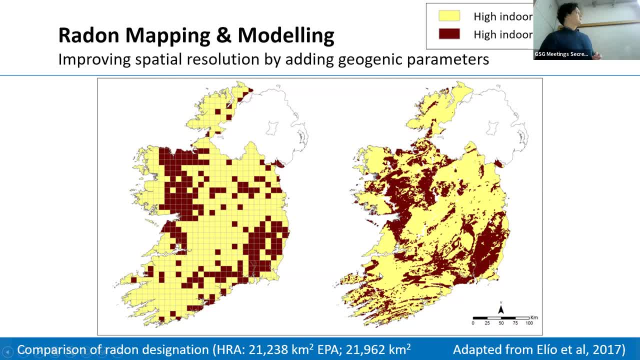 And certainly we can start to see some geological trends. So, if you can remember the geological map I showed you previously, this is a trend within the Carboniferous And this is a fold pattern that we can see in the Carboniferous limestone shales And it's clearly been picked out. 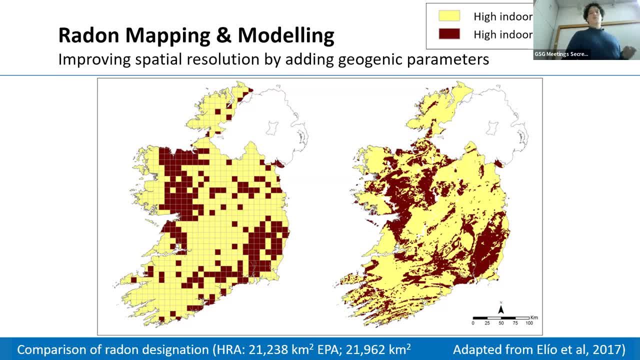 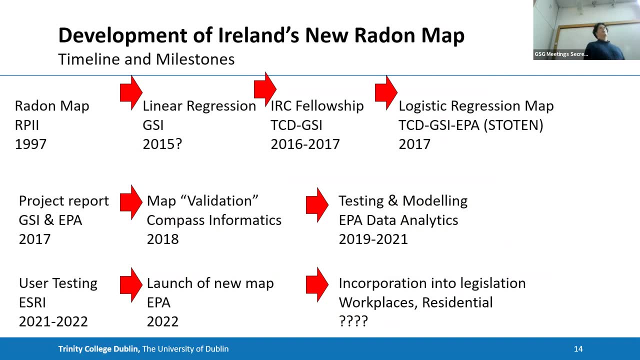 as areas which have a much higher probability of having high indoor radon. So putting the geology into the map seems to make a lot more sense. Now, if you're a sceptic- and I think it's really healthy to be sceptical- you might ask: well, did you test this? It was tested very rigorously And it was. 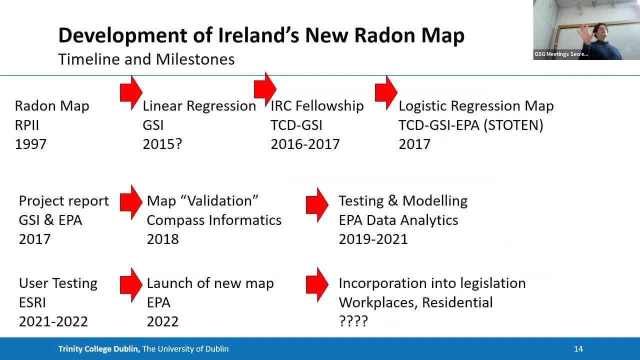 tested by us because we had a training data set and a test data set. So we treated the test data set as an unknown. we put it onto the map. we looked at the numbers of false positives and false negatives. That was good. 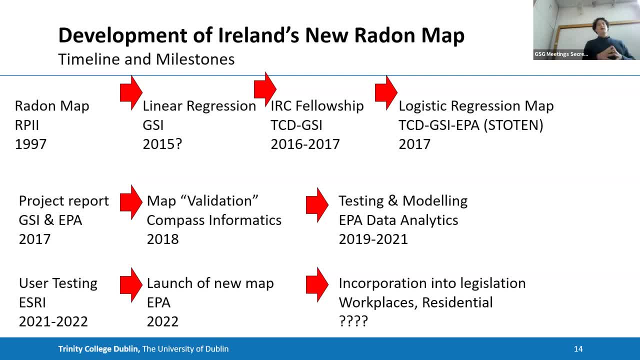 And we published this as a paper And we presented this in reports to Geological Survey Ireland and the EPA. The EPA became very interested in this because they were planning to update their map from 2017, but weren't really sure how to go about it, So we provided them with a possibility to 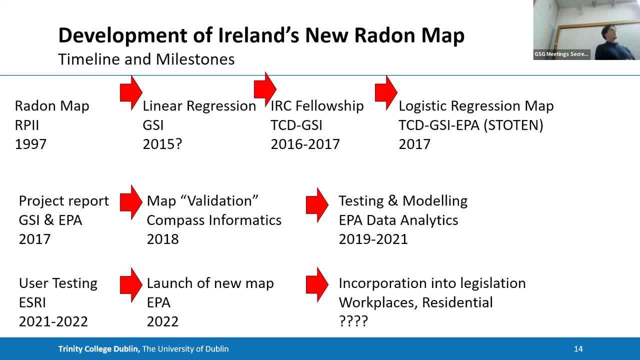 try it. They put this out for a government tender. It went to a third party who deal with a lot of geospatial information for the Irish government And they tested this and they validated our approach. They said, yep, this works. 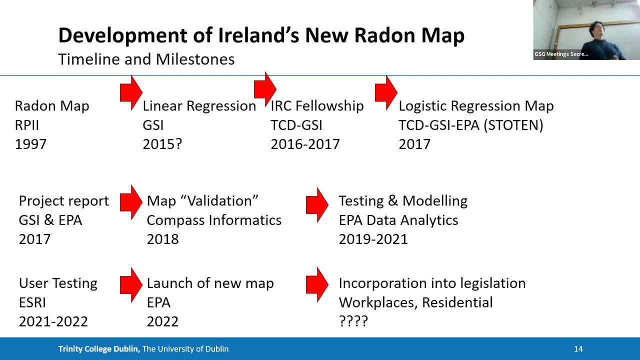 And then it went to the EPA. The EPA took this on as a training exercise to develop an in house data analytics team, And they worked on this for over two years. It coincided with COVID, so that slowed things down, And then it came back to us as a work group with the GSI. 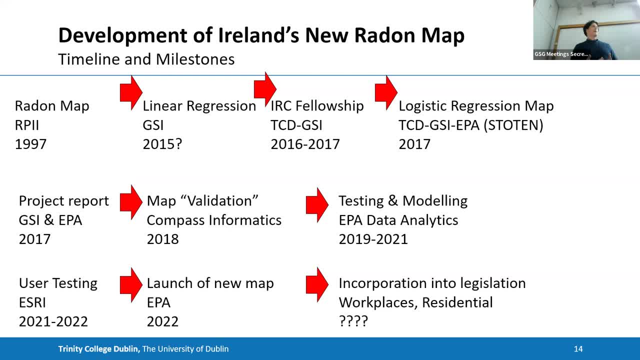 with the EPA And it was finally launched as a new map in May of this year, 2022.. It has yet been more, it has yet to be incorporated into all the legislation and but it's still there now as a reference map and the expectation is it's going to replace the old map and legislation very soon. 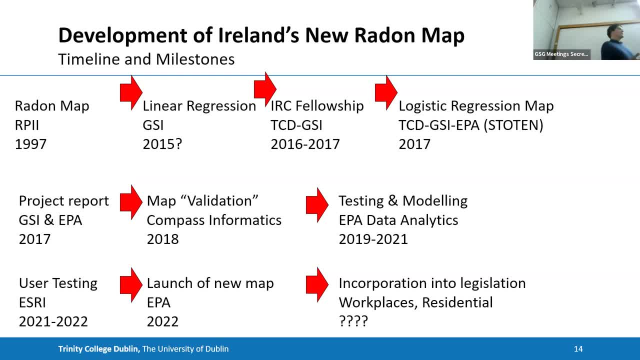 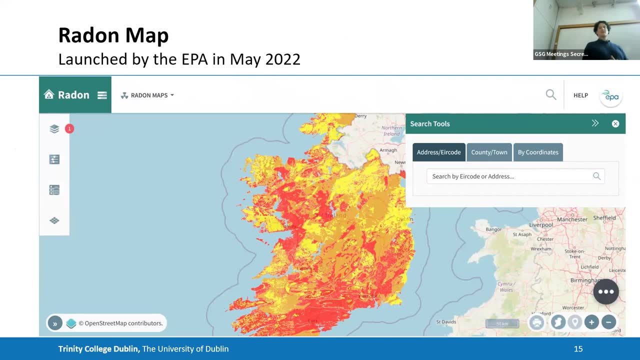 and the complication is that it covers both workplaces and domestic residences and they fall under the remit of different government departments. so it means that they actually talk to each other and cooperate. so it may take some time, let's see, but the map is there. if you go to the epa website, epaib, you can put in your postcode, you can search by geography, you. 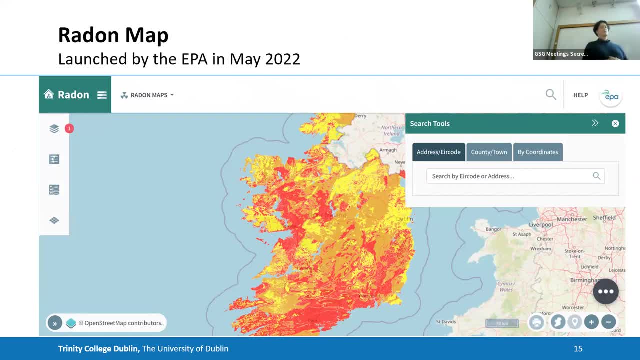 can zoom in and out, and i think that's something to be really proud of. it's a piece of research which just started as concept and a small bit of funding for a two-year postdoc and small research group to do something to integrate geology and then produce this as a new product or service. 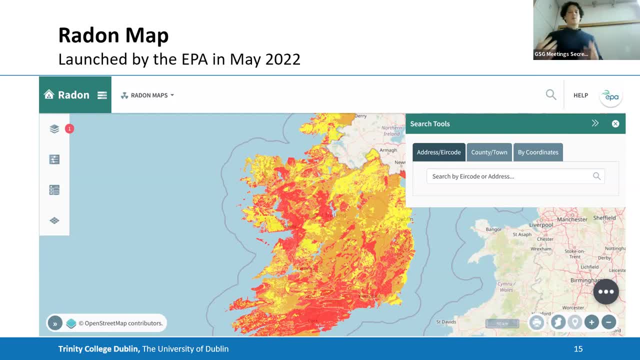 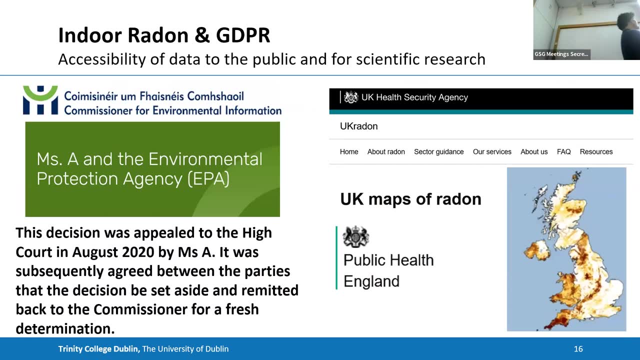 which you know potentially can benefit everybody, something i'm really really proud of. so let me come on to the whole notion of data sharing, and gdpr is the general data protection regulation, which is an eu-wide legislation. um, and this whole notion about access to data to do 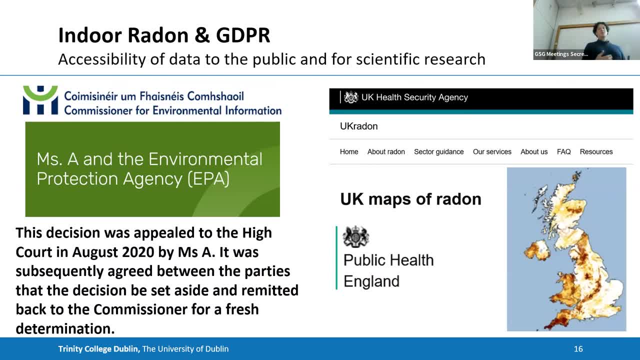 research. so um several years ago i was contacted by the green party in ireland out of the blue um and they were proposing, or thinking of proposing, a new um bill around healthy homes, primarily because of the fact that the green party in ireland is the only party in ireland that has a 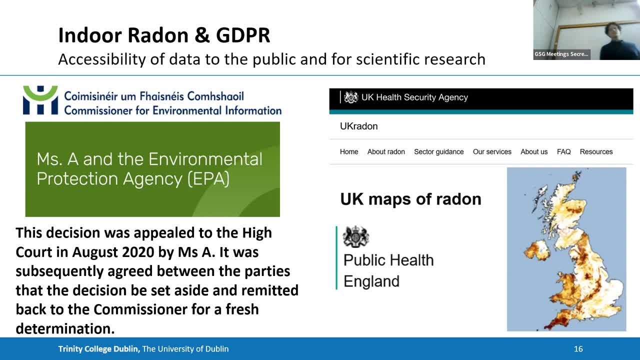 for the rental market- i think actually exclusively for rental properties in ireland, so about one third of all properties in the country are rental properties. um primarily about thermal insulation, but also there was something in there about indoor air quality in relation to radon. so one of the 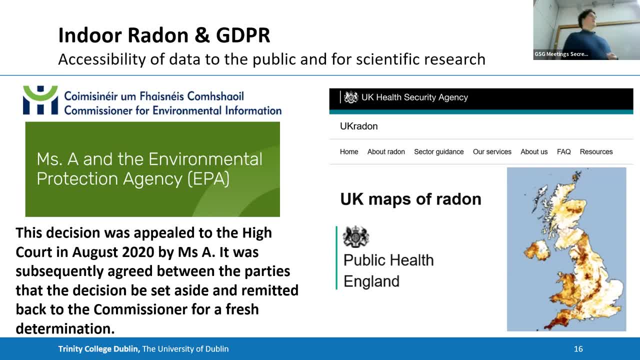 researchers in the green party went to the epa, said this is my address. i'm renting an apartment in dublin. i'd like to know: has it been tested for radon eps? the epa said no, we can't tell you gdpr. so they said: okay, could you tell me, uh, what the average concentration from my neighborhood is? 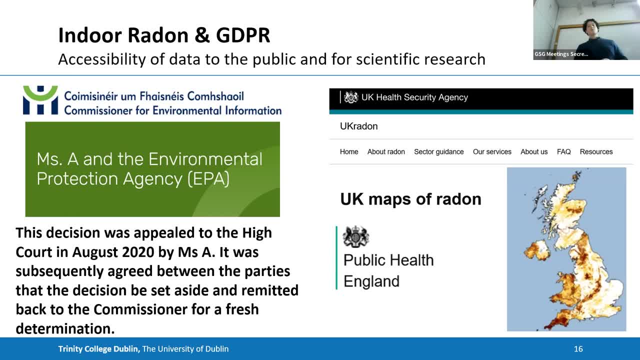 they went: nope, we can't tell you that. so the individual decided to take them to court and it's escalated and escalated. it's been to the high courts and it went to the data protection commissioner or the commissioner for environmental information and it's gone back and forth and it's. 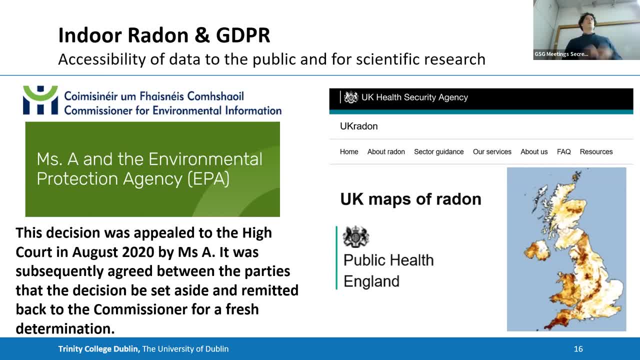 still not resolved, actually, but this has thrown up um a whole can of worms around the country, and what's going on is that the people are saying that the people have lost their property. um, and so what is the outcome on the part of the city of town? is there more evidence? 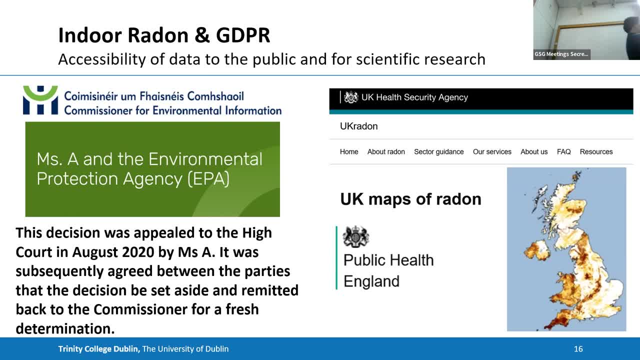 for so-called um. and now, if there's no evidence, what's the outcome of the case? um, it's just, it's not that i mean, it's just so a lot more data to write about, and i was just thinking about this a little bit and um, but i'm not completely sure that's the answer. i would say: 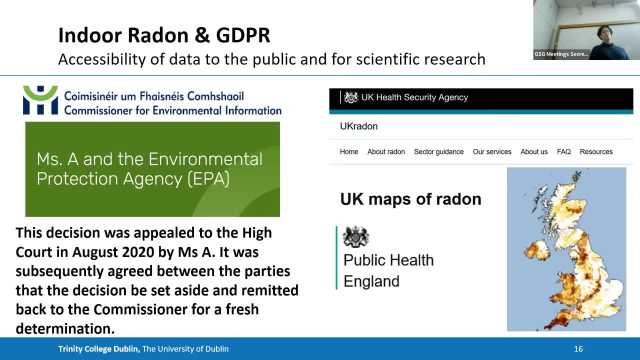 that's uh. the answer is that there is information about the history of the data that is being used and we should have access to this information. it does throw up a can of worms in terms of value of property if you own a house and try and sell it, and so there's nothing in law in ireland around. 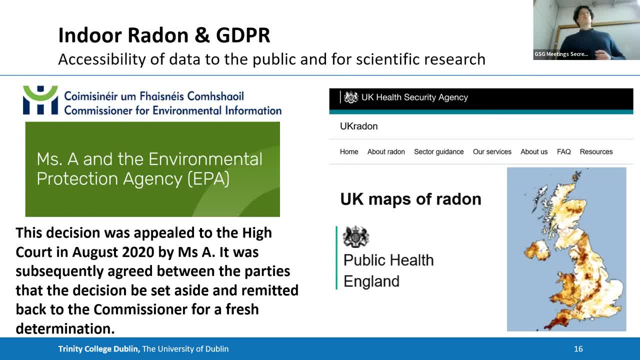 that at all. i know in the uk there is, and and also for rental properties if it became known that a property was higher rate on who's going to want to live there really. so there are implications for sure, and i do think this needs to be tested again in court, and but i also think that there 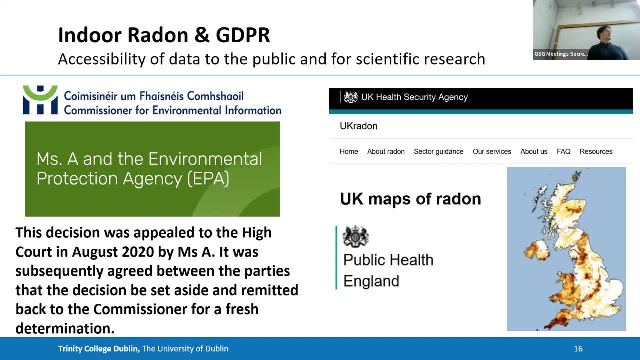 needs to be proper provision by the government to cover remediation costs if high levels are found. there's another side to this. you might have noticed in the map that i showed you that there's a gap for northern ireland, and there's a reason for that, not just because it's northern ireland. 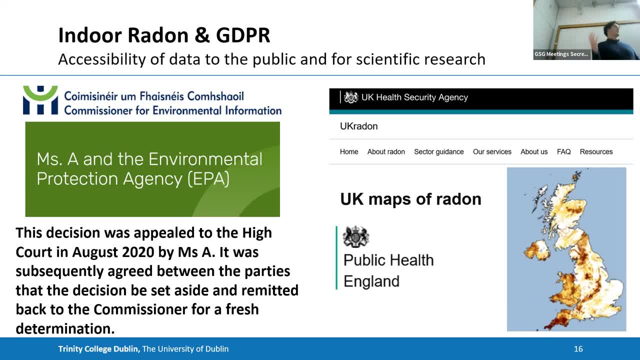 i would have loved to have produced an all island map of radon. i was not able to because i could not get access to the point data for indoor radon for northern ireland. so i spoke to colleagues in the northern ireland environmental agency. they said they do not have access to the point data they gave. 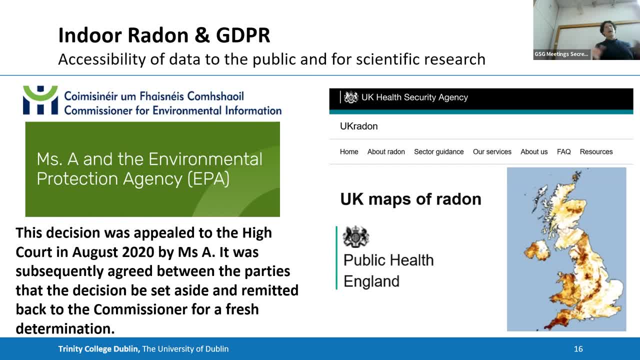 me their maps, which everybody has access to, and these are aggregated data by small area, but the small areas are really large so really i can't do much with that. and they referred me on to the bgs. actually i used to work for the bgs in keyworth and nottingham for a number of years. i know the. 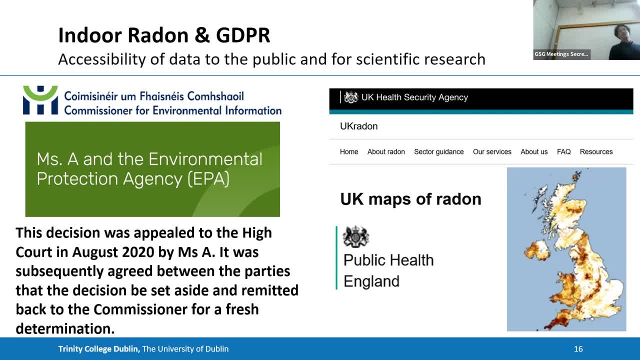 team who have worked on the map and there has been this new map produced. they said: we can't give it to you. you have to contact what was then public health england. contacted public health england- nowhere. so i think there's something interesting there about what kind of data should be shared for. 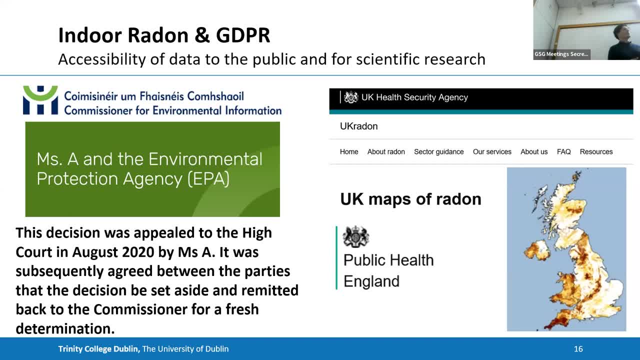 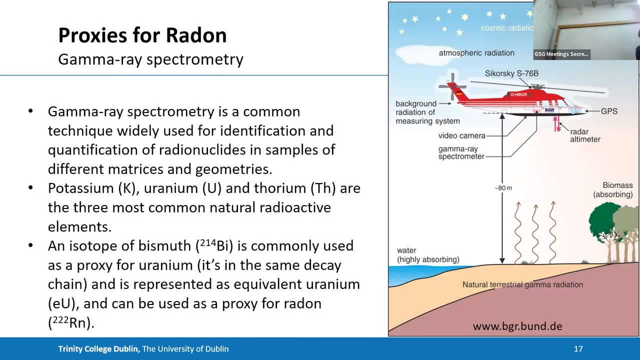 the public good and i would argue a case that this should be shared. indoor radon data should be shared for the public good. currently it's not okay. okay, so i'm a problem solver. i love a good challenge. i love a good problem. i thought i'm. 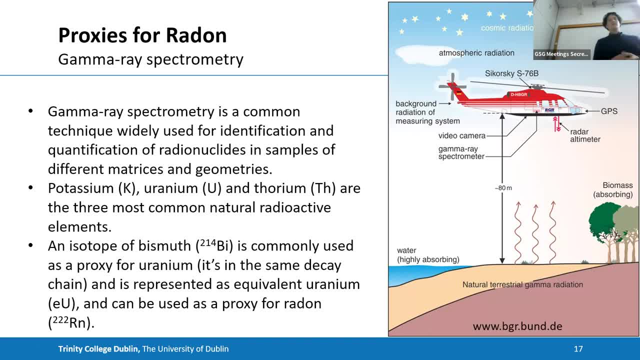 not going to stop. no, i'm not going to let the lack of access to indoor radon data for northern ireland stop me from producing an all ireland radon map. what else could i use? well, i have the geological maps. okay, that's a start, but the method i've used in the past has combined indoor radon. 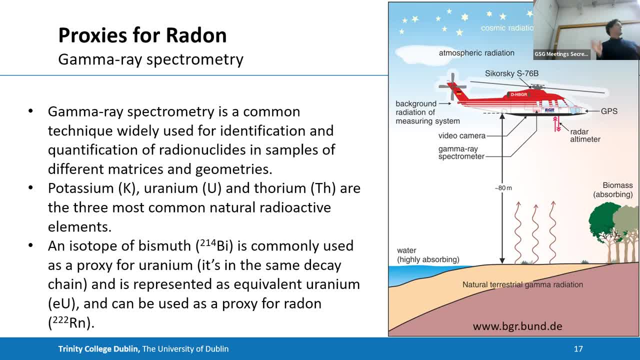 with the geology maps, and the geology of northern ireland is very different to the rest of the island of ireland, so i can't infer what's the indoor radon concentrations i'd expect for northern ireland and above the basalts, because we don't have basalts like that. okay, so i thought your point about radiometrics very valid and so. 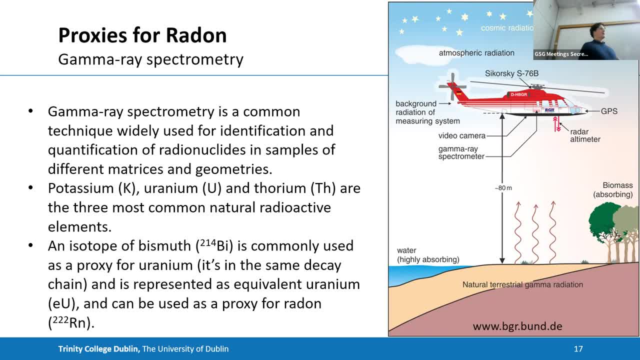 gamma ray spectrometry. it's a technique which has been around for a very long time and there are elements which are naturally radioactive. they give off different styles of radiation and we can pick up these signatures of radiation and use the energies of these to actually pinpoint which 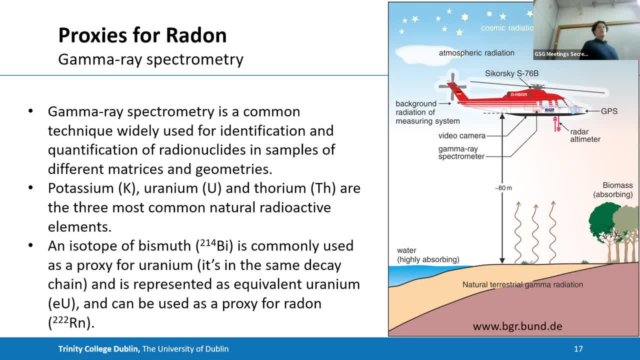 element is emitting this radiation. so the most commonly occurring radionuclides on the earth's crust, on the surface of the earth, they're potassium, uranium and thorium. and we can use these techniques, whether in this case, in this schematic, from a helicopter, or with a handheld detector, or with 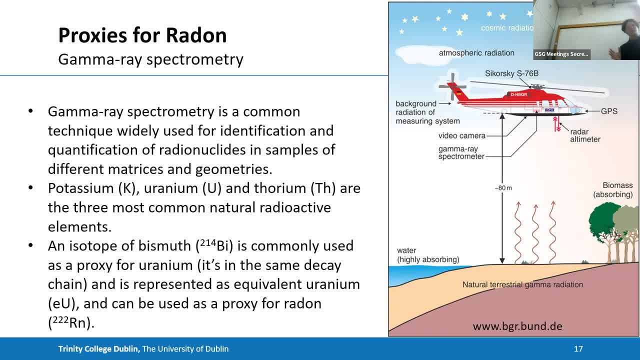 a backpack or, even more recently, with a drone and a miniaturized detector, and we can create maps. and we can create these maps for these elements that can be used for different styles of mapping. it could be economic geology, it could be bedrock geology, it could be radon. now remember, at the start i said uranium-238 is the parent isotope. 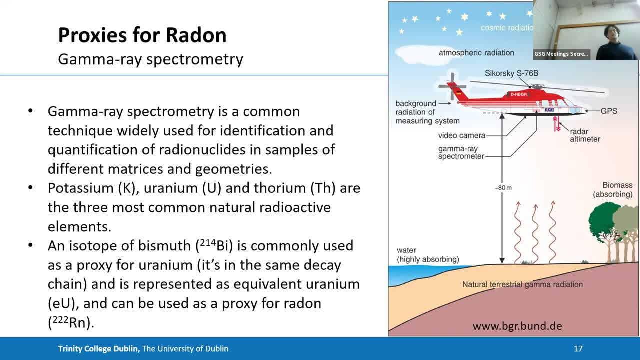 of this decay chain where we have radon-222. so i thought, if i can use the gamma spectrometry maps for uranium, perhaps i can use this as a starting point in a model, as a proxy or a substitute for radon. now the thing is: 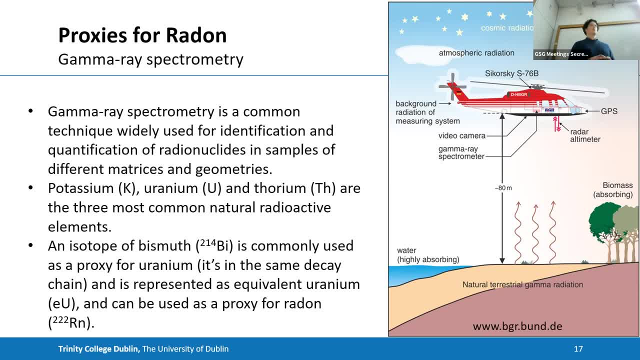 the gamma spectrometry doesn't measure radar doesn't measure uranium directly. it measures one of the daughter isotopes. it's a bismuth isotope, bismuth 214.. it's easier to measure than uranium and it's commonly used as a proxy or a substitute for uranium. you might see a small e and a u. 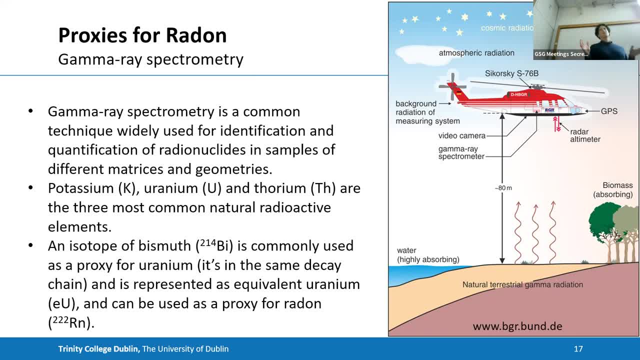 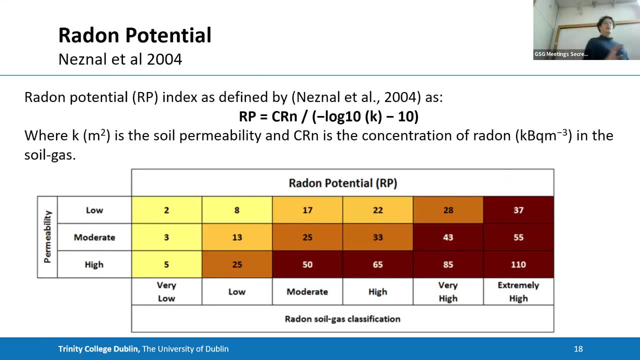 it means equivalent uranium. so i thought, well, actually i'm more interested in the radon. so i converted the bismuth 214 data to equivalent um radon and that's what i used as a map. now, very luckily, um, there's a known correlation between the 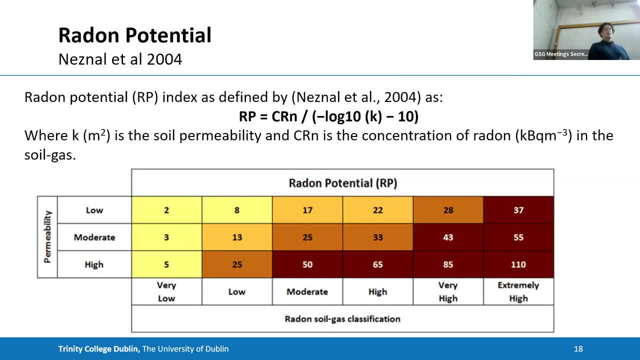 concentration of radon in the soil, the permeability in the soil and the potential of exceeding a certain threshold level of radon, and this it's called the radon potential, or sometimes geogenic radon potential. it was developed by scientists in the czech republic, or what was then czechoslovakia. 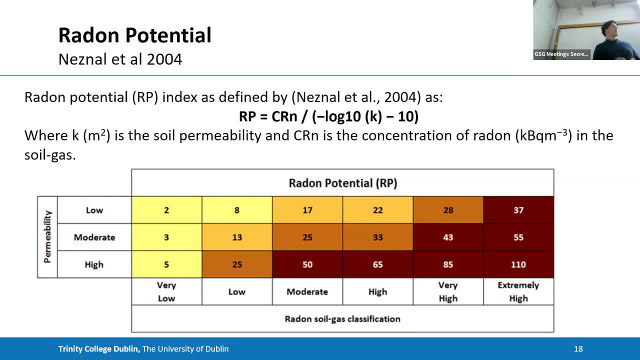 are the only EU member states who have this enshrined in their law. if there's any new bills take place, they must measure the subsoil permeability and the soil gas- the radon concentration in the soil gas- over a certain number of measurements over the intended footprint of. 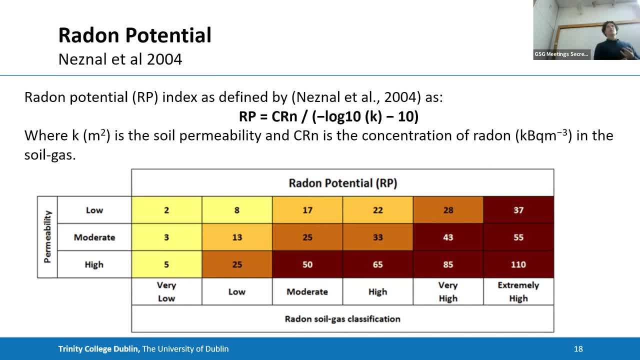 that house They use this formula: It's a function between the radon concentration in the soil and the permeability of the soil. And from this matrix, and if this value was over 35, they say you must put in preventative measures like a pump or a radon barrier. And I think this. 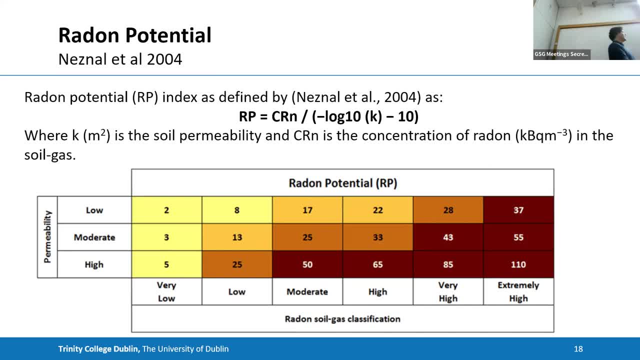 is a really, really sensible approach. If you think about the maps I showed you previously. with the indoor radon, there are large data gaps in the maps. So if you have what's sometimes called a greenfield site, if it's an agricultural area and it's rezoned for housing and houses are 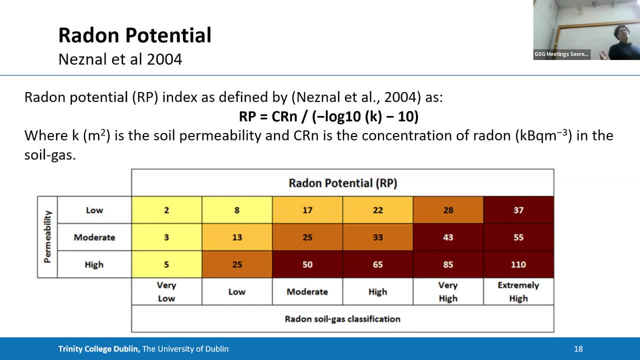 built there for the first time, that means nobody's measured radon there ever, Because nobody's ever built a house in it, at least not in living memory- Whereas if you use this technique, you can measure directly in the soil and you can infer what you would expect to. 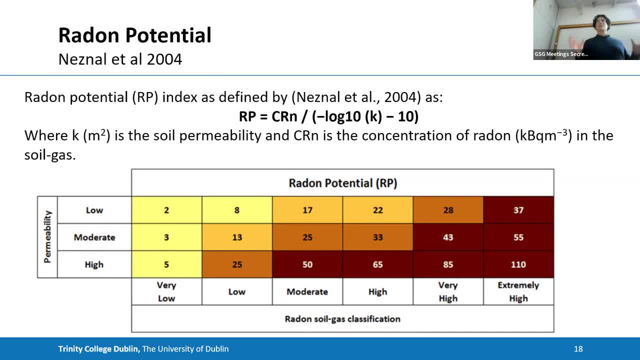 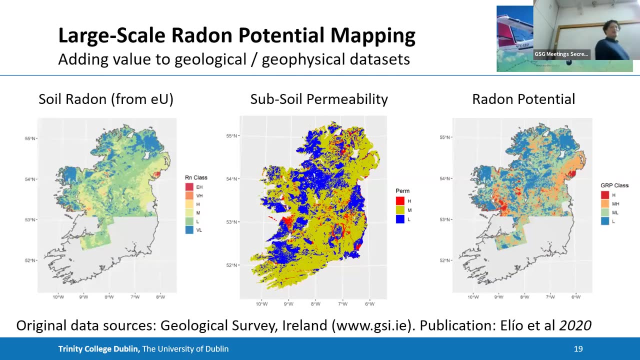 find in a house, should a house be built there. So I think it's like a really eminently sensible approach. yet there's only one EU member state that has this in law, And I think there should be more, and even non-EU countries. So back to the radiometrics. The map on the left. 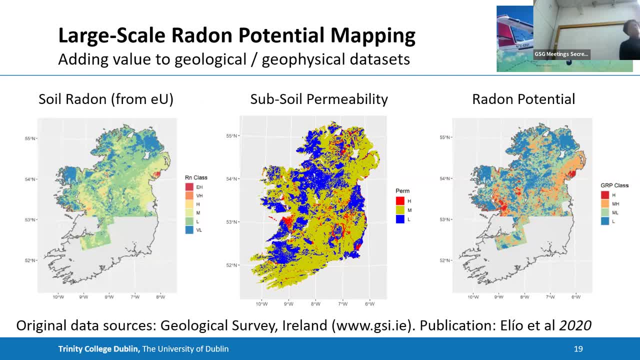 the map in progress. in time which I published was 2020.. So you might have heard of the TELUS survey. It started, there was a TELUS Southwest in Cornwall, then there was a TELUS Northern Ireland and then slowly it's moved southward across the border And it's a combination of airborne. 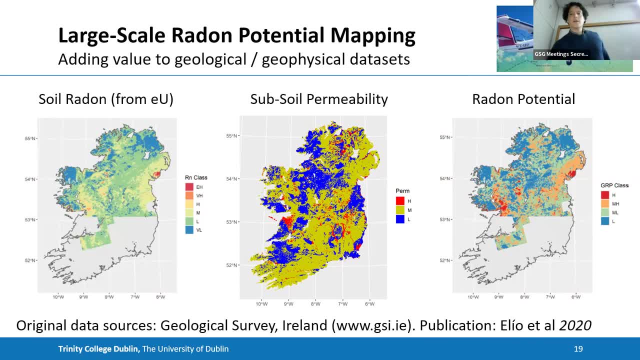 surveys and ground surveys. So the airborne survey is conducted by this plane, or one like it, and it's measuring three different geophysical parameters, including radiometrics, gamma-ray spectrometry. And the ground-based program are things like soil sampling, soil geochemistry, water sampling, heavy mineral separates from streams, sometimes vegetation. 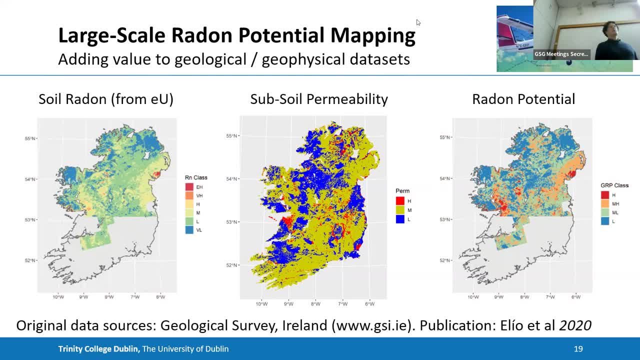 samples. So it's a huge collection of different types of data sets again, which is all free to download. It's amazing. So, starting from soil radon, which is inferred from the bismuth, really, rather than the equivalent uranium- the subsoil permeability map which we derived. 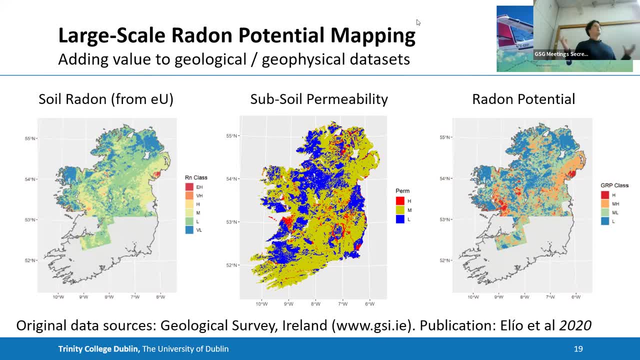 we can produce this radon potential map And, lo and behold, you'll see it also includes Northern Ireland. So this is something we published a couple of years ago as a methodology really, And it did again attract quite a lot of attention because a lot of geological surveys 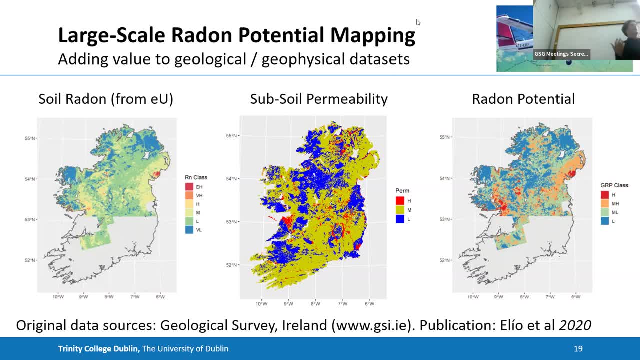 a lot of private companies. they hold these old archived data sets such as the gamma spectrometry, and they've never really thought about using them to map radon. So in a way it's kind of adding value to existing data sets to showcase. 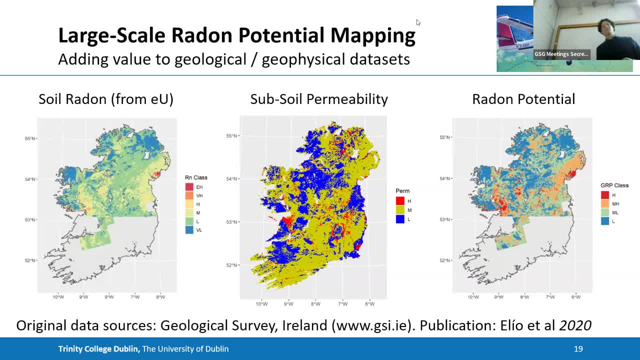 Look, you can use this data set. It may have been collected for mineral exploration or economic geology, but you can use it for a totally different purpose And this is very useful. It's useful for society. It can help planning. It can help you decide whether or not to test. 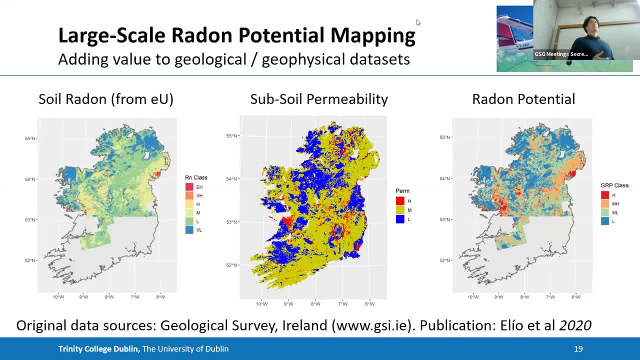 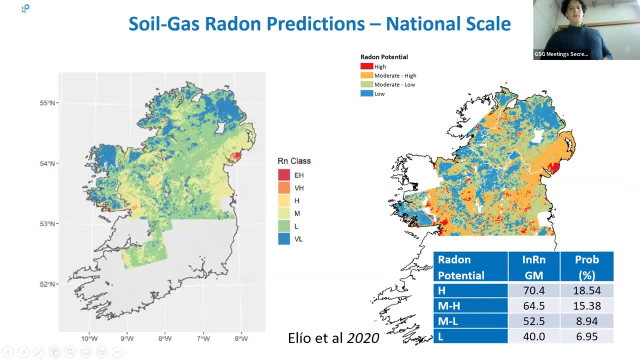 houses in a certain area, or what kind of preventative measures could be included in new bills, Like: why not use it? So again, you may think it's a pretty map and you may be sceptical about this, So we wanted to test it. 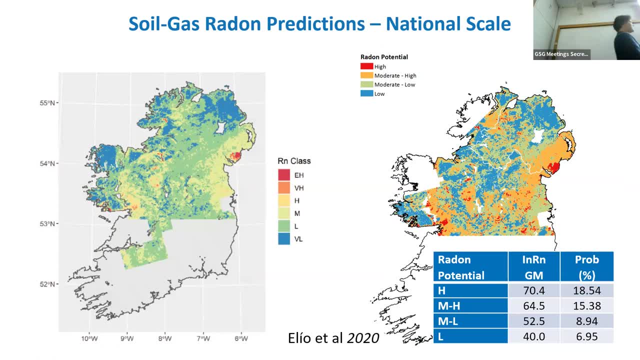 Now, indoor radon was not used in making the map. It was the gamma race spectrometry and subsoil permeability. But we then got the indoor radon map data points for the Republic of Ireland, not for Northern Ireland, And we plotted these on the map into the different 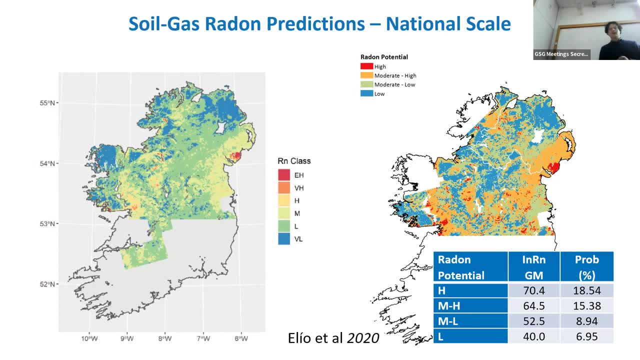 categories, different radon classes and the areas which are designated as high on the map. Now the model doesn't know Where the indoor radon is high. We've plotted them on the map. It gives an indoor radon geometric mean. that's a GM, It's 70.4.. That's becquerels per cubic metre. And if you go, 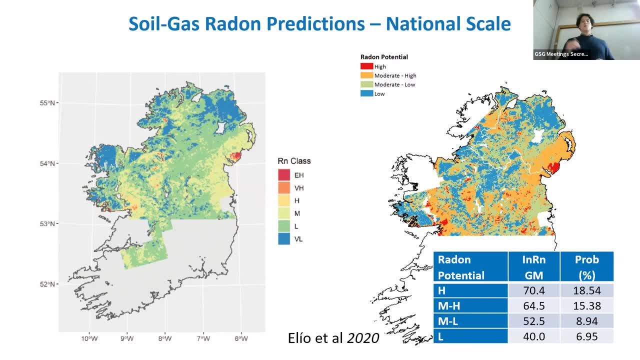 down the table from medium high to medium low to low, you'll see that the average concentration decreases, as you would hope it does. So, although the model is very simplistic, actually there are lots of things it doesn't include, like variability of humidity. 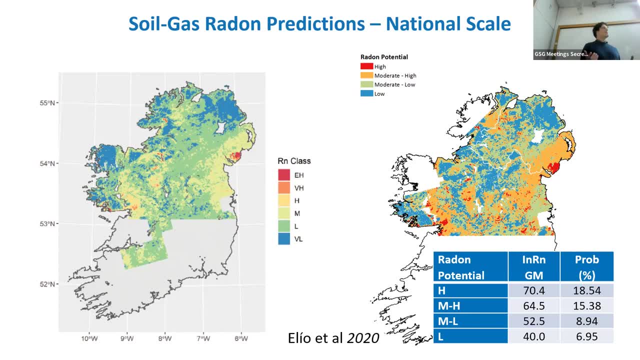 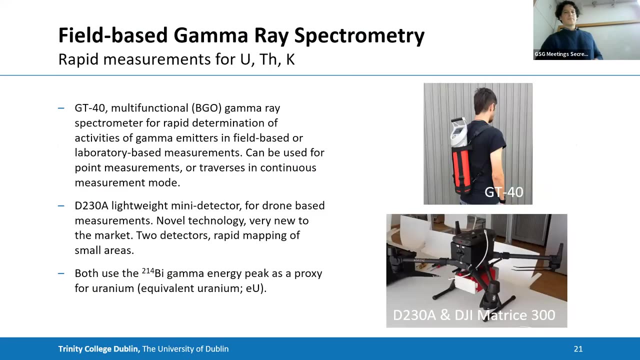 Or soil saturation or soil type. It doesn't include any of these things. It's just basic model and subsoil permeability and the gamma race spectrometry. It actually works really well And I think probably we could improve that with different data and more data. 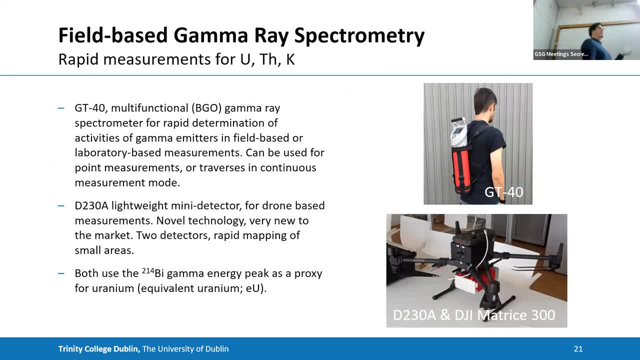 So that's the question: what do I do when I go on fieldwork, When I'm studying radon, typically I don't carry a geological hammer. I have to say, it feels really weird. Even now, I do sometimes have a hammer, but it's not a geological one, It's for hammering down. 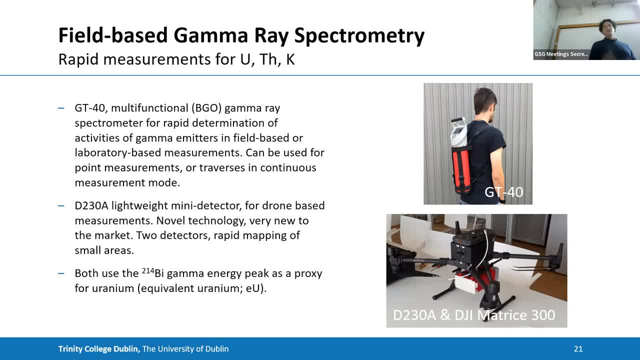 steel poles into the ground. So it's more like a rubber mallet that you might have for bricklaying. And quite often I'll have geophysical equipment with me. So the top one on the top right it's a handheld, or in this case it's in kind of a backpack gamma-ray spectrometer. 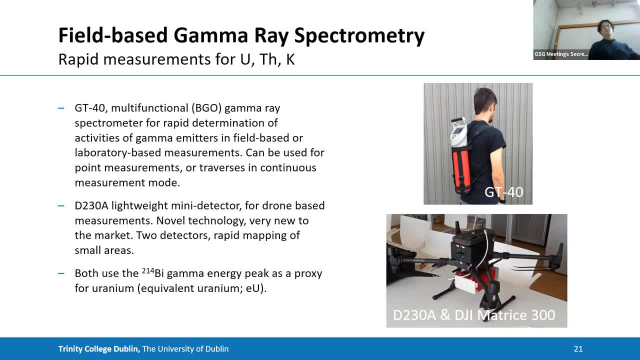 So it's very easy to use. It collects uranium, thorium, potassium data. It can be point measurements or continuous. You can do lines, You can make maps- This one on the bottom right. I commissioned this red box to be made. I think it was one of the first ones that the company made And 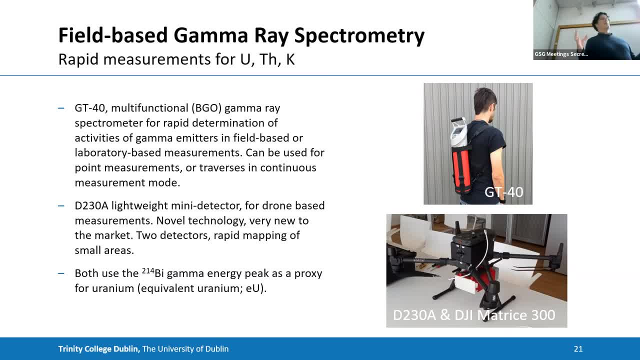 it's a miniaturized version of what would be in the helicopter or the airplane for gamma detector. It's quite heavy, though. Why does it be lightweight? Passed to a drone, It means that we can deploy the drone, We can fly at low altitude and we can collect very high 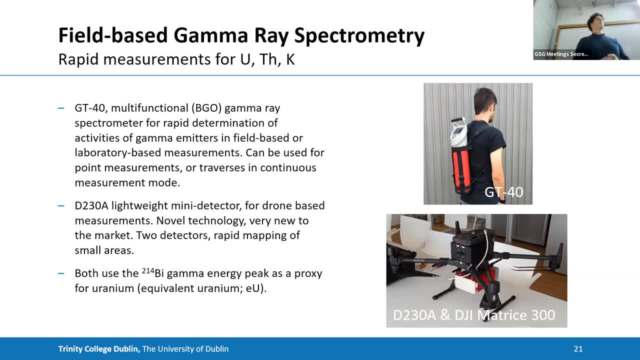 spatial resolution data very quickly. So if there's an area you want to investigate, we might identify it on the TELUS data set for the whole country. But we say, okay, we think something's going on here. We don't really have the high spatial resolution data to look at it. Let's take 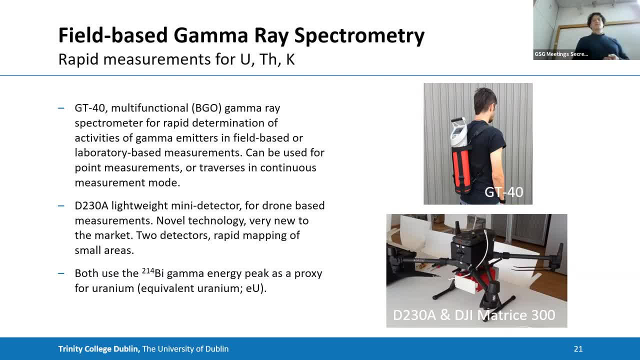 the drone out for a day, We're going to collect data and then we're going to process this And then we've got, you know, custom made high resolution data set. So it's a very novel technique. It's a lot of fun. It's not that simple, straightforward to do. A lot of problem solving. 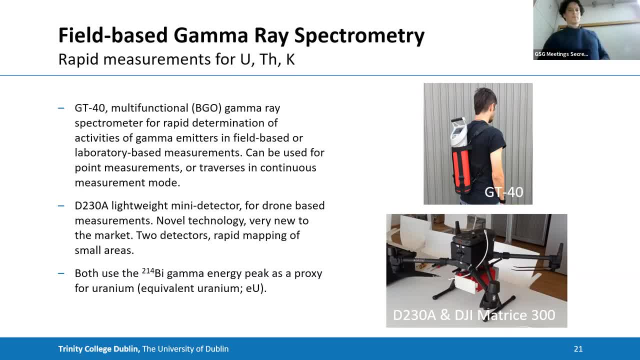 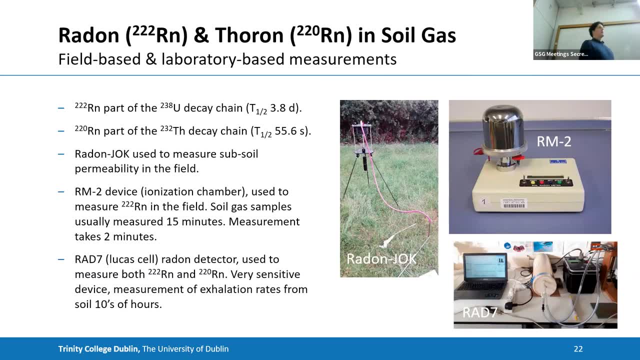 But I think a lot of promise. Well, I know a lot of promise. Other things we do: we measure soil gas. So we actually take gases from the soil, typically at a depth of around 80 centimetres to a metre, And we put them into this thing called it's an evacuated cylinder. It's a kind of 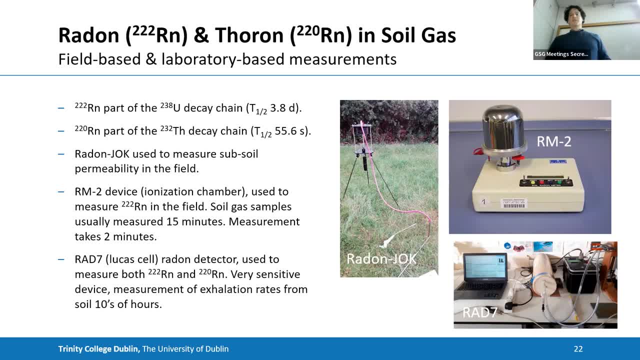 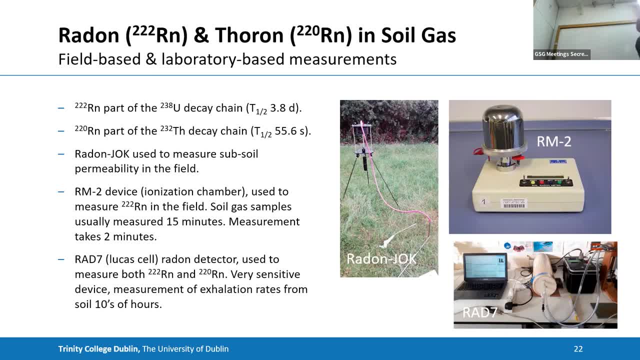 It's about this size, It's a tiny thing, And what it does is it counts the pings of energy from each alpha particle. that's been taken from the gas sample in the soil from one metre depth. It's been bled into this chamber, It's popped on the top of the ionisation chamber. It's left for two. 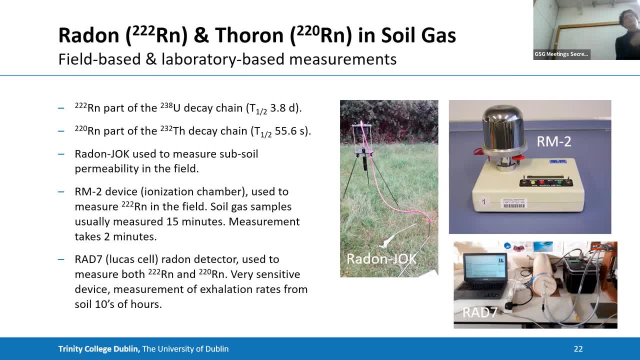 minutes And every ping of an alpha particle registers. There's an internal calibration. It counts the pings, It knows how much time it's on there for And it calculates the concentration of radon in the soil. And it calculates the concentration of radon in the soil And it 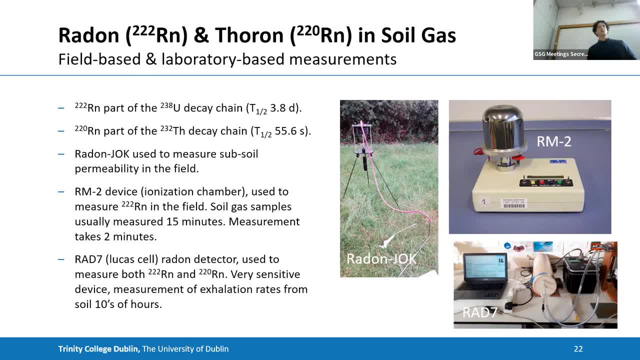 counts the pings, It knows how much time it's on there for And it calculates the concentration of radon in the soil. And it calculates the concentration of radon in the soil gas which, incidentally, is typically in kilobecquerels, or thousands of becquerels per cubic metre. 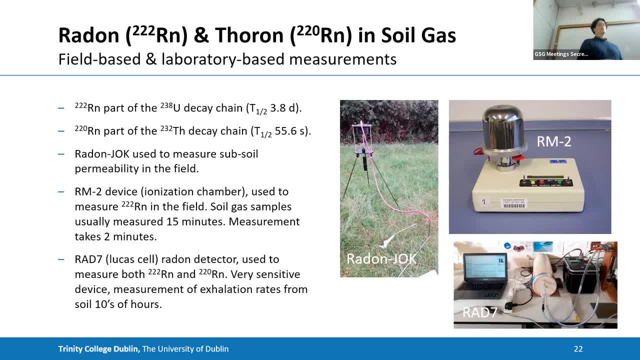 So it's a really versatile, low-cost way to measure in situ radon in the soil And it can collect a lot of data very quickly. Other kind of instruments there, I won't go into it, but they may be more suited to longer-term experiments in the lab which are 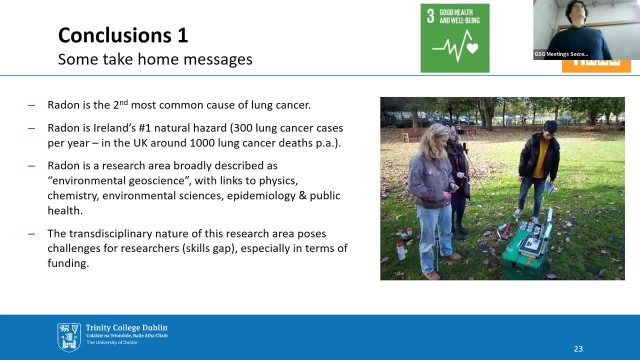 temporally resolved kinds of experiments. So I see we're now coming up to quarter to nine and I know that we have to wait a little bit. So I see we're now coming up to quarter to nine and I know that we have to wait a little bit. So I see we're now coming up to quarter to nine. 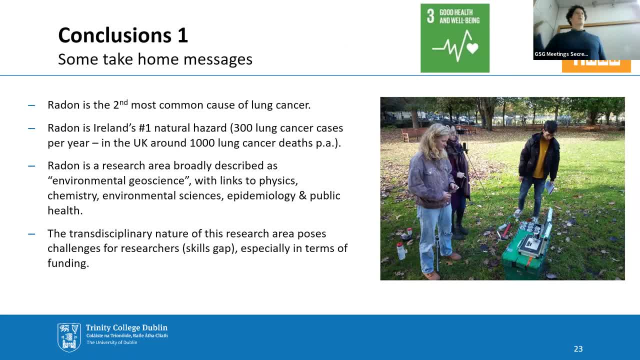 and I know that we have to vacate the room by nine o'clock. I'm keen to have some questions and answers and conversations, So I'm going to wrap up, So I'm going to finish with two conclusions, I suppose. the first one for people who have never heard of radon, which isn't you. 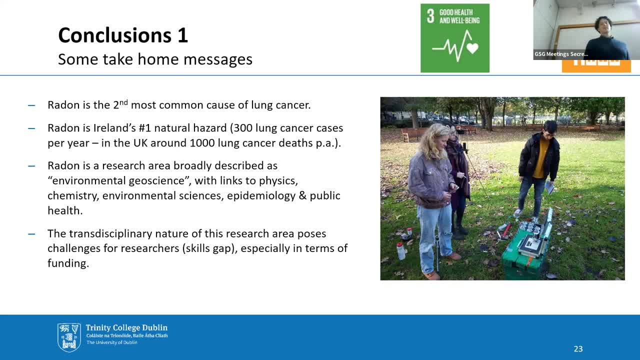 Radon. it's the second most common cause of lung cancer. It's the number one cause of lung cancer in non-smokers. In Ireland. you could classify this as the biggest natural hazard, And that's a very unusual thing to say, because generally 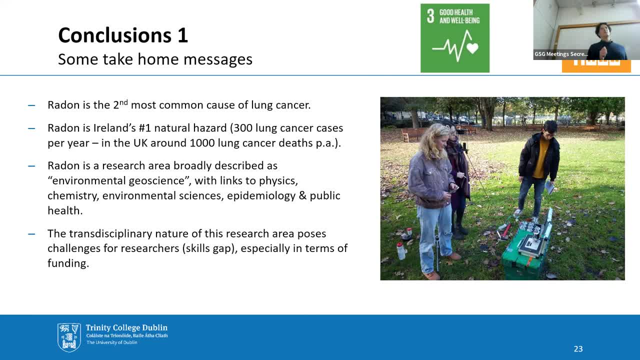 speaking, radon is not considered a natural hazard because the hazard is indoors and indoors is not natural, But it comes from the ground. It's what Earth delivers. It's very much a natural hazard. An estimated 300 lung cancer cases in Ireland per year. The UK the estimate. and it's reported differently. It's reported in terms of numbers of lung cancer deaths per year and the estimate it's around 1,000. That's a lot of people dying from something which is very preventable. So radon: I feel this is a research area. I'm very passionate about it. 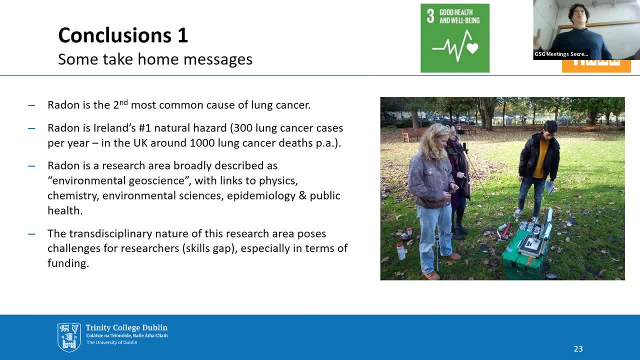 as you might have gathered, It's an area which I suppose, broadly, you could describe as environmental geoscience. It's not geology, It's not geoscience. It's not environmental science. It's somewhere in this fluffy, woolly area, somewhere in between. It has links to physics, links to chemistry. 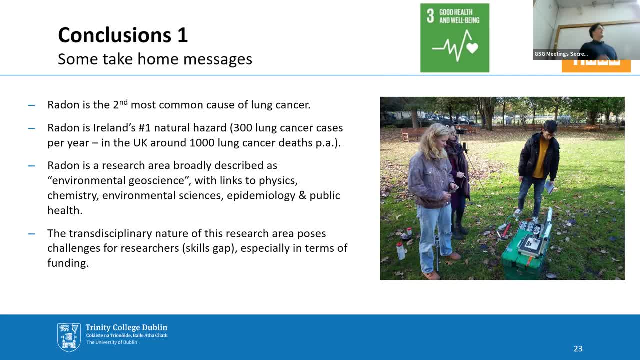 links to environmental science. It has links to physics, links to chemistry, links to environmental science, epidemiology, public health. It's very transdisciplinary in nature And I think that position where it sits is also one of its biggest challenges, because typically geologists do not. 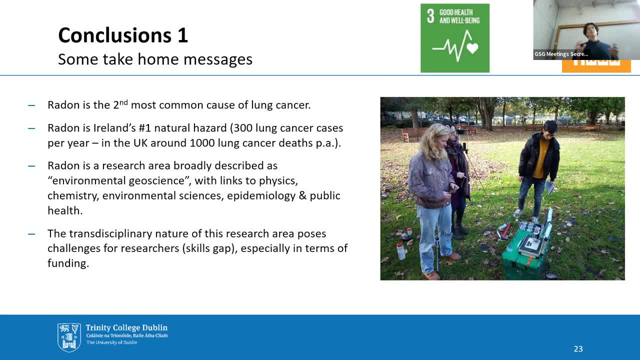 study radon. Physicists do not study radon, Chemists do not study radon. A few here and there. There are exceptions, like myself I suppose, But by and large they don't, because it somehow falls between these gaps And there are different kinds of gaps. There's this discipline-specific gap. 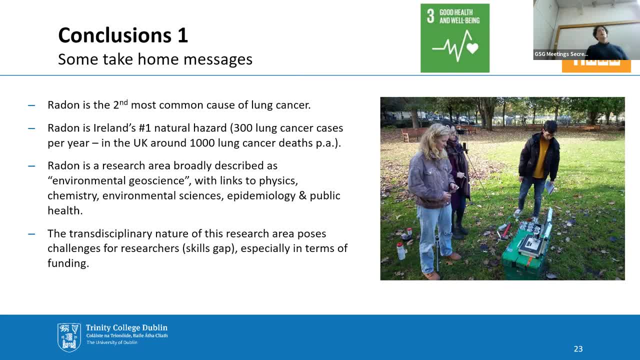 but there's also a very real skills gap. So the EPA in Ireland recently conducted a survey. They were putting out advertisements for vacancies within their radiation protection units. They were getting zero applications And it wasn't because people weren't interested, It's because nobody felt qualified. There was a very real skills gap in this area, which 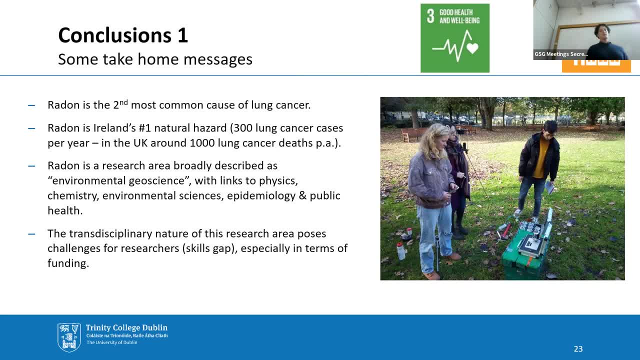 you know could include geologists and geoscientists. So I do teach at an undergraduate level, bachelor's level And a master's level. I do have PhDs and postdocs. But this is one small research group in one small 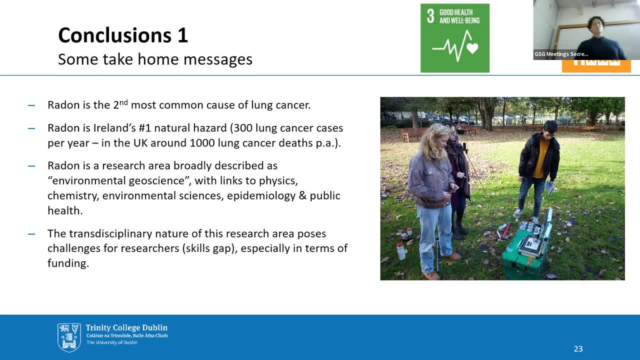 university on one small island, you know. So there's more to be done, I think, and especially in terms of funding, because different funding bodies see this as a different remit for another body. So you could apply to the Cancer Society to say, please fund my research on this. They say. 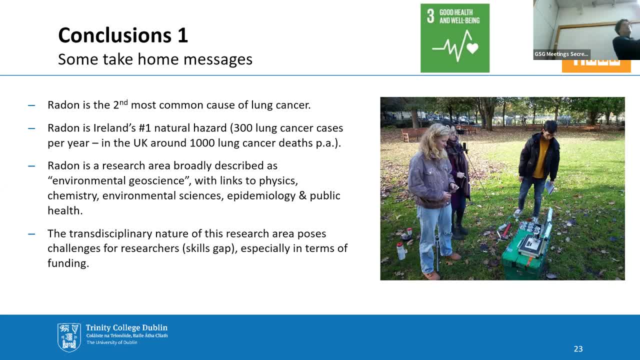 well, that's really, that's environmental science. So you go to the environmental science research body and you say, please fund this. They go: no, No, that's epidemiology, We're not going to fund that. So that's also a big, big challenge. 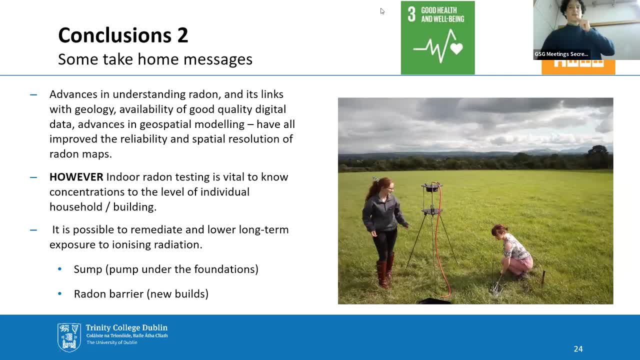 Bonus points for noting if the Sustainable Development Goals the colours. number three: good health and well-being. Number 11,: sustainable communities, cities and communities. It's the Irish flag. There's a white space in the middle. Okay, conclusion number two And I suppose a big thing for me, a big lesson in this is that 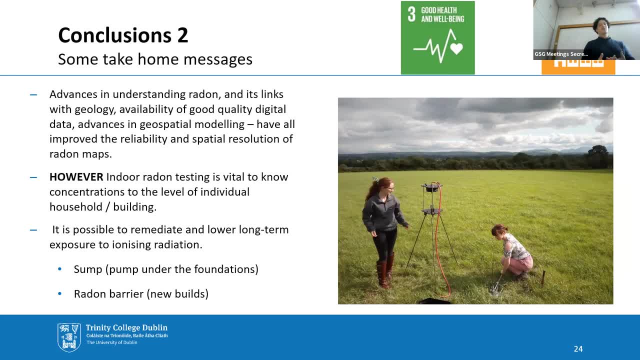 when we understand the geology, the subsurface. there are a whole lot of benefits to that, You know. this is one example. You could choose other ones, but certainly I couldn't do this research without availability of good quality digital data, And certainly there've been innovations. 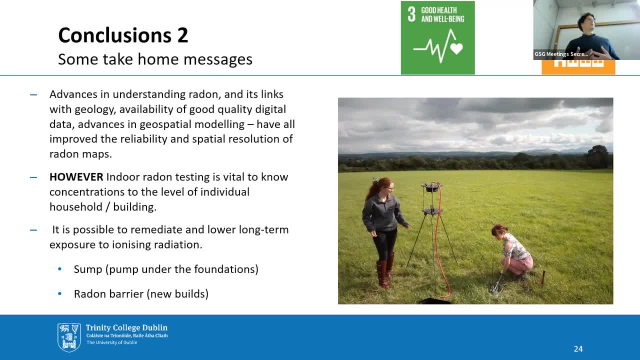 in terms of technologies and modelling and you know, computationally this is really heavy stuff. But all of this working together it has improved reliability of the maps and the spatial resolution of the maps. And if you look at the UK radar maps and if you try and get access to an older version, 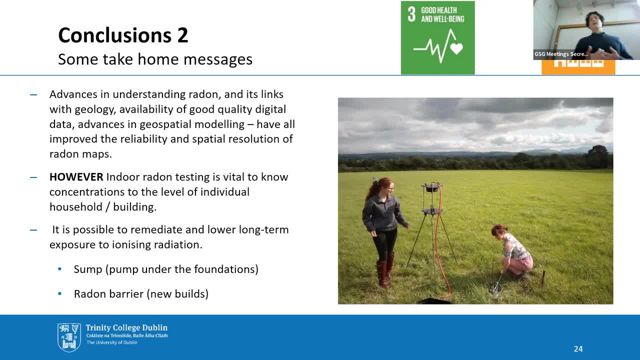 maybe you can find more archives. they are quite different. Now I haven't mentioned the UK map because I don't know exactly how it's been produced. But again, if you produce, if you put a geological map next to the new radar map, even for Scotland, you can see there are definite 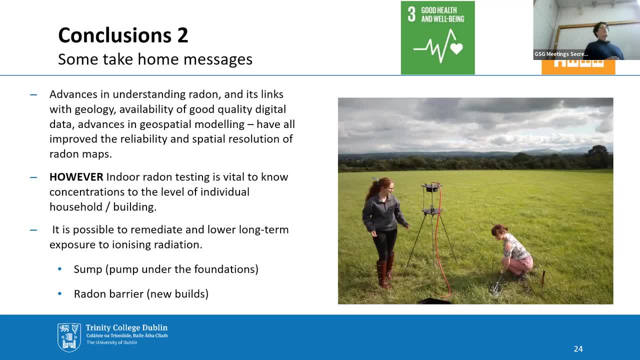 correlations with geology, and particularly granites, but not just granites. Now, as sophisticated as all of this is, that I've shown you, you know we can go measure in situ, we can do our modelling, we can integrate different data sets. There's no real substitute. 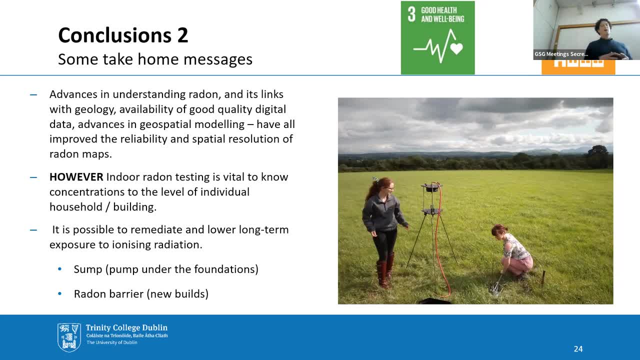 for actually measuring at home. So if you haven't measured at home, I would suggest that you do so If you find something that is high. so the levels, there's a- I think it's called a- target level, which is 100 in the UK. If it's target, that's kind of, you know, aspirational, like you know. 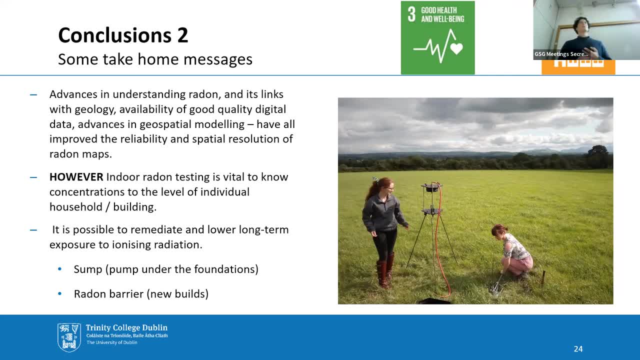 we should be at 100 or below. 200 is seen as a kind of action level. So if you measure and it's above 200, you should do something to lower it. This is for domestic residents and for workplaces it's 300.. The idea is that people spend less time at work than they do at home. I'm not sure that's. 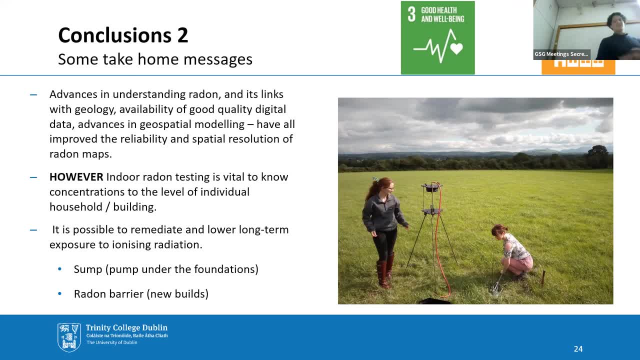 the case, But in terms of that's how the calculation is done, And so, similarly, if you're an employer and you measure in your place of work and it's over 300, then you're legally responsible to do something to lower that. So all the information you'll find on relevant websites. 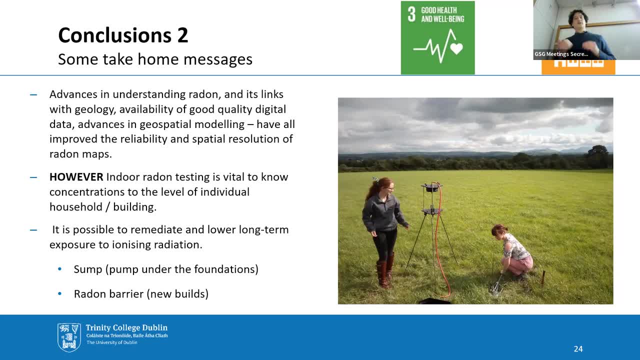 for UK radon. But in general terms, you know, if you do find radon is high you should do something about it. It's not cost prohibitive. There's something called a sump or a pump which can be inserted under the foundations. It creates negative pressure. It sucks air out of the soil. 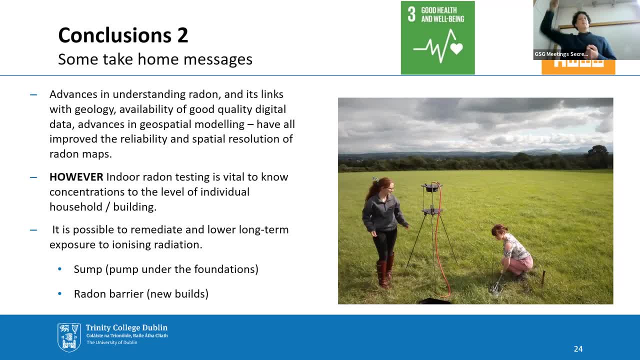 goes to an exhaust, usually at the roof level of the house, the eaves- and it stops or slows down the ingress of the radon. So if you find radon is high you should do something about it. It's not cost prohibitive. There's something called a sump or a pump which can be inserted under the 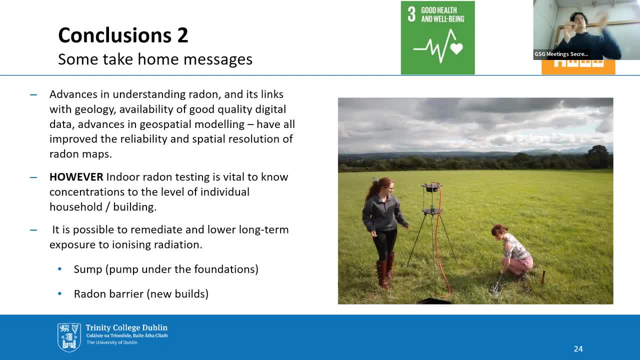 foundations. It's not cost prohibitive. There's something called a sump or a pump which can seep through cracks around pipes and things like this. If it's a new build that you're building, even if it's an extension, it's a good idea to put a radon barrier in. It's not hugely expensive. People put 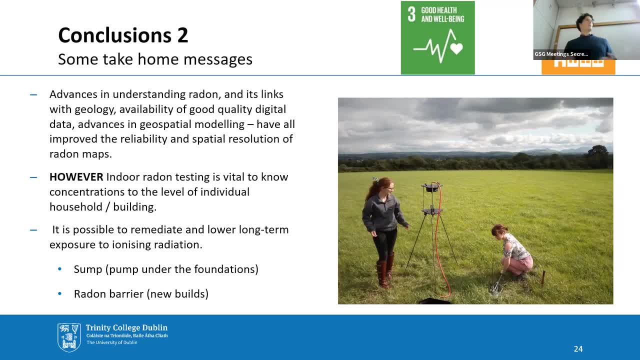 in moisture barriers. Why not put in a radon barrier Again? it's a good preventative measure, So it's easy to ignore, but don't ignore it because it can make a real difference. So I'm going to finish there. I'm just going to say, if you have been interested in what you've heard, 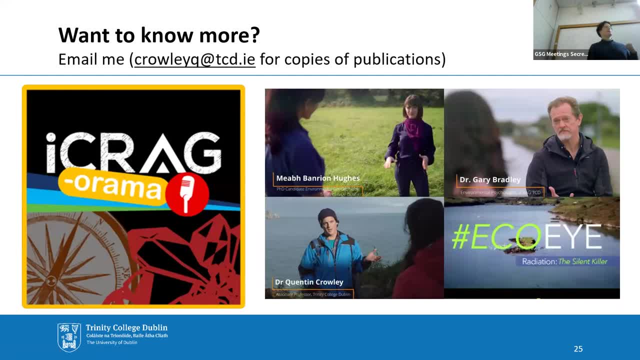 this evening and you want to know more, you can email me. My email address is here. If you'd like to read scientific publications, I can send you PDFs of these by email or I can post them out to you if you don't have email. ICRAC, it's a government-funded research center in applied 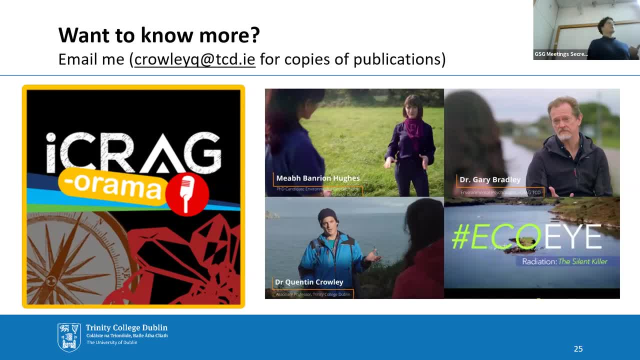 geosciences in Ireland. I did a podcast with them last year. You can go onto their podcast. it's called iCrigorama. You can listen to that. There are actually two of us. One person is talking about geothermal energy and I'm talking about radon- EcoEye. it's a documentary series. 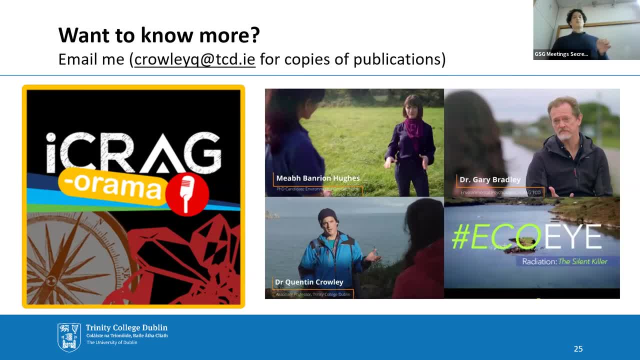 on Irish TV. You can find it on YouTube. So if you just Google YouTube or you go to YouTube and you search for EcoEye radon, you'll find it. So I'm part of that, And these two- Gary Bradley is on the right, who's actually a psychologist- was part of my research group at the time. Gary Bradley is on the right. who's actually a psychologist was part of my research group at the time. Gary Bradley is on the right. who's actually a psychologist? was part of my research group at the time And Gary was studying. 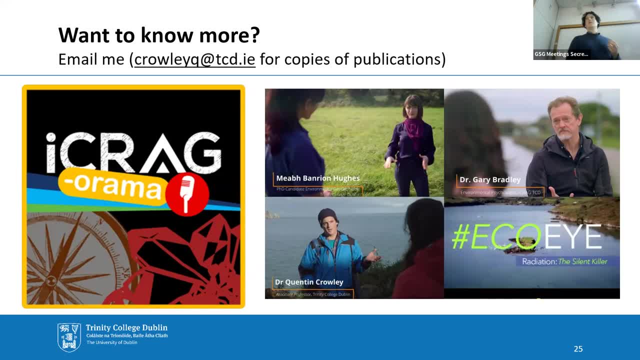 people's risk perception of radon and how it affects their decision-making about whether or not to test and, if they find high, whether or not they remediate, And there's a huge factor in people's perception of this as a risk. The bottom line is it's much easier to ignore than to do. 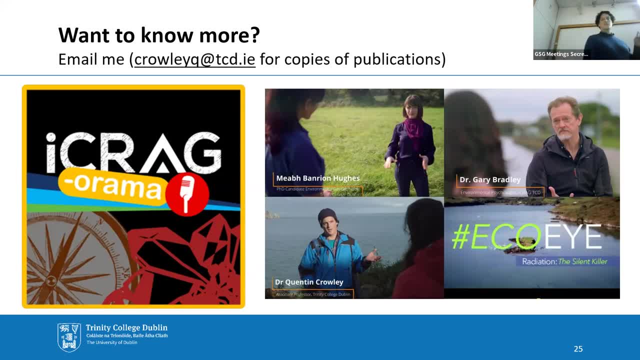 something about it, And Maeve Hughes, who actually has her PhD defense next week- hopefully she recovers from COVID, which she has at the moment. Maeve did her field area in Southwest Ireland in an area called Castle Island, where there was a house that was measured to have 1,600 becquerels per 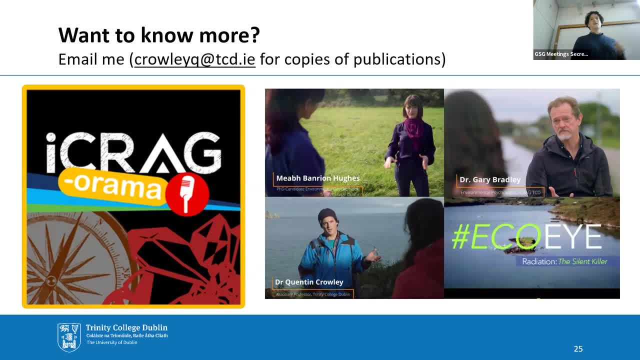 cubic meter, really off the scale high. Yet there was very poor understanding of why it was there. So she was looking at this from a geological perspective: mapping the soil, gas radon, taking soil geochemistry, doing geophysical measurements, And we now have a much. 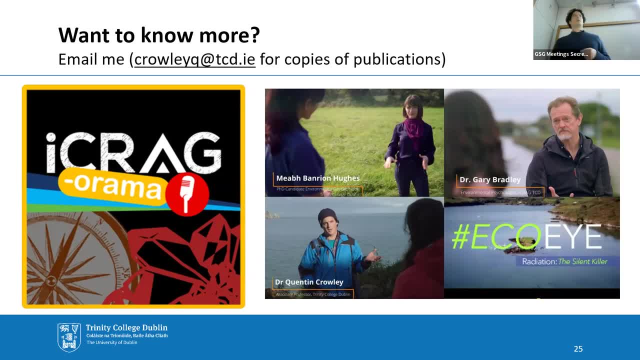 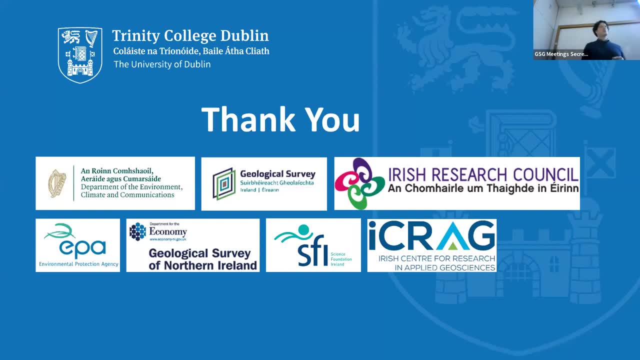 much better understanding about why anomalies like that Castle Island anomaly exist. So thank you all for your attention and thank you to the various bodies who have funded my research over the last few years. Hope you've enjoyed the talk and I look forward to questions. 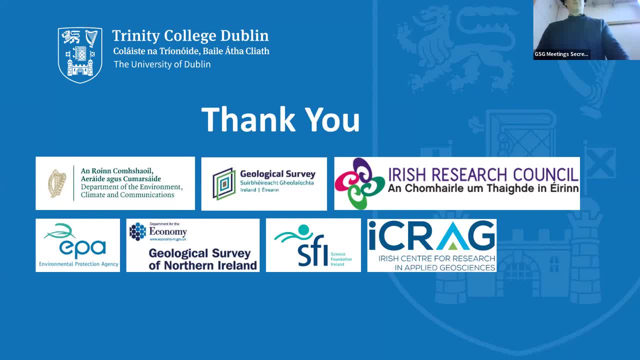 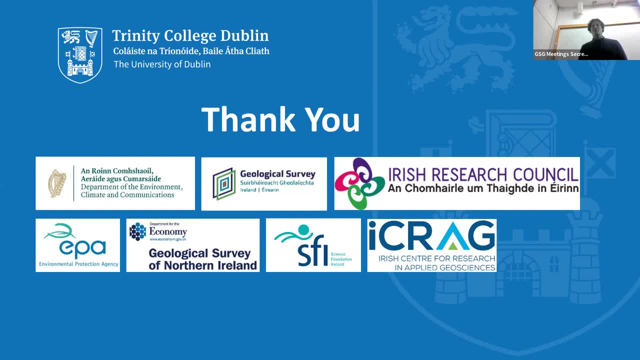 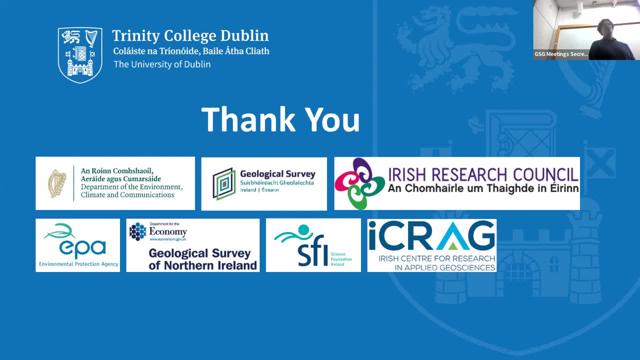 It was used in the 1980s to make cheap glasses as replacement for glasses, you know, for the lens that were ground down. And then some physicists realized that it actually reacts to alpha particles. Every time there's an alpha particle, It's disintegration. 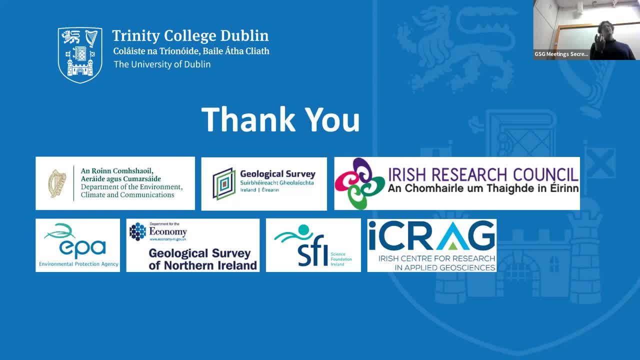 It leaves a small track. So there's a thing called track density, basically, and the higher the concentration. usually they're left for at least three months in a room and this radiation damage accrues on the surface of the polymer. And then they're etched in sodium hydroxide and then they're point counted and there's 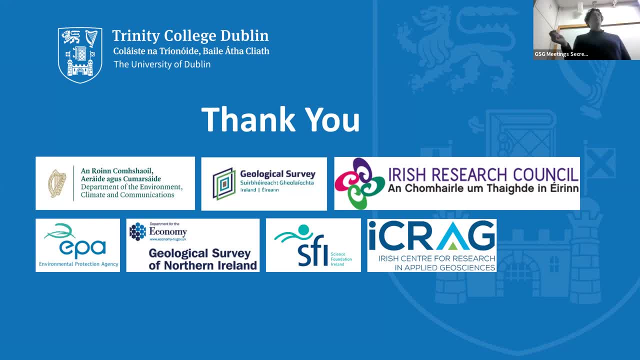 a direct correlation between the track density and the concentration of radon in the room. So the thing is Very good. I have a couple of questions I didn't ask. Okay, Go for it. Second, which is completely different, Go for it. 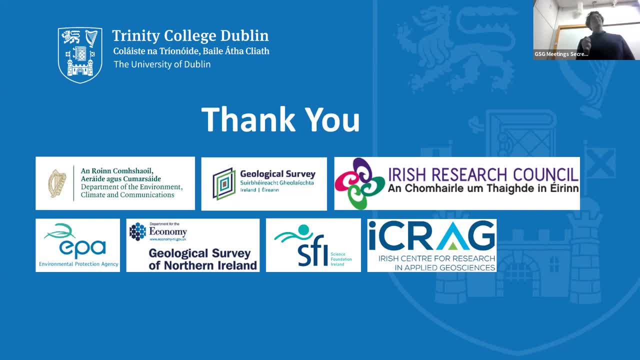 You said on a couple of occasions that there's no way to identify on the individual that all the blood cancers are deep in radon- No, In non-smokers. But are you aware of any work on rotational profiles and rotational signatures in tumors? 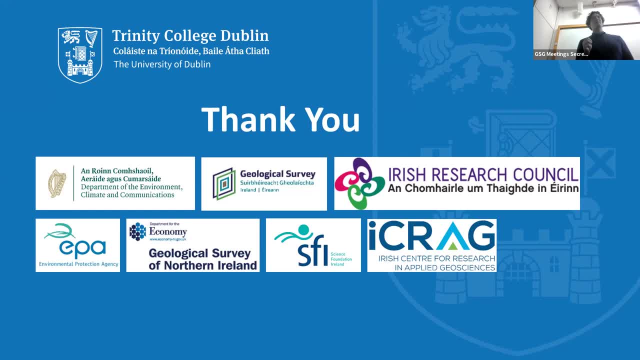 Yes and no. So there has been. It's a friendly thing. Yes, Okay, I'm not a cancer expert or a lung cancer expert, So what I understand is there are four subtypes of lung cancer, and it's not understood if particular subtypes are related to radon, let's say, and another to tobacco. 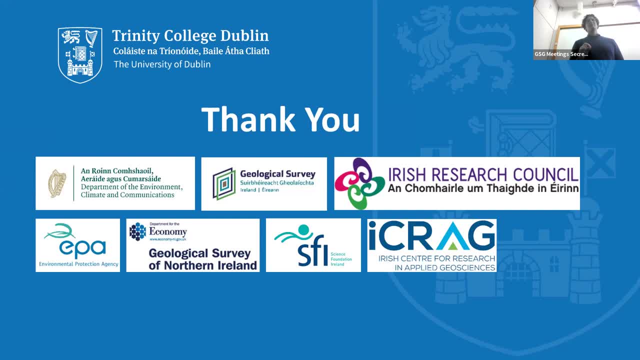 It's not known. Increasingly, it's becoming apparent that even within the histological subtypes of tumors, they may have different mutation profiles. Yes, It's not known. It's not known. Okay, That's an interesting question, And actually I'm working with researchers in Queen's University Belfast on that exact. 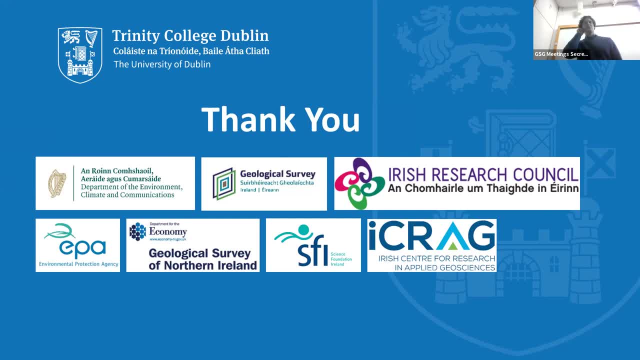 question And they've just advertised a PhD studentship and one of the areas is to investigate this, But we don't know. It's a simple answer. Okay, Quick question. Thank you, Yeah, Quick question. I live in a town in Glasgow. 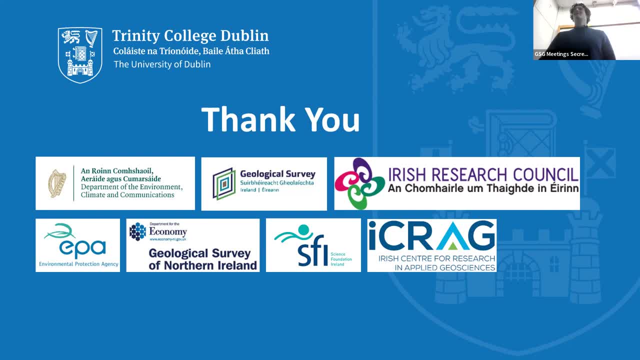 Mm-hmm, I noticed What floor are you on. I'm on the second floor. Okay, It's made of triacetic sandstone. Yes, It's the corner. then It's the corner. Where does it come from? 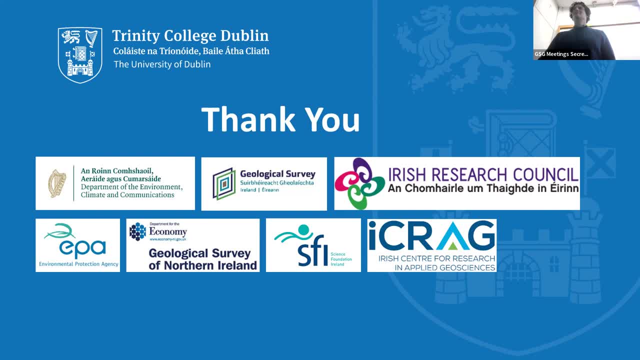 It's in Kowloon And I noticed I've also done some work myself in this department. Mm-hmm, Yes, Triacetic sandstone, It's down in Devon, Okay Measuring. But what comes to my mind now is when I got to Aberdeen. 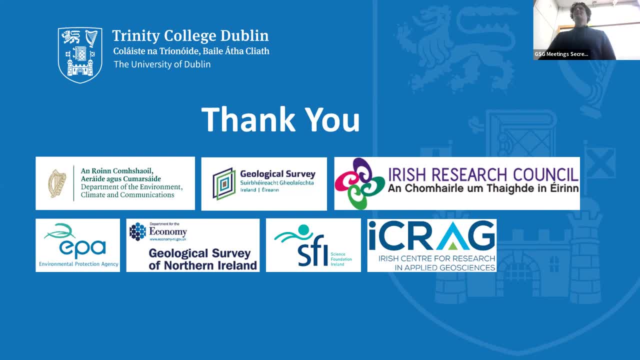 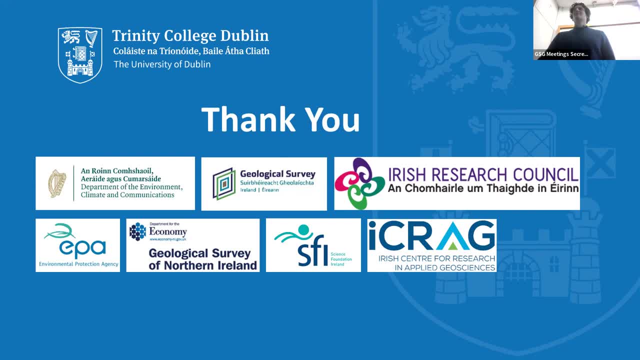 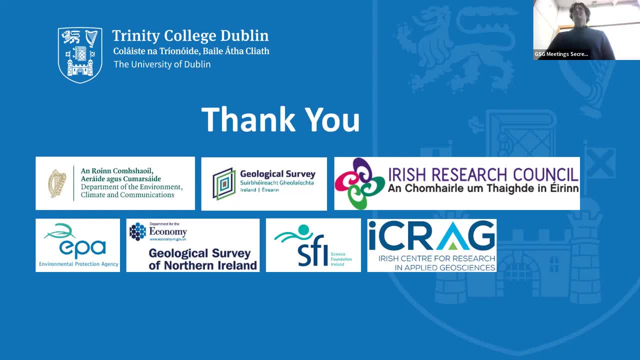 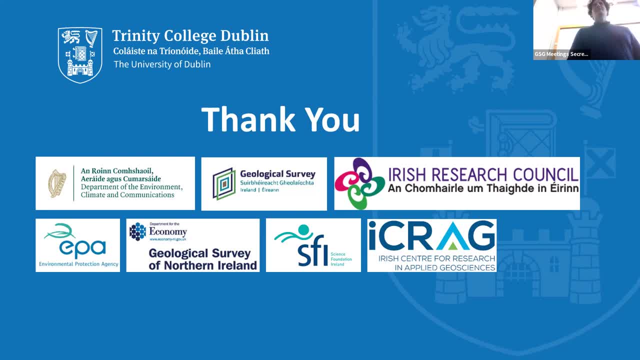 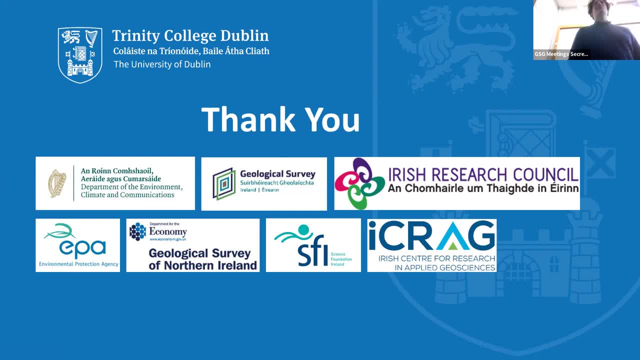 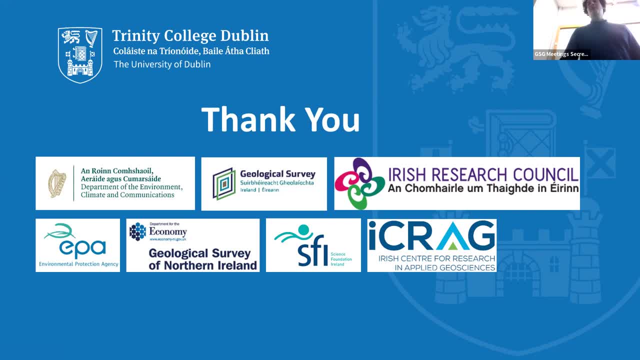 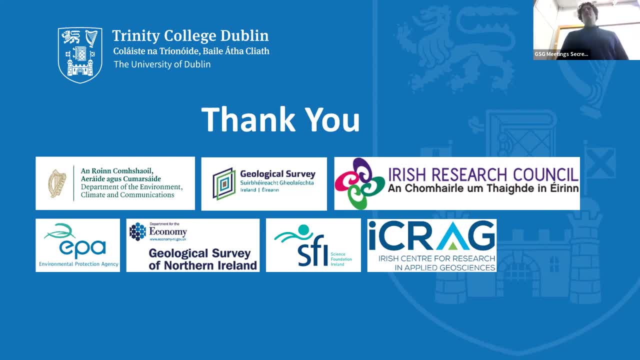 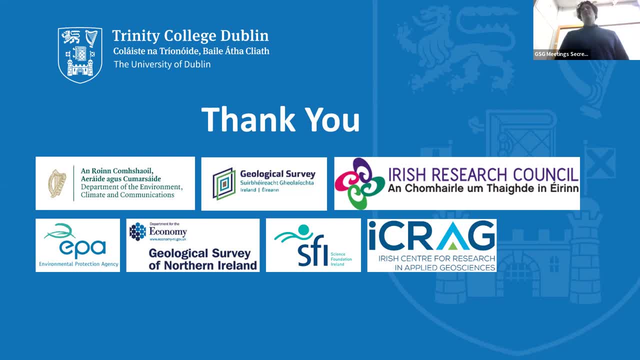 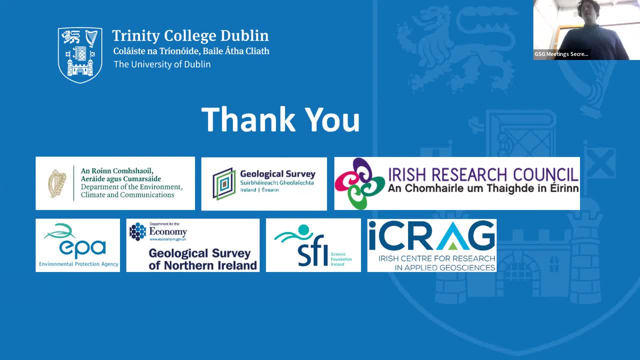 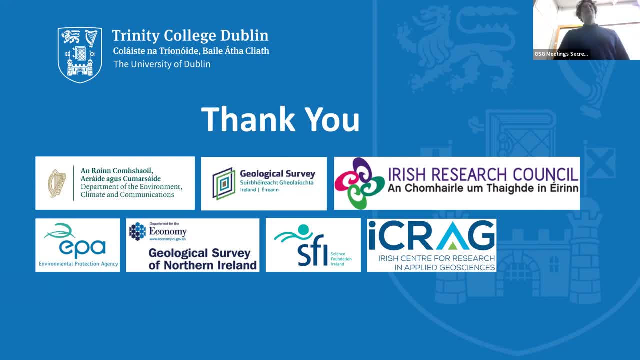 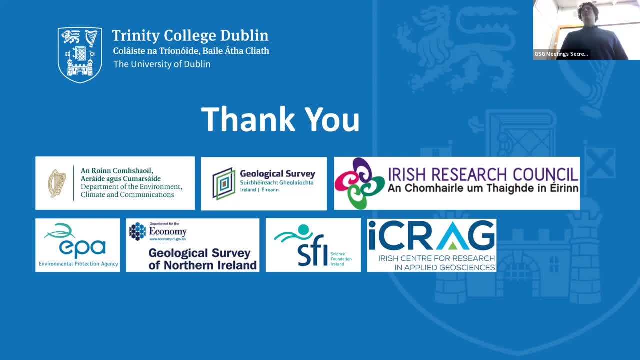 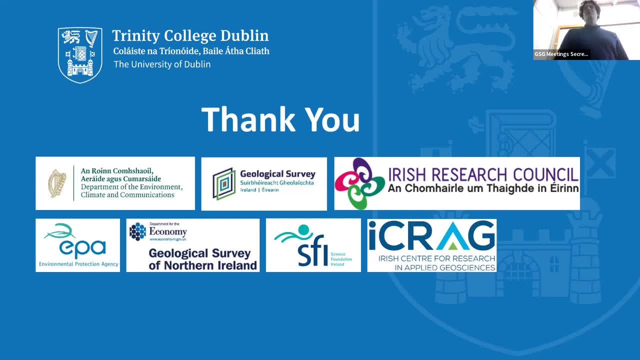 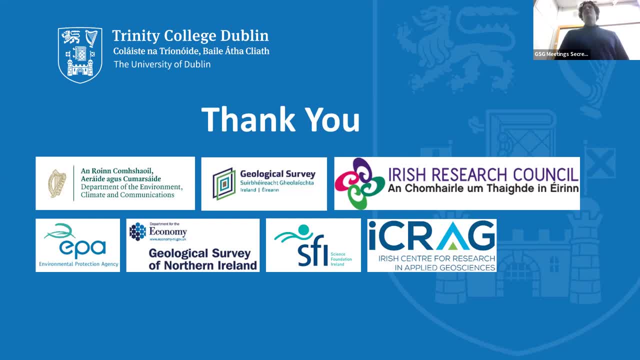 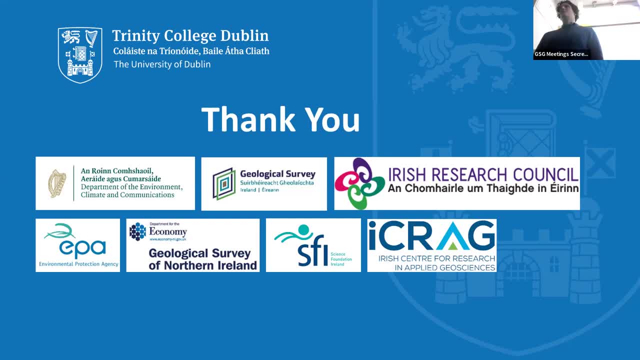 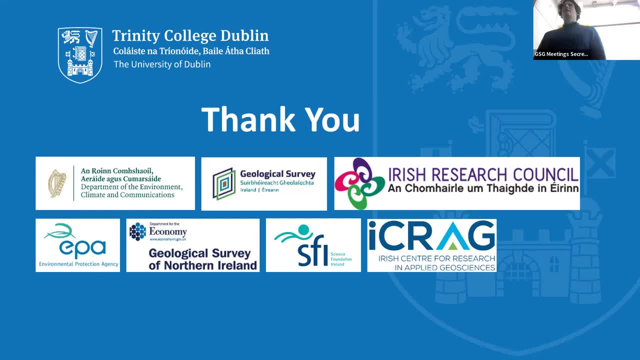 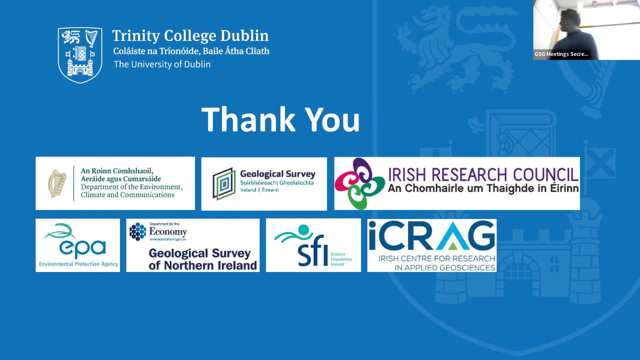 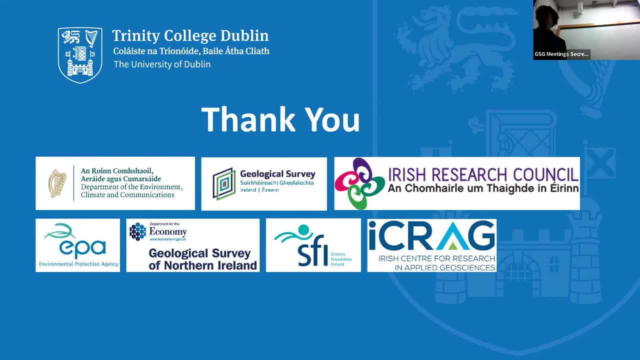 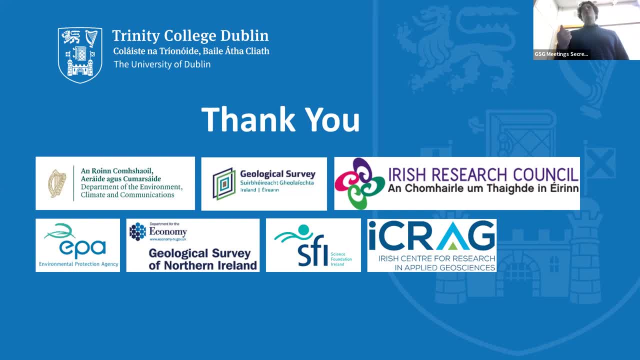 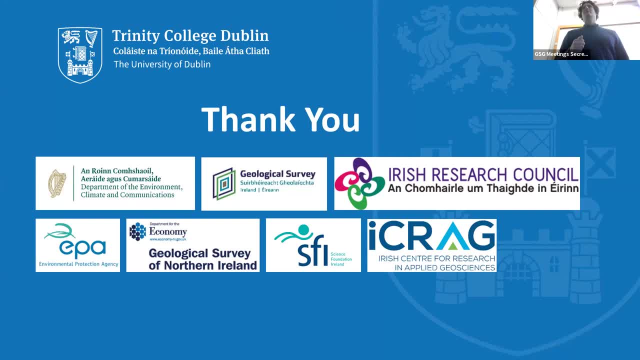 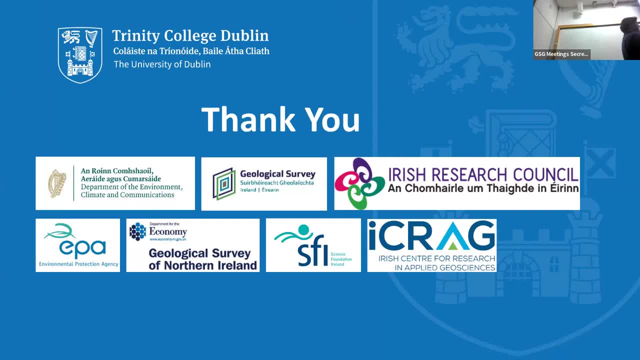 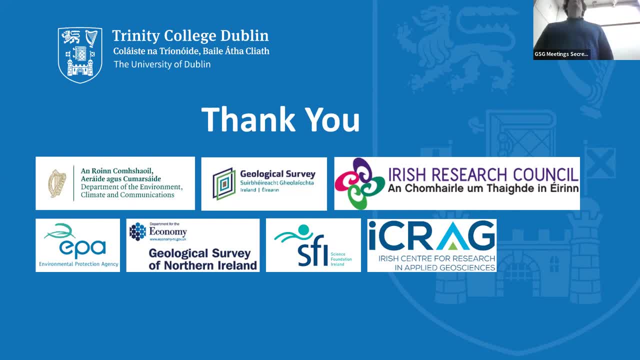 You mentioned that we take a look in public at the rates we have. We also mentioned on that the bedclothes density in the soil is much higher. Is that a review and is that something to do with it? No, it's because the soil, the radon and soil gas is much higher concentration. Once it escapes to the atmosphere it's essentially diluted, So you're getting like a small point source which is diffusing into the atmosphere. So typically you might have like four becquerels per cubic meter of radon concentration in open air over land be much, much lower over. 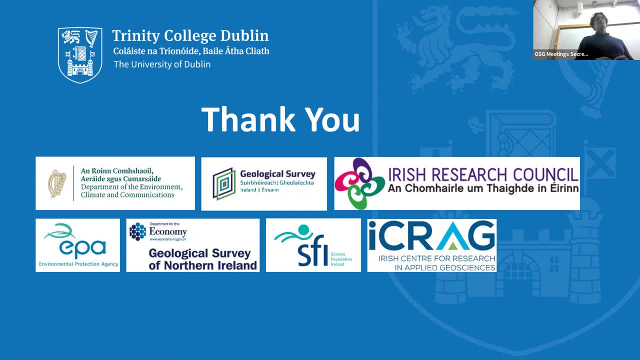 sea because there's very low concentrations in seawater But then in in soil concentrations it's typically kilo becquerels like thousands of becquerels. Yeah, Related to that in terms of protection for us, obviously, if you put a layer down. 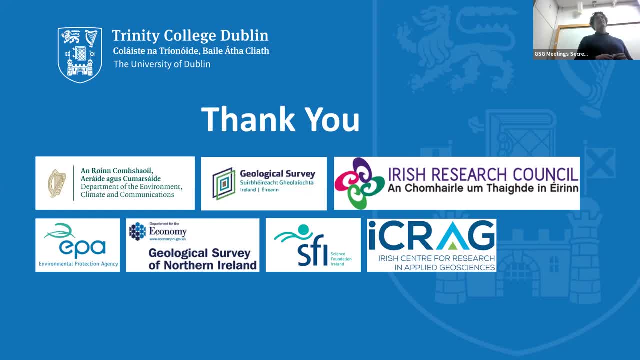 Yes, And presumably some of the things we checked on the back end would say: if you have to test one, you're just going to need to put a layer down on the first one. Yes, It's cheaper, But presumably if you put a fan in your earwax. 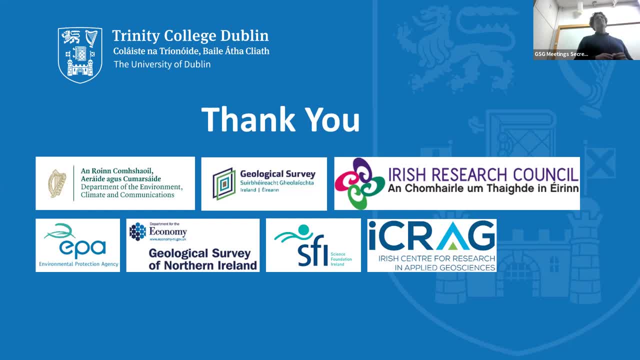 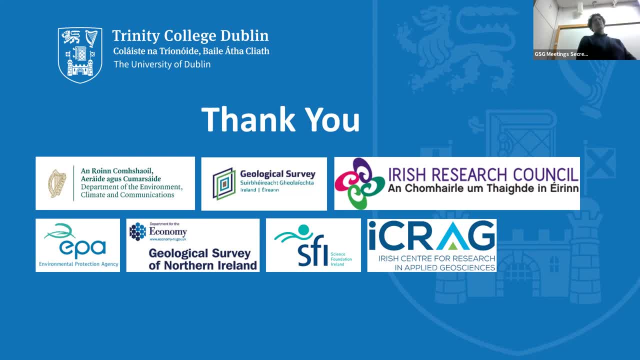 the floor and the ground level. essentially Yeah, So anything which increases ventilation is a good thing. There are some incidents of the opposite happening, particularly in retrofitting of old buildings. I mentioned Castle Island and the really high values. That was a perfect storm. 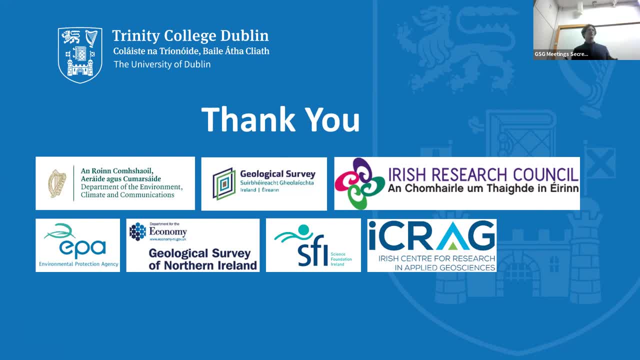 in that there was an old cottage, I don't know from when, could be 1700s, 1800s. It didn't have a solid foundation, It was compacted earth. Family had lived there for generations. They emigrated. 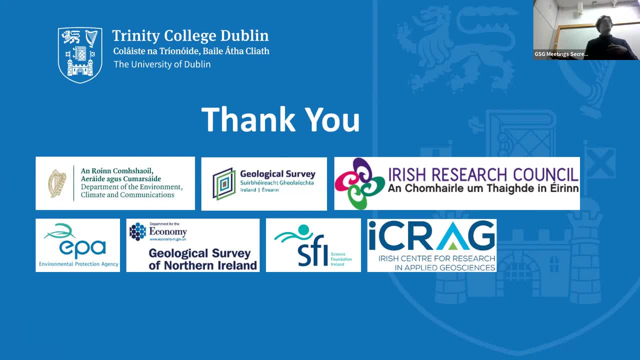 they went to the States And maybe two generations later some people came back. They renovated the house. They put an extension on. They put double glazing in. The new parts of the house had foundations. They put in central heating. Ventilation was really poor, The soil 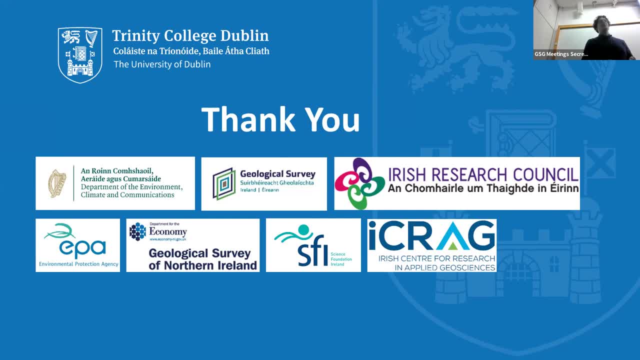 gas radon concentration almost broke my radon detector. It went off the scale. You couldn't measure it, It was so high. So that was a good thing. That was a perfect storm. It's an example that retrofitting where ventilation is poor can be a 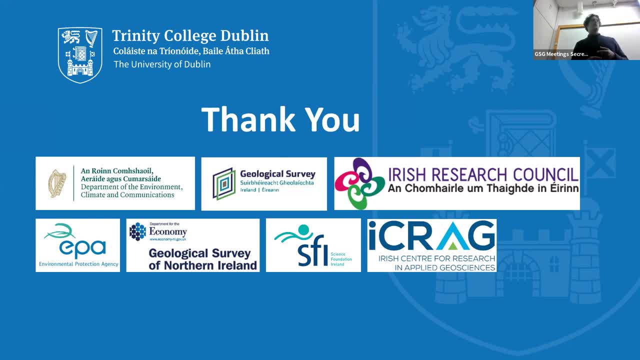 really bad thing. It doesn't mean that all retrofitting will lead to high indoor radon, but it can happen And it's something to be aware of. You never want to decrease the ventilation. Yeah, exactly, It was a convection cell, basically. 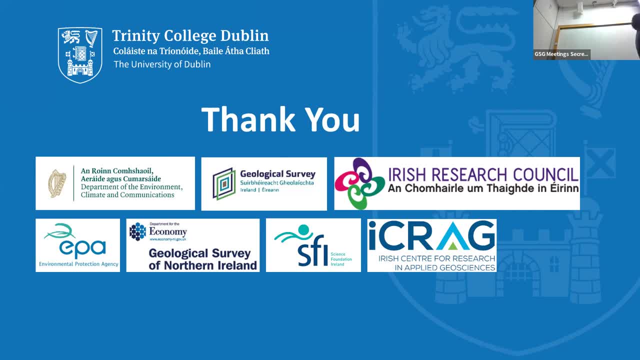 You've been very patient. You had your hands up first. I know, Yeah, Yeah, I know I'm asking you now. I started a lot of works in Sweden. I bought a house last spring about an hour west of Stockholm And it was, of course, visiting. And he said: 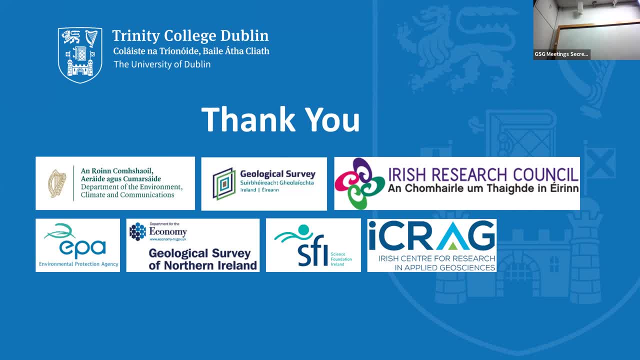 part of the process. they're strongly encouraged there. but I don't think it's not legal to do a radon test on the property. And he was saying he thought I presume it's a private business over there quite costly, and he's wondering And I now realize the total. 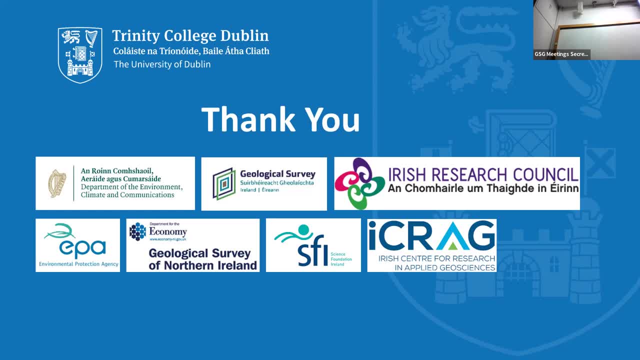 egg dumps. I'm drilling down at the geological map mark of Sweden to see what his house is sitting on, which I did. It's not sitting on a granite. it's sitting on either a schist or an ice, I don't remember. I said it's unlikely to be a problem. 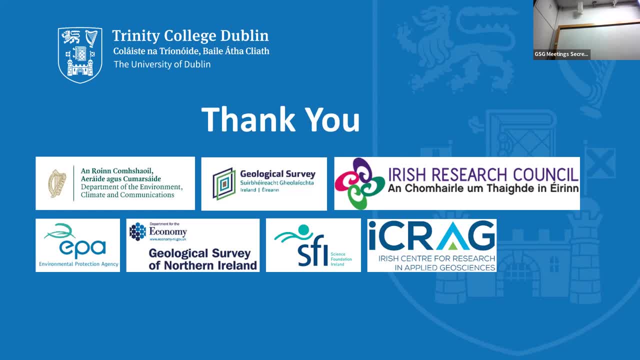 and he's not had the test done yet. Am I killing him? You should get the test done. You should get the test done, Always get the test done. The second question, which is: how much does the test? how do we do the test in the UK and what? 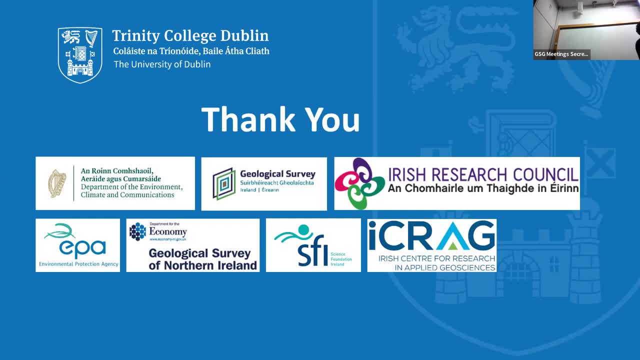 would it cost? What's the cost of Sweden worth? The only way to know for sure is to measure So, and it could be a confluence of different factors. Something I didn't mention, though, was occupancy style and build characteristics, So it could be that the geology, the geogenic factors, 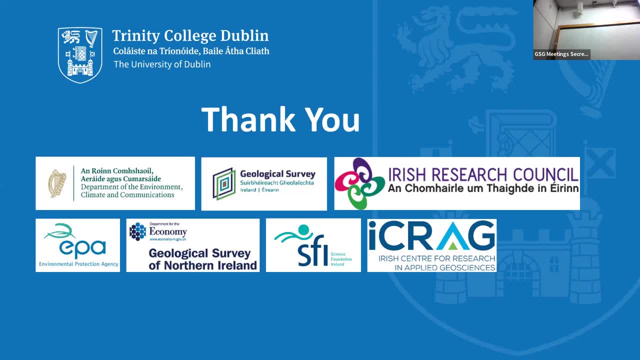 could be responsible for something like 40% of the variability of the spatial variability of the radon, which means 60% is coming from the same thing. else It changes from area to area. but the type of building, how it's ventilated, how it's occupied, you know all the windows. 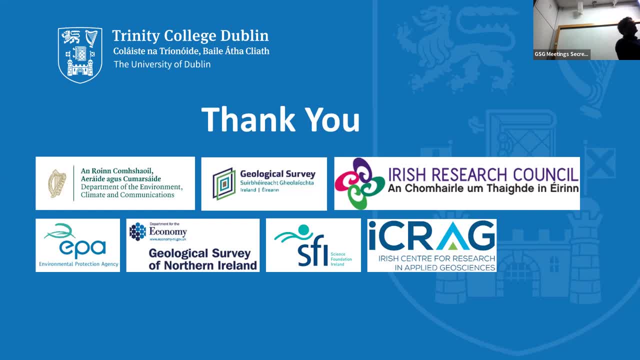 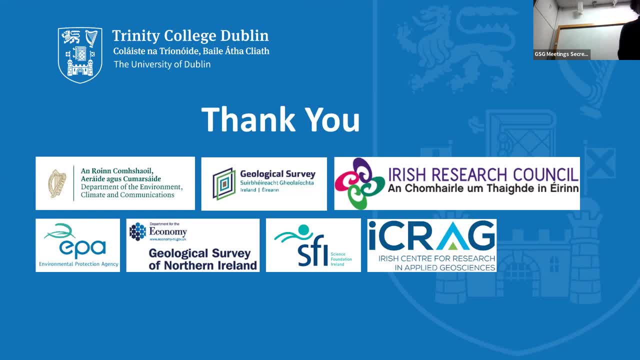 It's good to get on the ground, pitch right. I mean that's just the cost of the UK, but if you go to, I always want to say health protection. I mean that's just the cost of the UK, but if you go to, I always want to say health protection. 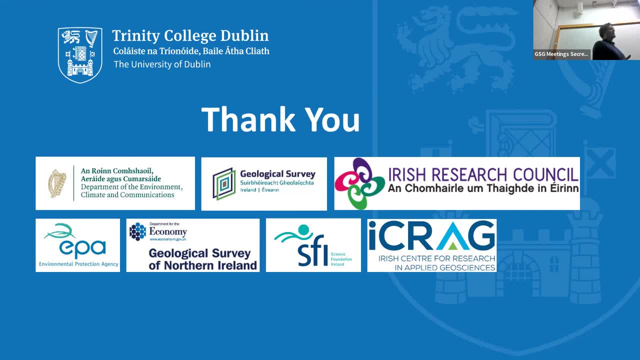 whatever it's called now. you can find information about ordering tests. I know from Ireland. the cost is typically like 40 or 50 euro and they send out two of these little detectors. they're single-use things. There's a very interesting Norwegian firm- I don't work. 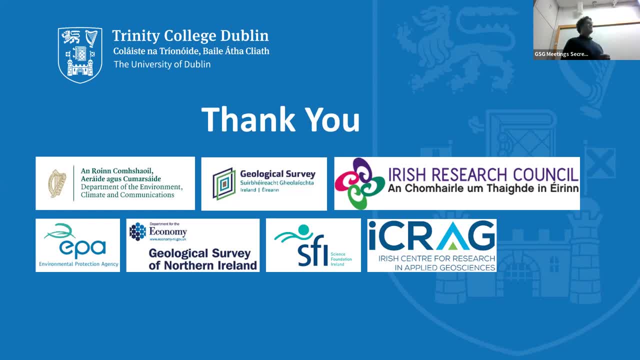 for them. I don't have shares in the company. I did buy one of their detectors because it's a thing with a battery: you can hang it on the wall and it measures continuously. So the thing with these small, solid detectors is there's no spatial variability. 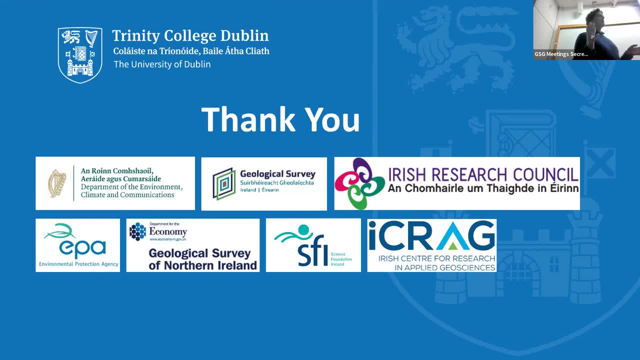 it gives you the average concentration for that period of measurement, which is usually three months, and then it's averaged and it's upscaled to one year. it's like a conversion factor, But for these digital monitors they give you a real-time thing, real-time reading. and you can see if the temperature is changing outdoors, like day and night now you see a change in the concentration indoors- And if there is a weather front coming through and the air pressure is changing. if it's a high air pressure, it's a combining pressure which tries to keep the gases. 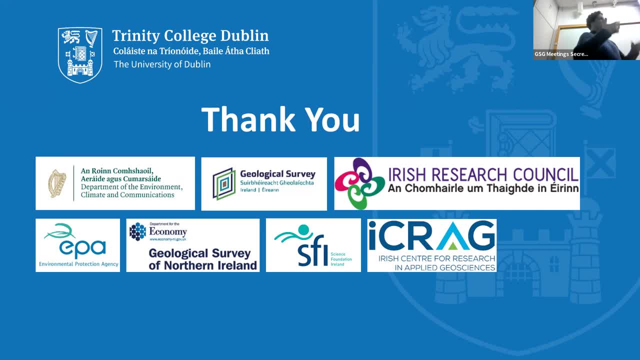 in the soil. If it's a low pressure, they're actually being sucked out, So you can also see oscillations over different timescales. It could be that somebody opens the window and suddenly the pressure changes in the house and then the concentrations change. So they're very useful. 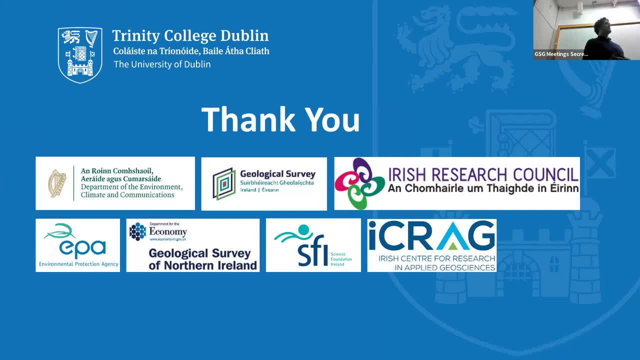 things, but then they're talking about a few hundred pounds, but you can use them for years and years and years. Thank you very much. Great talk, really important. Thank you. Okay, I think we have to draw to a close. 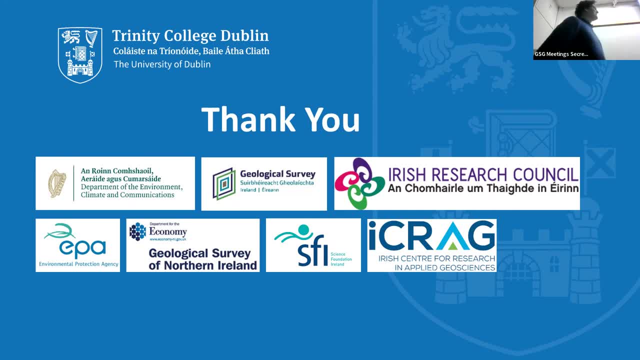 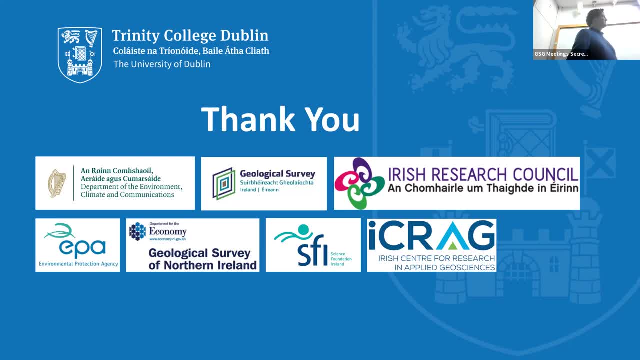 Okay, So the meeting secretary's email address: Just send them back and send them to me, and then I can send them back. Yeah, Yeah, because we often don't get any bookkeeping what you provide in there. Yes, Ian has a PDF of my slide deck. 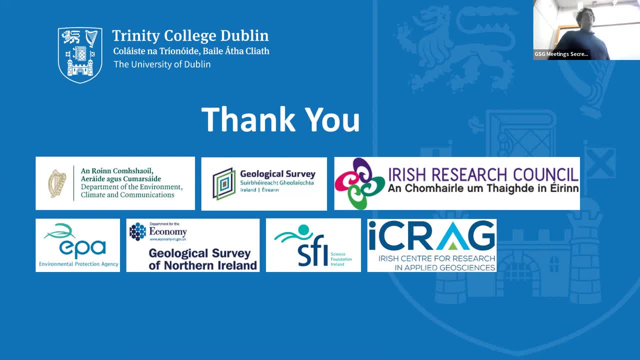 Yes, Ian has a PDF of my slide deck, So anybody who wants a copy, you can email them in a second too. Yes, Ian has a PDF of my slide deck, So anybody who wants a copy, you can email them in a second too. 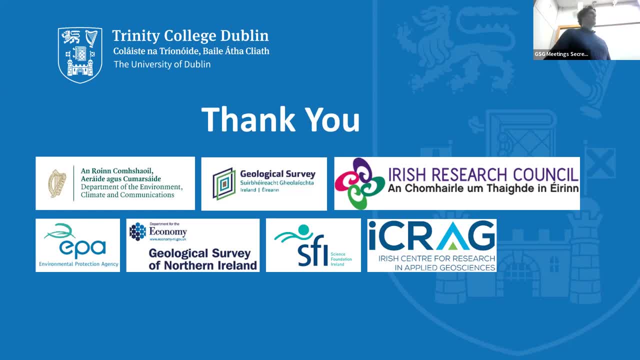 I think it's something like two megabytes. It's not too huge. I used to be one of those people in the Fetal C area, So I've now gone to working on nothing but color box and and stuff like that, And so somebody else was saying: the plan It, This is a lot. It's really nice to see that convergence there. So I was given the job of TPGIS and things like that. It's really nice to see that convergence there. So I was given the job of TPGIS and things like that. I'm really grateful to that. I think that's really important. I am grateful to all the staff and I think it's a big job. Thank you. 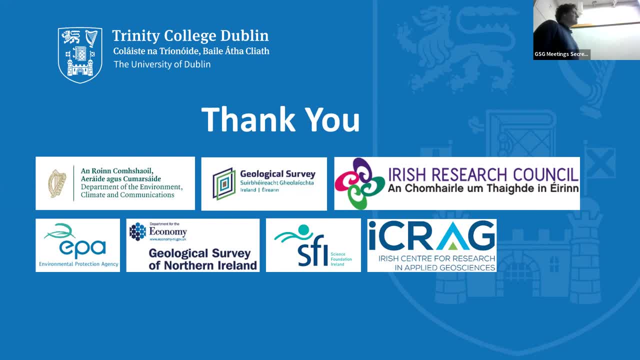 I had to cook up an exercise really quickly and the only really map I had that I could do the exercise on that I had to do the next morning was Cleveland and the hills around there. So I cooked up an exercise which had various layers and spatial analysis. I was delighted to see the 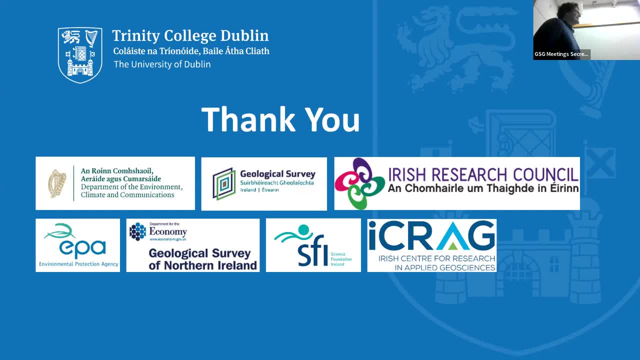 approach you used is almost exactly the same, except I've got faults in it, but they're all fictitious faults which are always permeable. so there we go. real world faults. so there you go. There's a kind of hidden feature is the effort that you have to put into the spatial analysis. 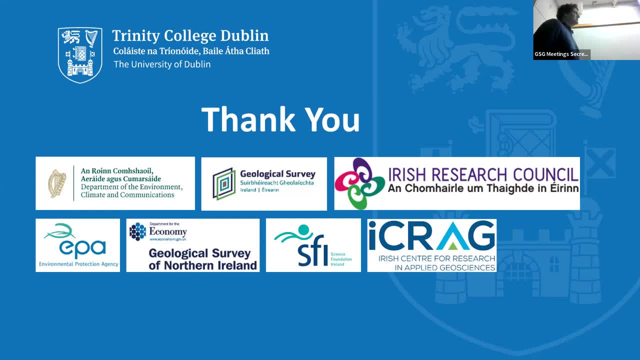 and it's a whole other story, and the power of that kind of application is amazing really to be able to do that. and so you know we've had a really nice presentation this evening, with actually quite a lot of complicated things distilled down to a level where we can all 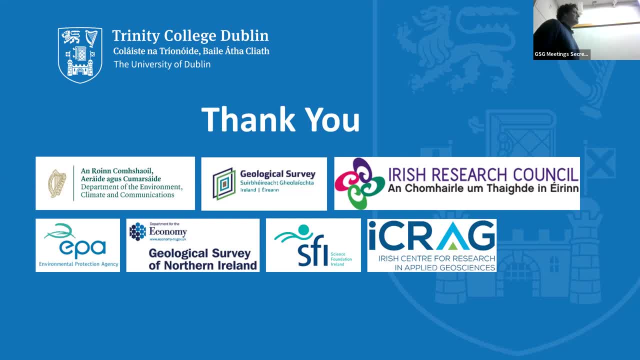 sort of get access to it. Very nicely, you've explained things beautifully and very clearly. I think that's been great, and we've just seen the way in which something's so human and so important to us all actually maps out and looks like geology and the geology there is the thing that's. 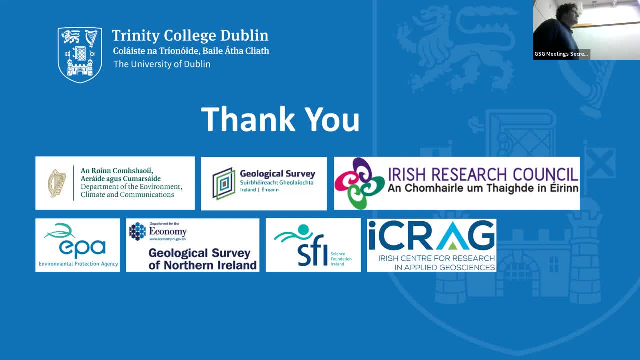 influencing people. so it's nice to have that connection between you know the real world lives of people and their health and the geology that we're also familiar with from a lot of the other talks that we have. So thank you so much. My pleasure For coming along this evening, I think. 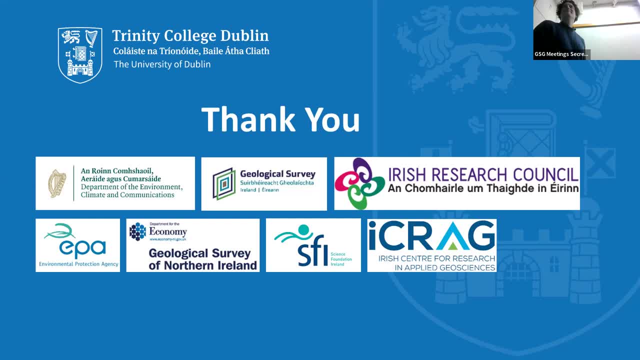 I'd like to thank you in the usual way that we've been talking about today. Sorry, we're not going to have the clap-o-meter or anything like that. Thank you, Unless you quit at the start. You're right. It's so good to know you. 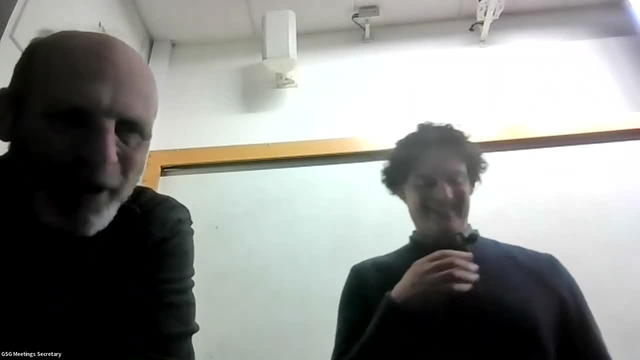